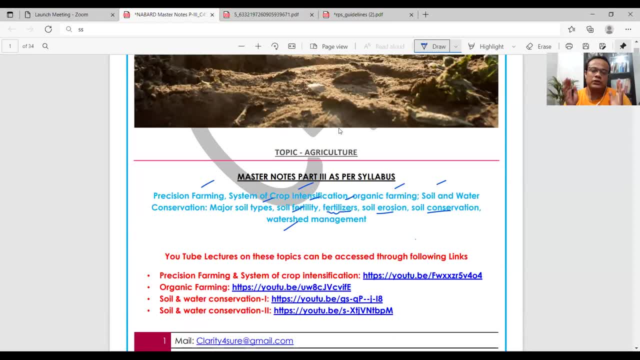 We will be discussing one by one, and I will be stressing upon those areas only where the question comes, because there are so many things to read upon. It is not time that we will discuss each and every topic in minutely. That is not the purpose. The purpose is to highlight: 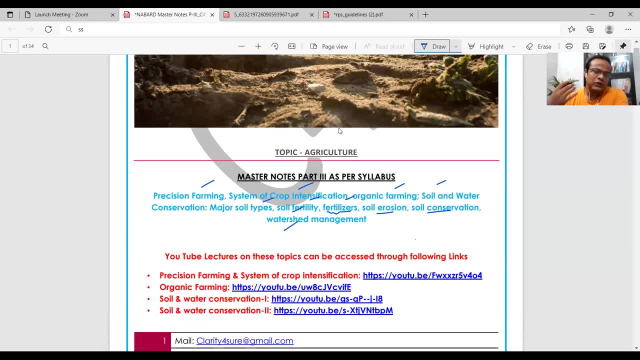 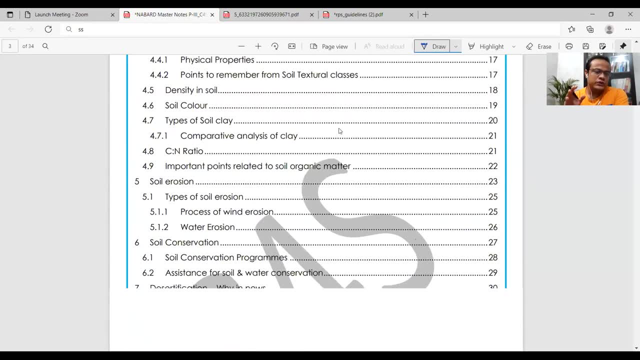 The basic areas, from where they are asking the questions and when you will revise again after this lecture. So stress upon those areas, only right. So as of you, all of you have the notes with you- I will carry on with the discussion As we are discussing. the first topic given by the NABARD is precision farming. 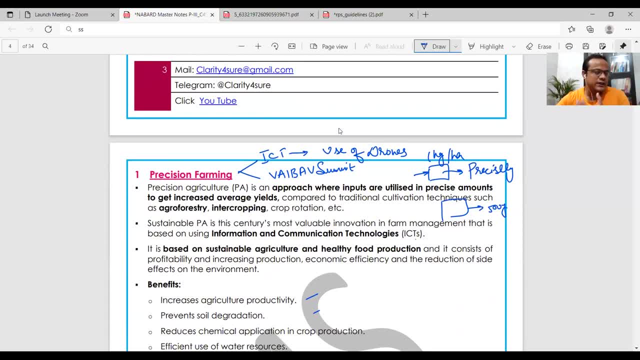 What is precision farming? As all of you know, the term only indicates. what does it mean Precisely? you measure each piece of land, each square feet of land. you are measuring and you are giving your inputs. you are using your technologies as per that. 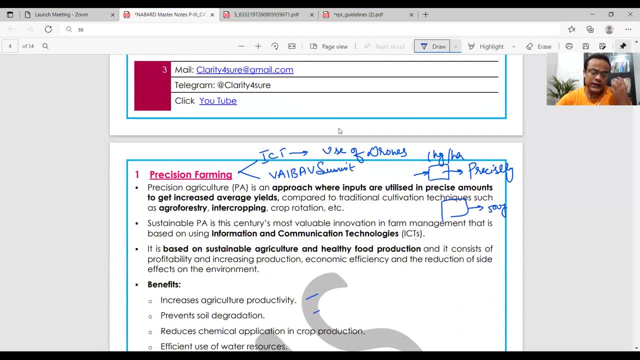 Now the chances of getting the question, what are the chances of asking question from this precision farming- are two. There are two points to remember here. The first is use of ICT. As I told you, ICT question is very famous and UPSC has also asked last year in their prelims related to use of drones. right, 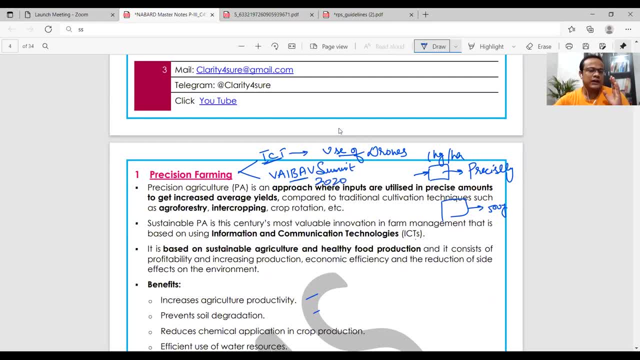 And the next is Wabhav Summit, which was conducted in 2020.. They can ask some questions from here. So these are the two areas from where they can ask the question, from the precision farming. There could be another question. It is simple. They will give one line and ask you which topic was asked. 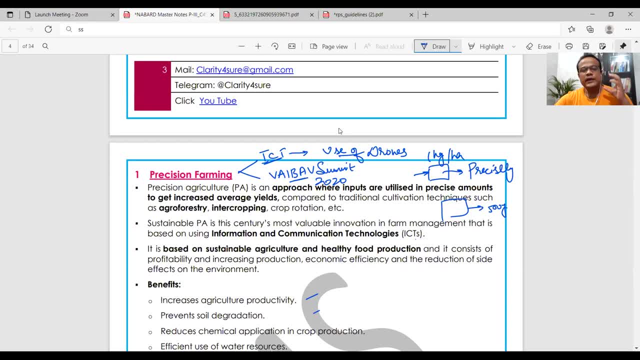 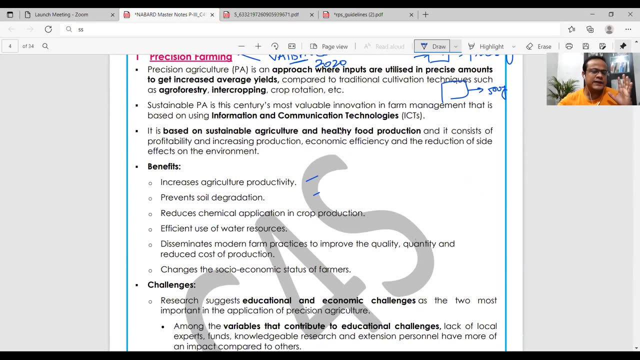 which type of farming it is. So you will easily sort out that this is related to precision farming. as I told you, Here we use input precisely according to each portion of land. Overall, we do not take which we generally use in agriculture. So if we talk about benefits, these are very 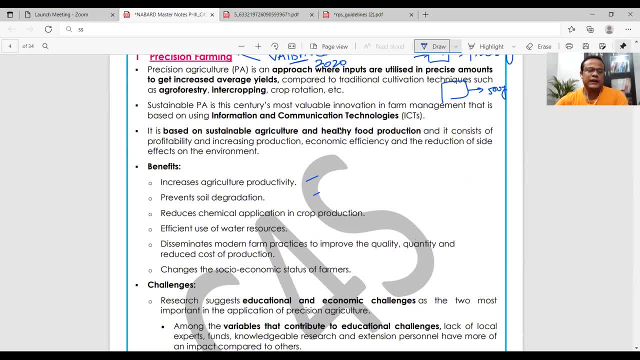 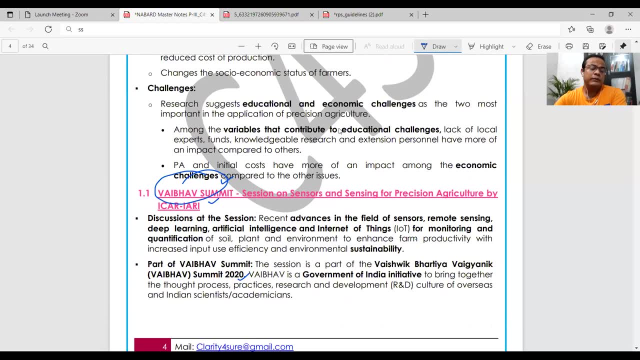 general self-understanding points. I do not need to explain anything in this Now. the point what needs to be explained is this: Vaibhav Summit is very important. What you need to remember is who conducted this. It was conducted by ICR and IERI when here at 2020 and its 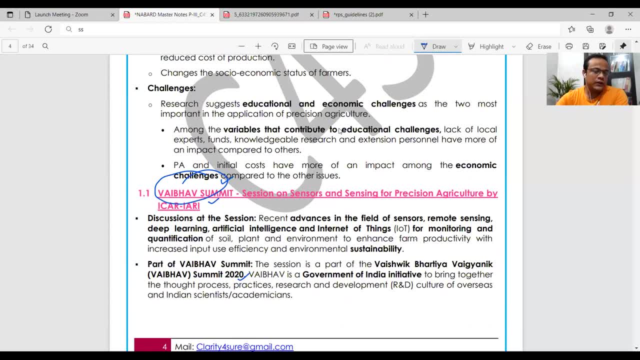 full form. what is talking about right? It is talking about Vastrik Bharatiya Vaigyanik Summit 2020, and in this we discussed all the things like use of sensors. what I was talking about, use of ICT, remote sensing, artificial intelligence- all these things we have discussed. 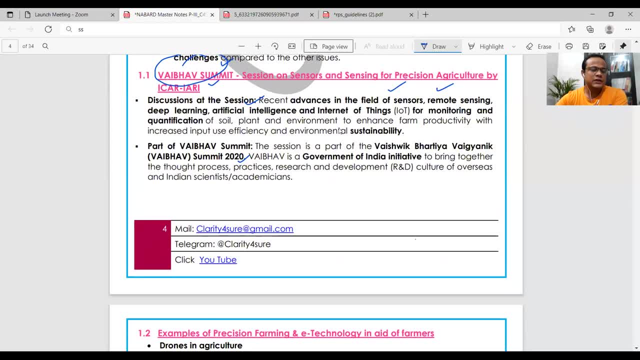 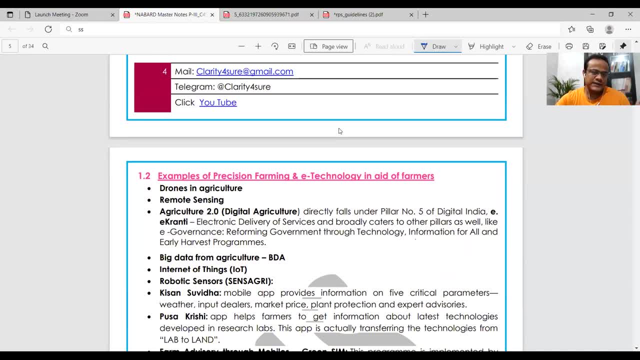 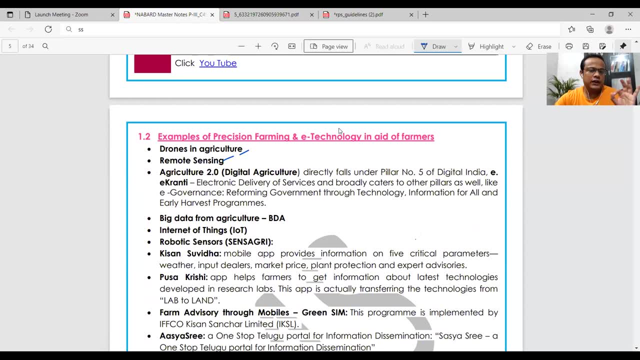 are using the ver parked ICT. Here you have some important things. what I will discuss here. You try to remember this. The first is remote sensing in agriculture, very general- The question may come from here- Digital India program. that is very important as we have. 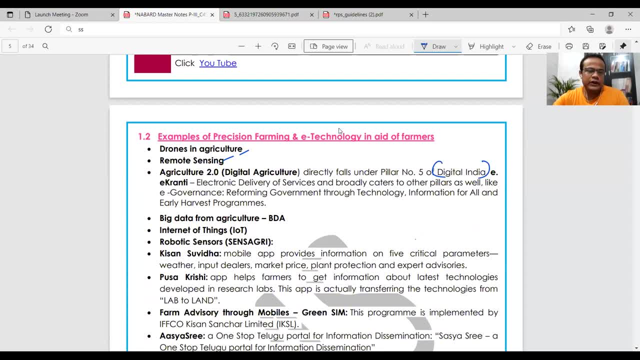 discussed earlier also that when Digital India has been launched, someone will comment in the comment box: when was it launchedLaunch of digital India? Which year it was launched? Very important india, if you can recall, just a guess somebody: 2015, very good 2015. 2015 may launch water and 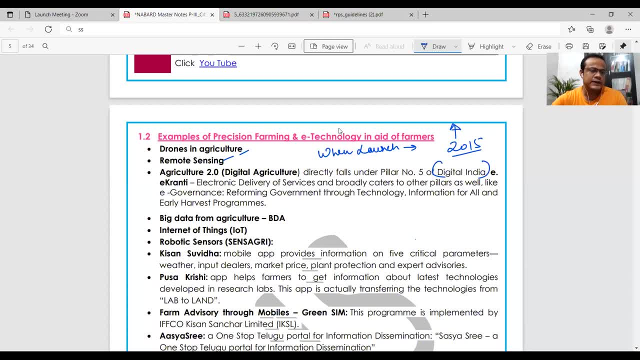 how many pillars it has. that is also important. how many pillars it has, that is also important. how many pillars number five. so it has total no, not six, not eight. total nine. somebody told nine, total, nine pillars. please go through that. please go through this. digital india. it is important, yes, static. 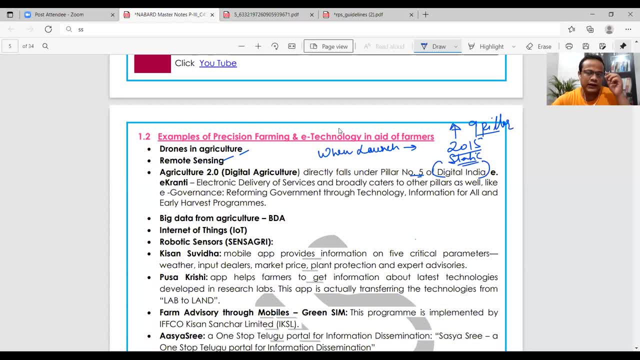 yes, static portion, but it is important, it is very important. i will give one card also for this digital india. it is very important. ticket is nine pillar. today we are talking about the pillar number five. pillar number five is related to work. it is related to electronic delivery of. 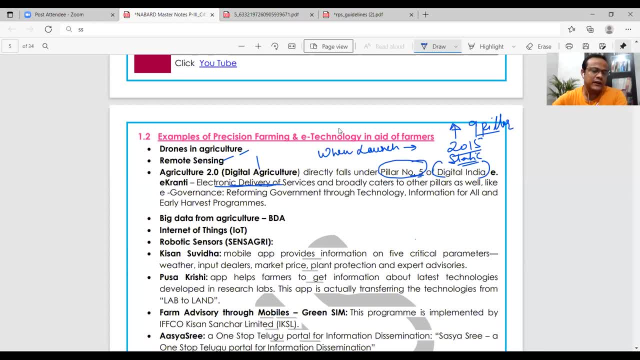 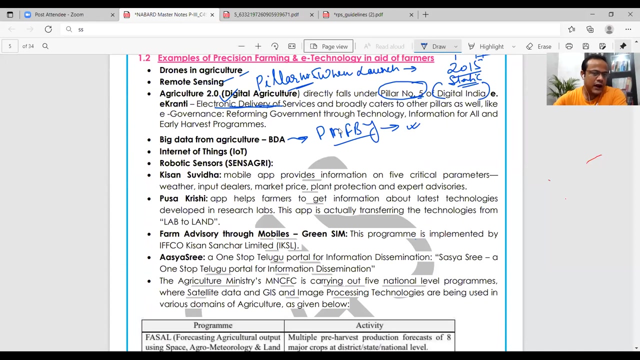 services and e kranti agriculture is. that is pillar number five, candle pillar number five. and let me tell you about wichtig- other services. this is also a very important um. This was also in the news a few days ago. Green Sim is to be seen. Ashya Shree. 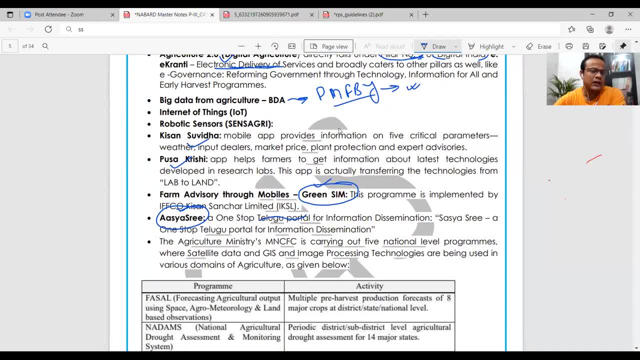 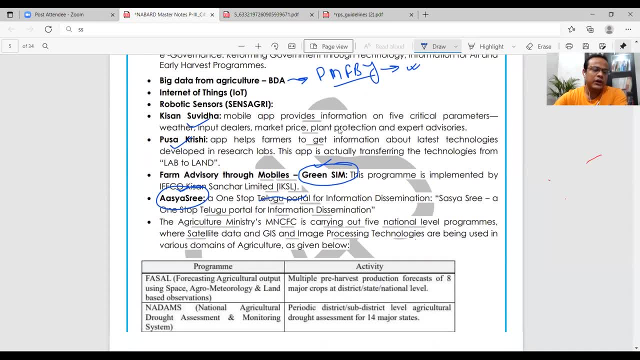 One Telugu portal dissemination is for this. So if you see it from different names, related apps- there is nothing to forget in this. Once you will go through that, you can easily remember what are all the important things Now. these programs are very important. 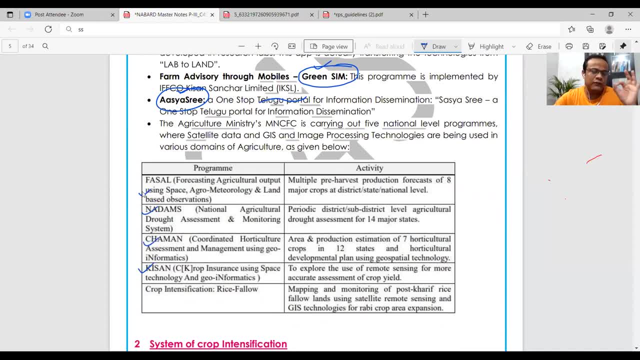 Fasal, NADMAS, Chaman and Kisan, Their full forms and what they are related to, Like Chaman is related to horticulture- Very important. You have to remember this Right In this way. which are the farmers? 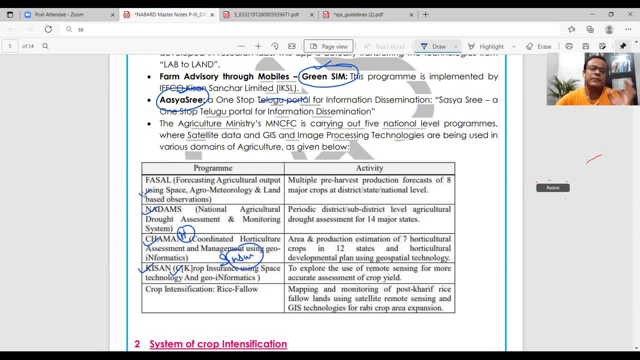 These are related to insurance, Their full forms and what are all their basic purpose. you just have to remember this much. There is no need to remember more than this. So, full form of Fasal. full form of NADMAS. 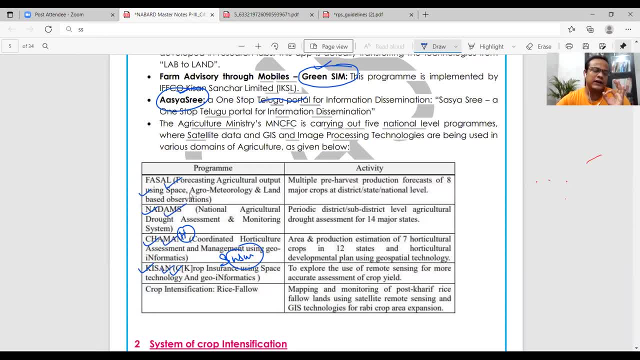 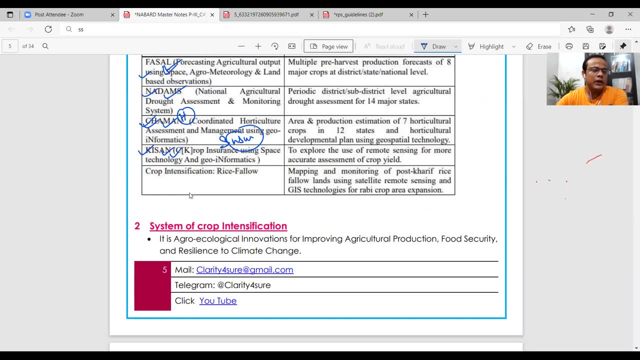 full form of Chaman and full form of Kisan. You have to remember this here. That is very important. Especially, Chaman and Fasal are both very important. Chaman and Fasal are important. You have to remember this here. 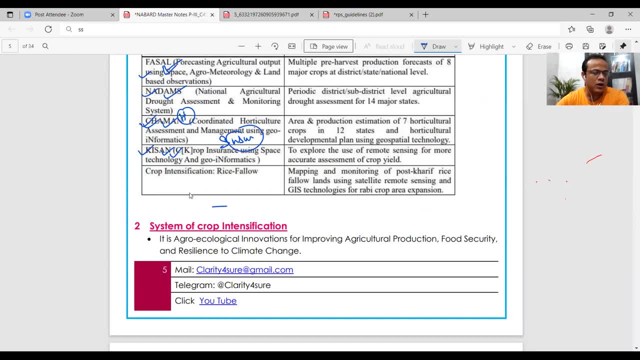 Now we are coming on to the next topic given by Navad, that is, system of crop intensification. We will visit Navad's website. They are working. Navad is doing a lot of work on this, Whether it is wheat or not. 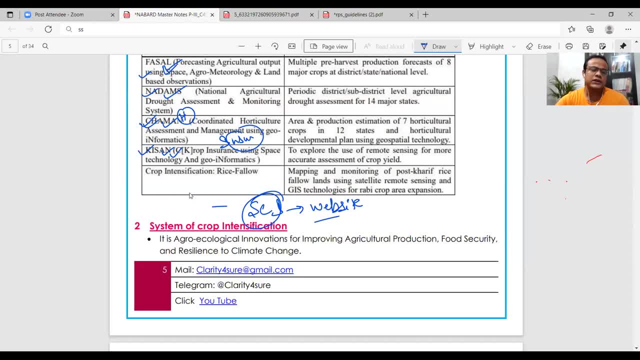 This is not only done in rice, But this system of crop intensification has been followed in wheat. We follow it in maize too, Right? So there is one keyword in this. They can ask one question from here related to definition. The question can come from definition. 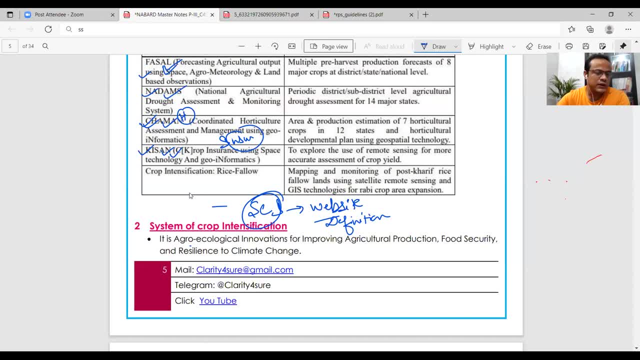 So one keyword in definition that is very, very, very important. You must remember that is agro, ecological innovation A, E, I. This term in itself denotes your crop intensification system. What do we do in this? This is not a technology, actually. 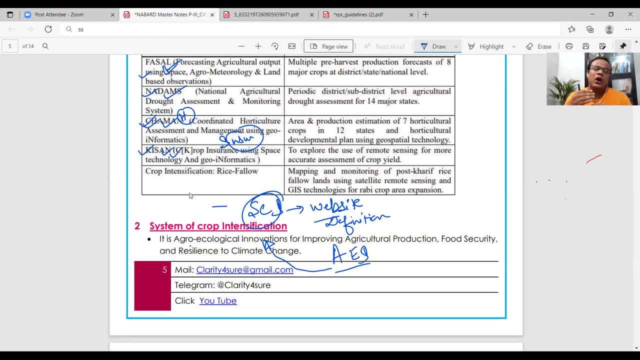 It is innovation. You are innovating some things, And those things are not yet full proof, But despite this, they are giving a best result. In the coming time it can be changed in technological form, But still now, these are what. 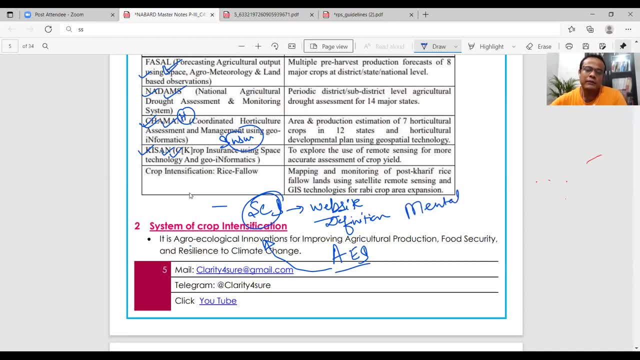 These are mental inputs. Very important term: mental inputs. This is mental input, Okay, Not material input. The general agriculture, what we are following, that is material input. How much fertilizer can we add? How much pesticide can we add? That is material. you are adding upon the agriculture. 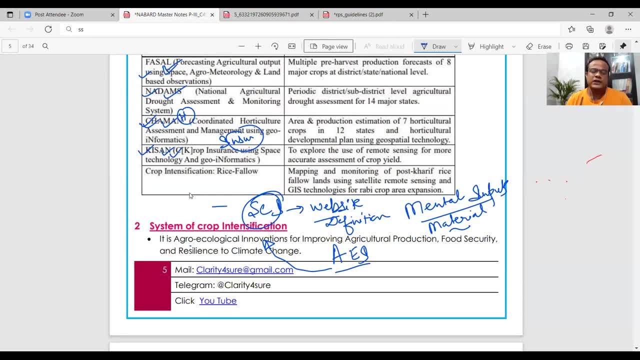 But in this system of crop intensification you are using your brain. Now, by using your brain, you are producing more resources. The best example for that is system of rice intensification. System of rice intensification is very important example for this. 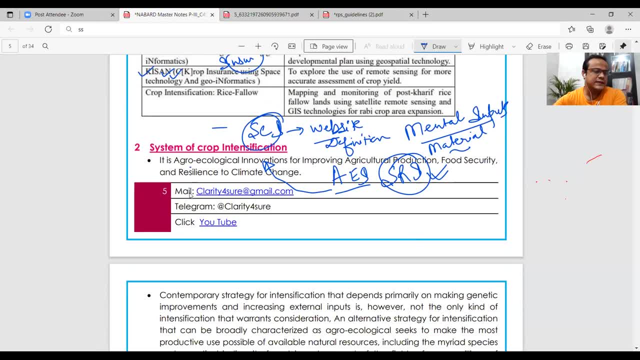 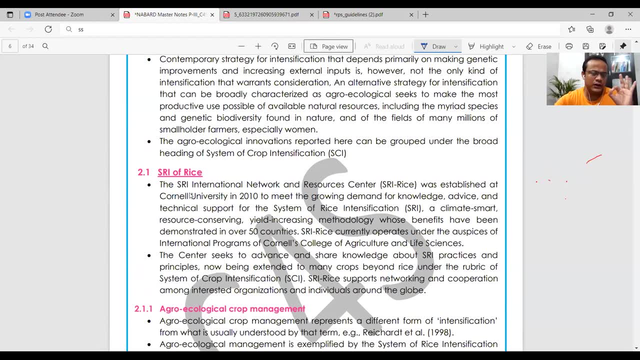 Okay, important example for this SCI, that is system of crop intensification. when we talk about it, So system of rice intensification, you must be knowing from where it came from. That is the first thing you have to remember. The next thing is: anybody can tell me who discovered this? Who discovered this technology? 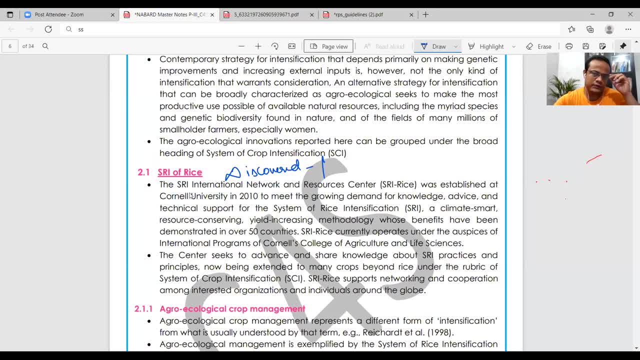 or promoted this technology. Name of the person in which year. that is also important- Somebody. It was discovered in some 1983 by Henry Laulani- this one in 1983.. This person promoted this system of rice intensification. You can remember the name of this person. 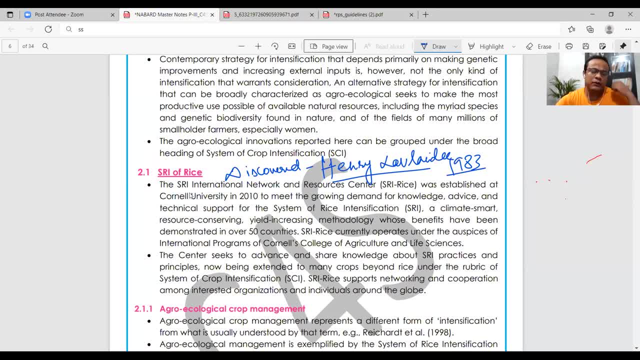 And for this extra information is required. So the extensive work is still going on that I told you that this has not been full proof yet, But all the related work is still going on. at Cornell University, work is still going on related to system of rice intensification. 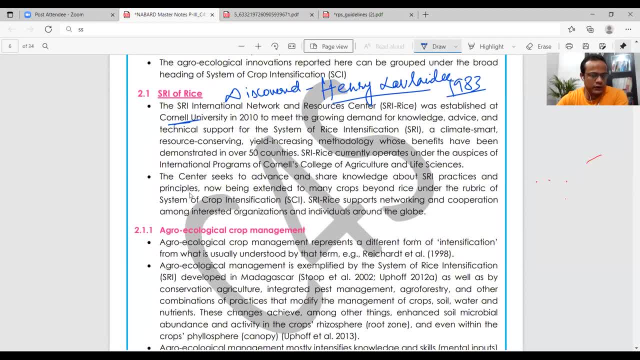 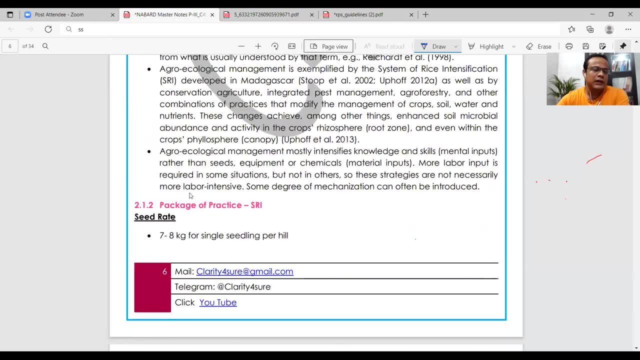 Right, the next question you can be asked from this. we will discuss it as well. As I told you, these are all agro-ecological management. So what all we manage in this? we will see that. First thing is, seed rate is very important to you. 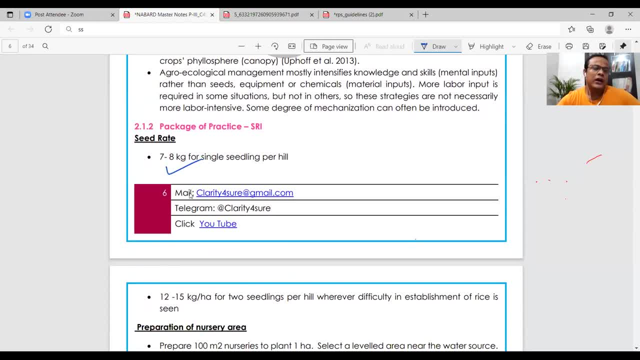 You must remember, in SRA method it is 7 to 8 kg. If you plant a single seedling in one hill, right, If you take one seed, then you will use 7 to 8.. But if you are using two seedlings per hill, then you will be using 12 to 15.. 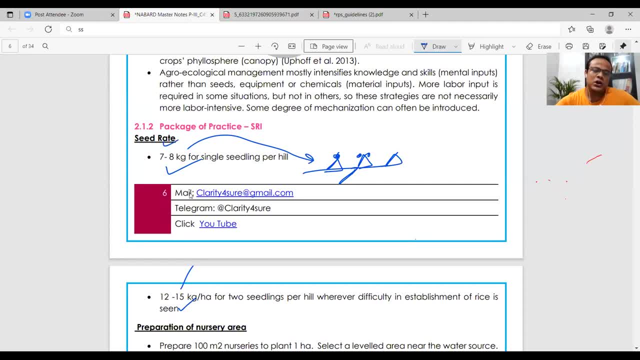 Use this one, So both the seed rates. you must remember If I talk about conventional system. conventional system know this too. Conventional system, the simple paddy we normally grow. what are the seed rates in that? Somebody can tell me? 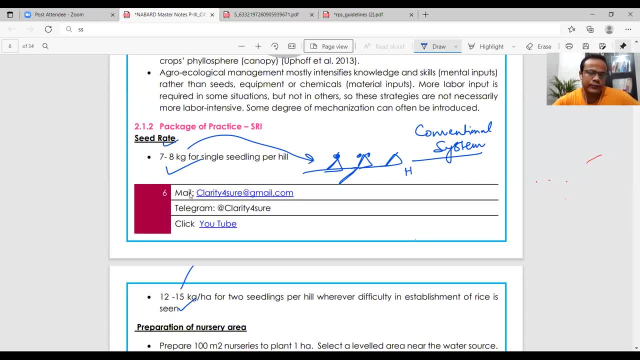 You also remember this a little bit: For hybrids. you can remember for long duration. you can remember for short duration. you can remember for mid duration. Right, You can remember like this: Rahul said it: 100,. the general range is 100, 100 kg per hectare, right, Rahul? that is okay. 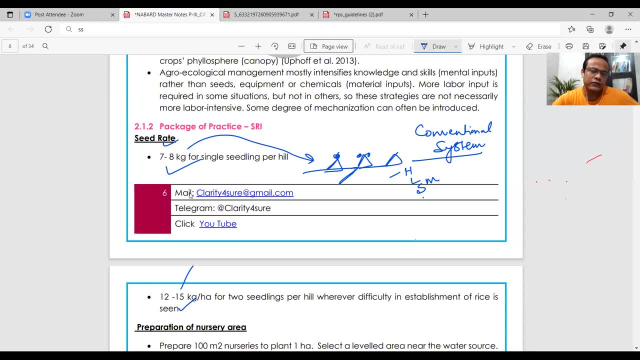 But when you will classify it as for hybrids- it has for long duration, it has for short and it has for medium duration- then the seed rates will change a little bit. So in hybrids, that is What is the most important thing, for hybrids is 20 kg per hectare. okay, you have to remember this. 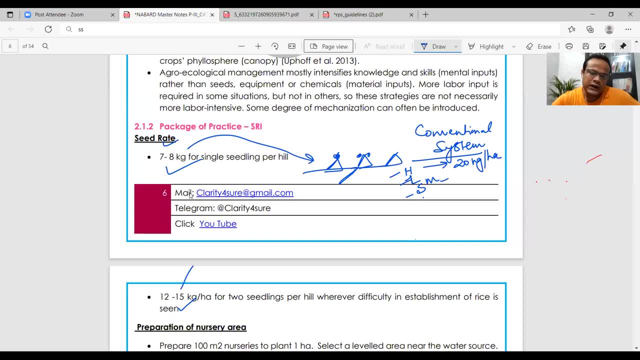 Then in long duration the seed rate decreases a little bit. that is 30 kg per hectare. If we talk about medium duration, it is 40 kg per hectare. If we talk about short duration, it is 60 kg per hectare. 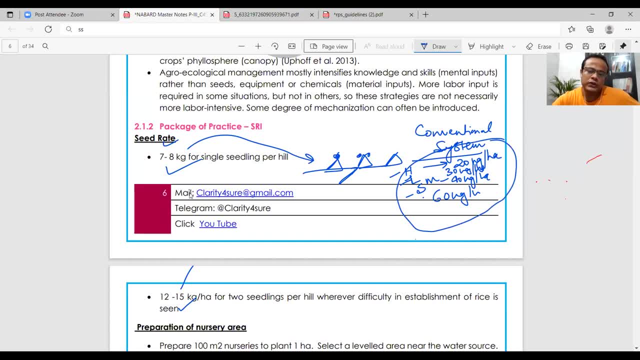 All these TNAU website data has been mentioned, so try to remember this data a little bit. Rahul, that is also okay. Shambhu, that is also okay. Shambhavi: 100 to 125,. that is the general range that you can remember. that is okay. 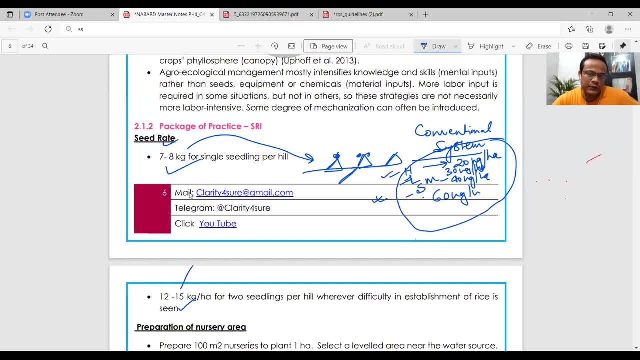 But if you are asked specifically what is for hybrids, remember this too: 20 kg per hectare. Long duration, 30 kg per hectare For medium duration, 40 kg and for short duration 60 kg per hectare. 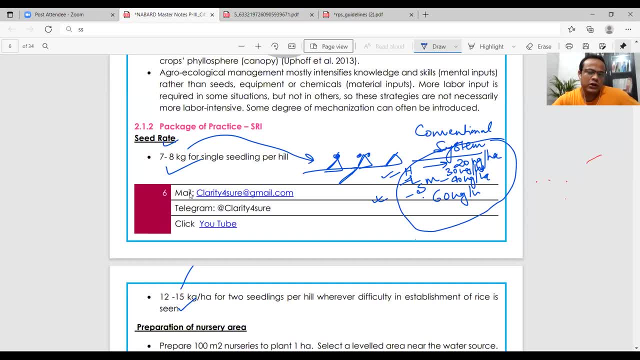 So if anybody can tell me why there is so much variation in long duration and short duration, In long duration you are using 30 kg per hectare, but in short duration you are using 60 kg per hectare. What is the basic reason? 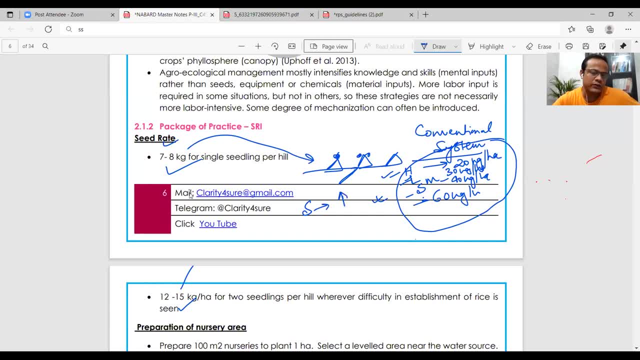 Why is the seed rate increasing in short duration? Why is the seed rate increasing in short duration? Basic analytical question: why it is increasing for short duration varieties. Why is the seed rate increasing? Why the seed rate is increasing when the duration of crop is smaller. 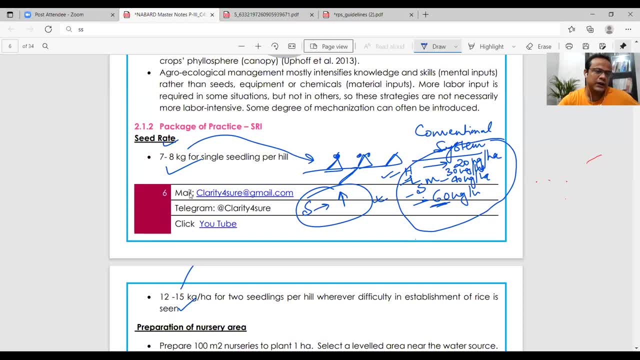 Okay, maximum output is okay, but the basic reason is, whenever the crop is growing for longer duration, its robustness will increase. It will spread more- right, It will spread more. It will spread more. the crop will spread more. 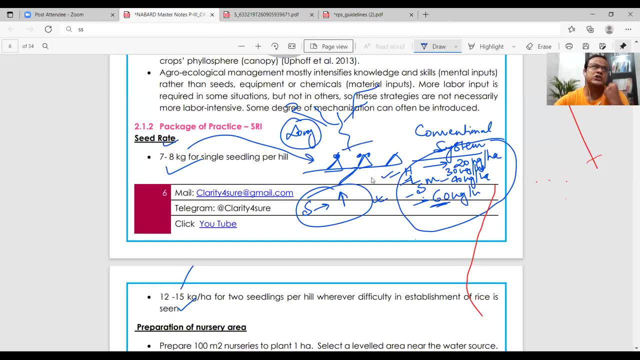 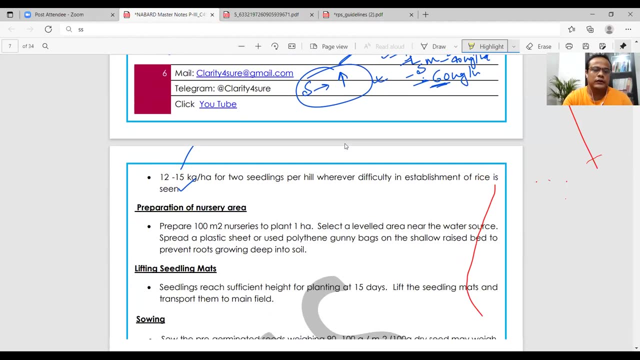 So what happens? because of spreading more What we do in seed rate, in longer duration We keep it less, But the chances of spreading in shorter duration are less. So what happens there? The duration will be less. Okay, You have to remember this. 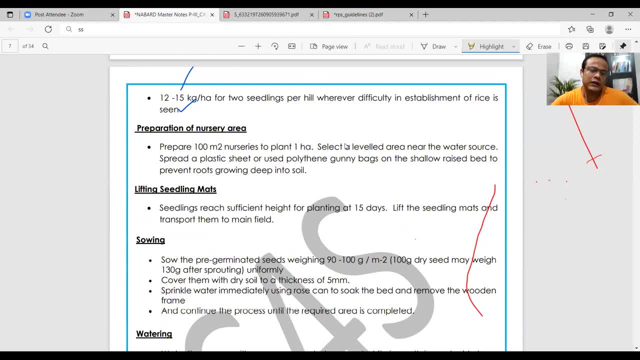 Next, preparation of nursery is very important. We were talking about innovation. Innovation is what we were talking about. Innovation is what we were talking about. Maximum innovation in SRI method is in nursery management. What we do in this. Whatever crop is grown, first thing you need to remember is rate. 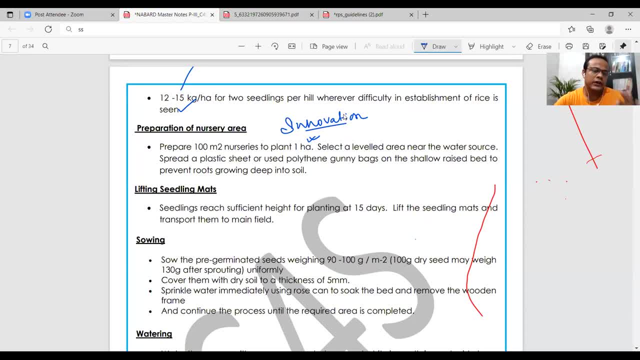 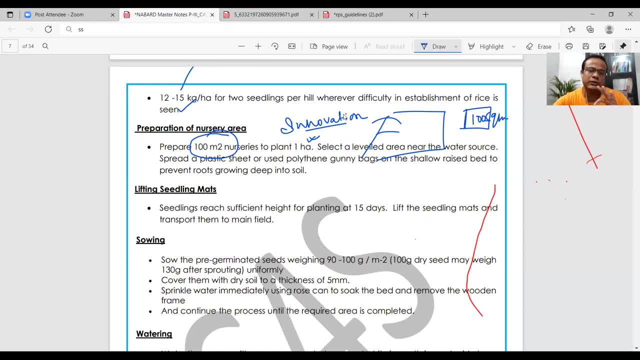 Okay, This is very important question. This you must remember. This question has been asked earlier also. Okay, This is the most important thing to remember. And when you do transplanting, you will do transplanting in two leaf stage in 15 days. You have to transplant in 15 days in SRI method But in normal it goes to around 20 days. We do transplantation between 20 to 25 days In SRI method. within 15 days we go for this transplantation. 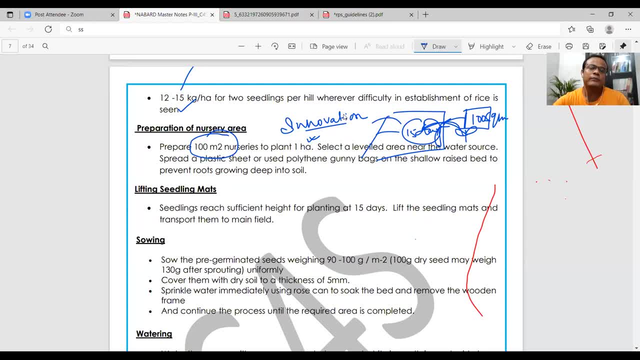 And this is the most important innovation that they have developed in this SRI method. So you have to remember which innovation we have done. First thing is we have reduced the transplantation time. Next thing you have to remember is we always use square system of plantation. 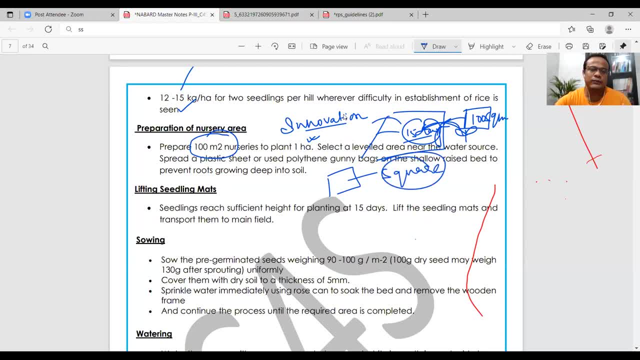 in SRI method. Square system of plantation is the next innovation. Okay, So we are reading this topic under system of crop intensification. As I told you, SRI means innovation, So whichever crop innovation we will study, like SRI is the best method. 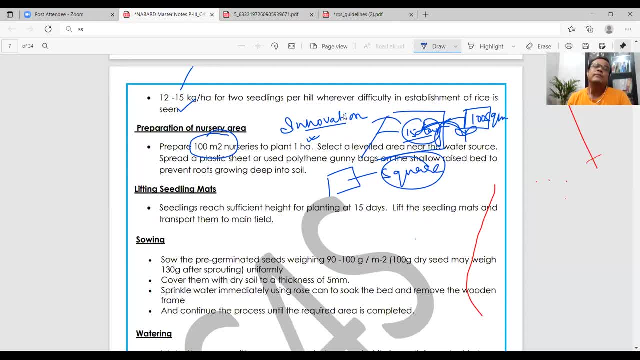 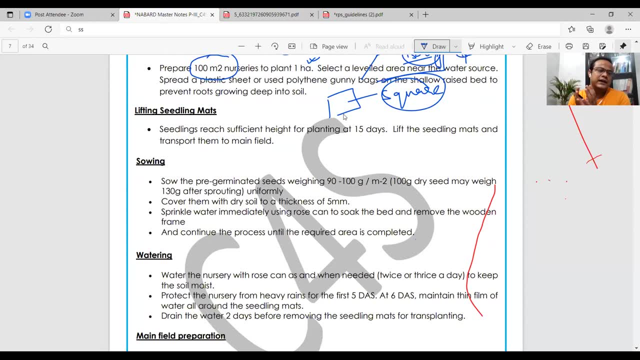 So what all innovations you have done to bring SRI into SCI, those are all becomes important. So you have to see all these points from here. Okay, I think the basic funda of this SCI is clear to everyone. If you can comment yes or no, then I can proceed further. 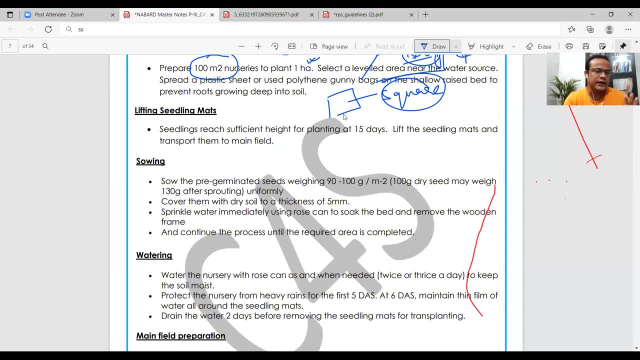 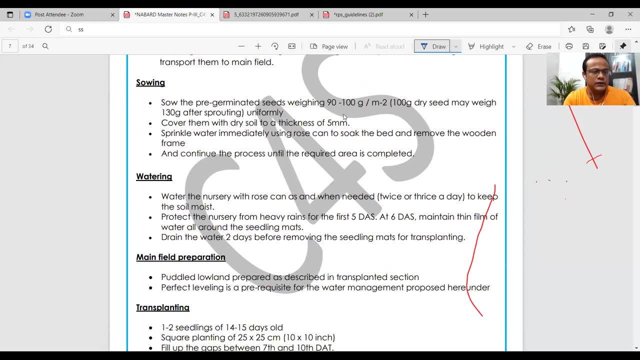 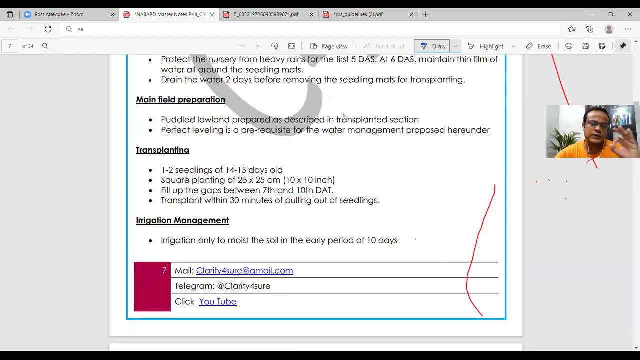 SCI is clear What SCI it is and from where. you have to see basic things. Okay, Rahul is saying yes, I think Rahul has only understood it. Okay, fine, Everybody has commenting. Okay, Let me tell you one or two more things. 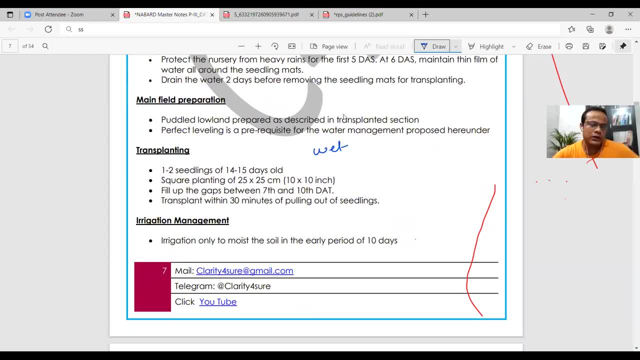 Do some comparative analysis from here: The weight and dry method of nursery. Weight and dry method of nursery: In this we have also discussed that for one hectare you need 100 square meter of area, But weight and dry method, which is the normal method of nursery. 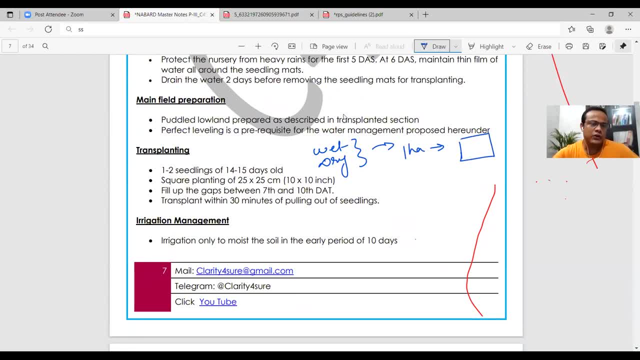 if you have to do it in one hectare, then how much necessary area do you need? What necessary area do you require? Just we discussed- I am repeating it, Just we discussed- that in case of SCI method, the necessary area required for one hectare plantation. 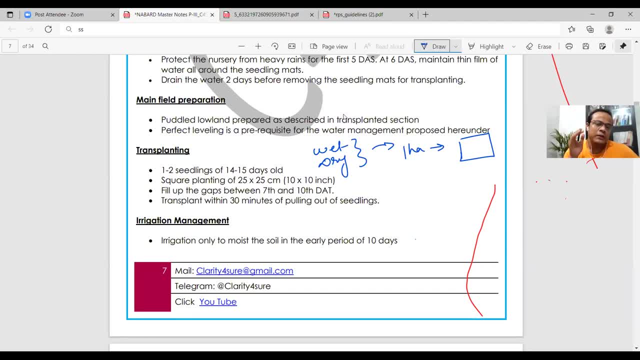 is 100 square meter. But in case of weight and dry method, what is the area requirement for one hectare plantation? This question is also important. If anybody can tell, please comment in the comment box. Nobody, Thousand, Thousand. it is coming. 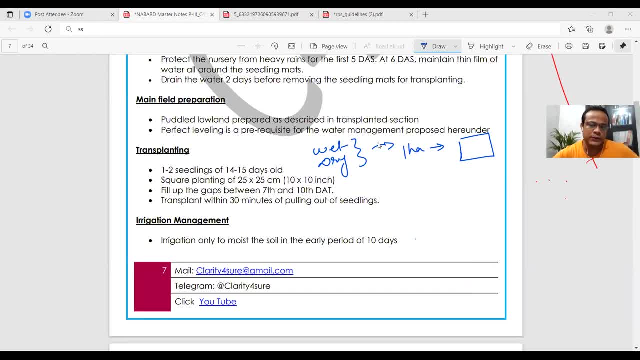 So you have to remember. Akshay Yogita, as per TNO data, 800 square meters. 800 square meters they have given for weight and dry nursery methods that we use. That is 800 square meters, So you have to remember that. 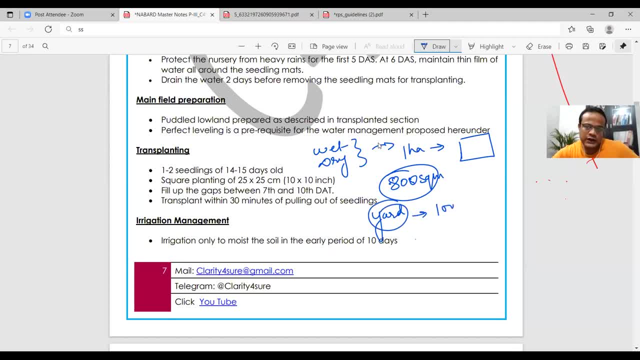 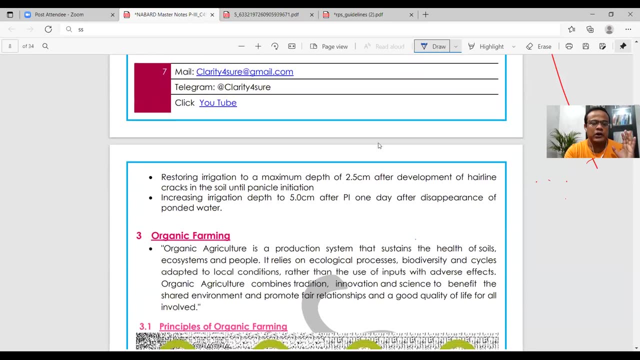 in normal methods. as you said, thousand it is okay, So thousand is normal. if we make it 1 tenth, then we get SRI. You have to remember this too. SRI method is always whatever inputs we do in normal method. 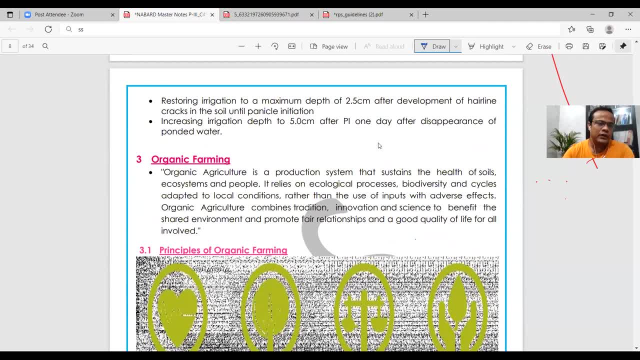 we always use its 1 tenth in SRI. You have to remember this. Now, coming on to the next topic, We have covered two topics as per syllabus. We discussed about the seed rate. We discussed seed rate in SRI. We discussed seed rate in normal method. 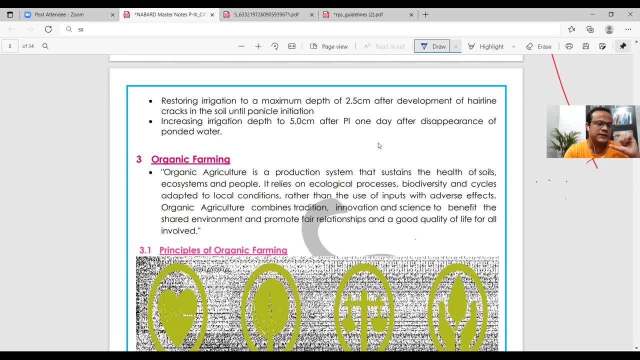 Then we discussed about the nursery area. What is the nursery area requirement? We discussed that too. In SRI it is 100 square meters, But in weight and dry method the nursery area requires 800 square meters. You have to remember this. 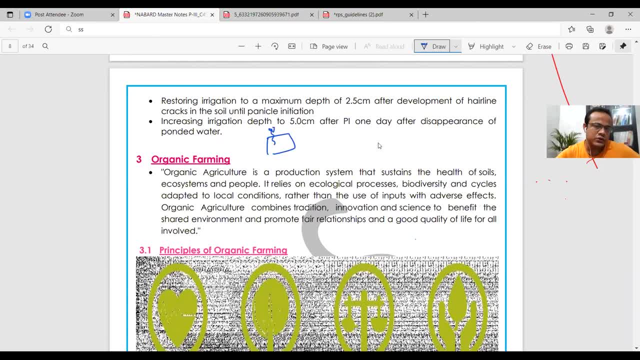 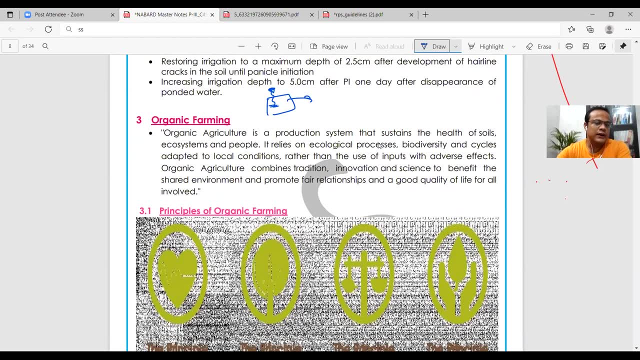 Seedling is the transplantation. When you grow in nursery, the plants are small in size. We call it seedling. Now coming on to the organic farming. That is the next important topic. You don't have to see much in this. Principles are very general. 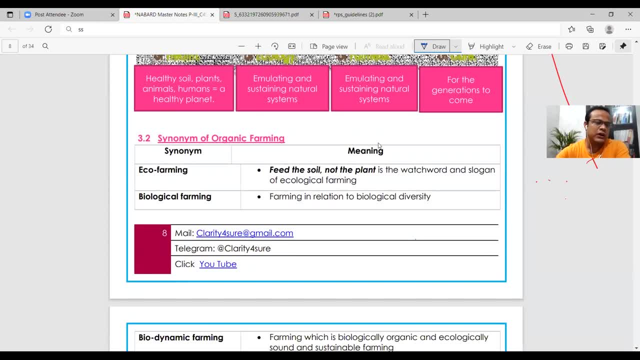 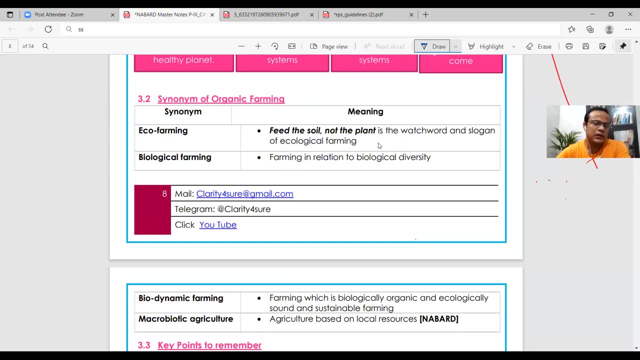 You have to go through once. You will not get the question from here. Question has already come from here. Synonyms of organic farming. Take all the close synonyms of organic farming In grade B. they have asked this question. In grade B. they have asked. 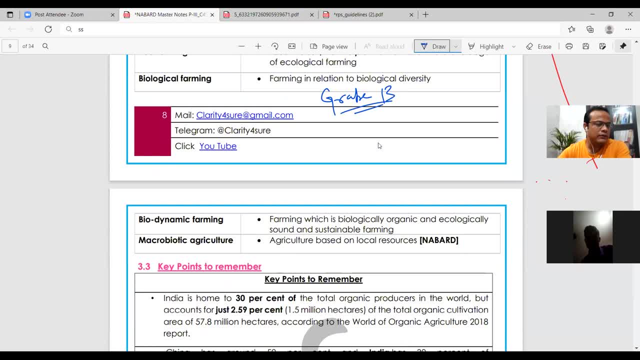 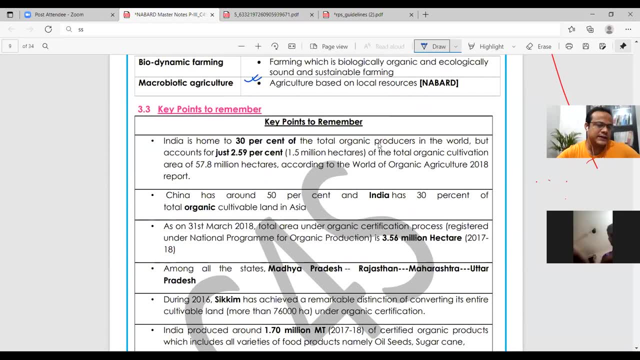 what are all the synonyms of organic farming? Eco-farming, biological farming, biodynamic farming, macrobiotic agriculture- All these are synonyms of organic farming. You can see this. I have given some key points here. You can go through this. 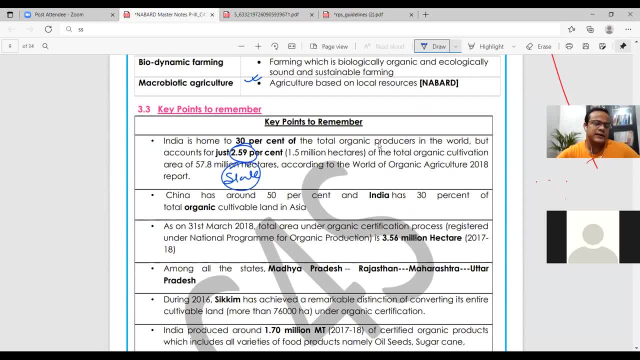 How much percent of organic area is there in India? Which state has maximum organic area? I have given all these statistics. Where is the biggest commercial market? Which country has the most organic land in the world? These are all the important things. You can sort it out from this chart. 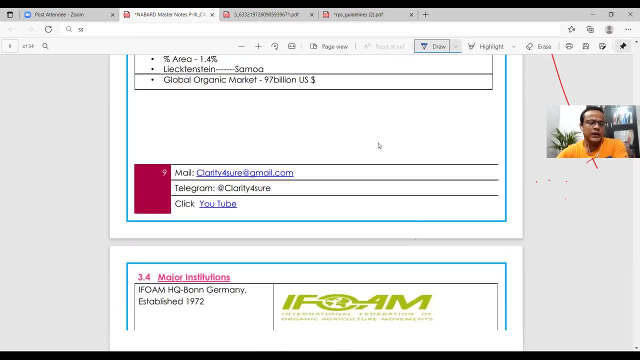 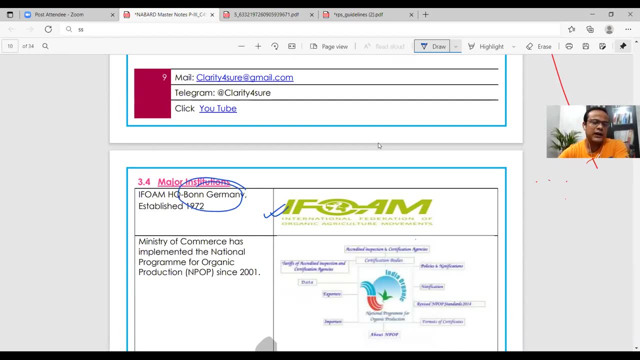 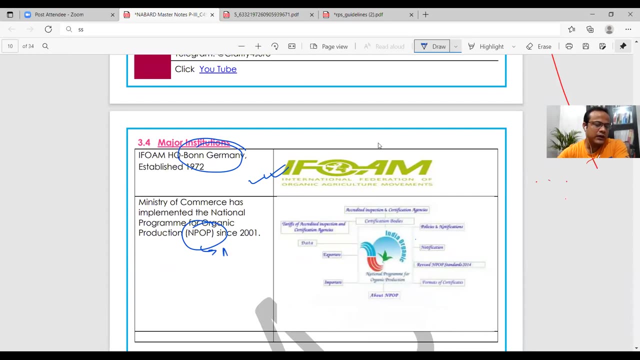 You will see it once. You will remember it easily. If we talk about major institutions, iPhone is very important. Remember that is in Bonn, Germany. International Federation of Organic Agriculture Movement. This is NAPOB. Remember the ministry of NAPOB. 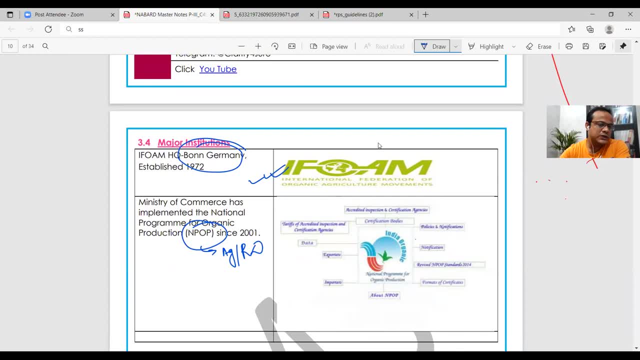 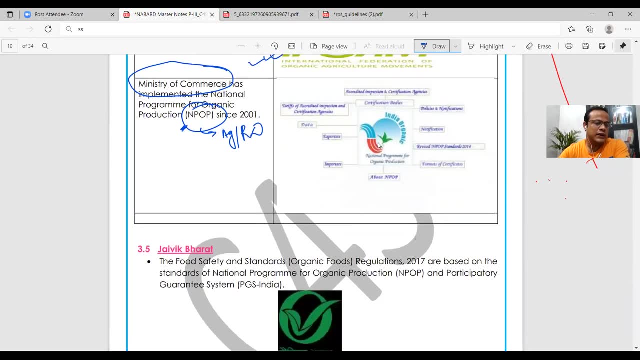 Don't confuse it with agriculture ministry, Don't confuse it with rural development, But it comes under Ministry of Commerce. NAPOB comes under Ministry of Commerce- Very important. Don't get confused. Who developed Javik Bharat Logo? Who developed this? 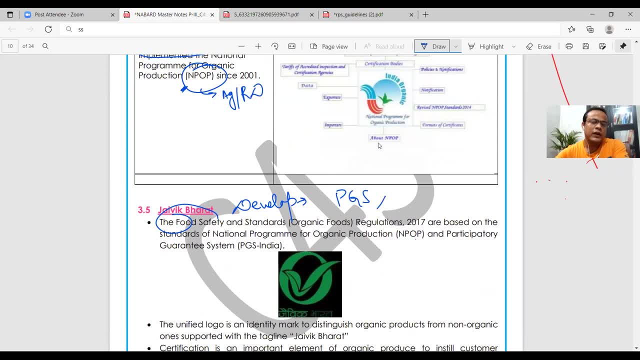 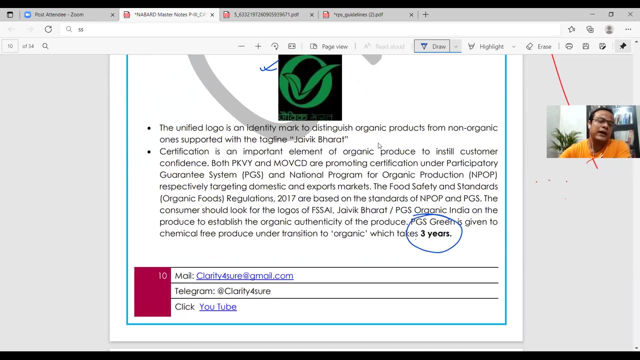 This is important. It was all developed together: FSSI, NAPOB- All of them together developed Javik Bharat Logo. All of them together developed this. All of them together developed this. This becomes important. Another thing is that 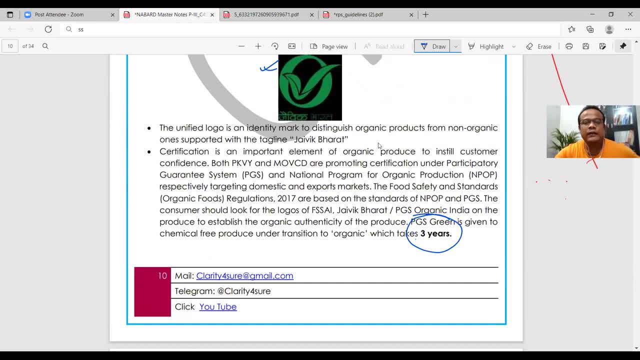 you get 3 years conversion as per NAPOB guidelines. Assume you have land That is inorganic land. Now you want to grow organic. So the inorganic concentration here, the time period given to finish this when you want to convert from inorganic to organic. 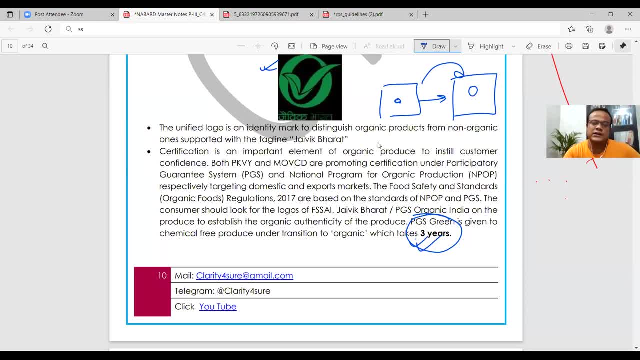 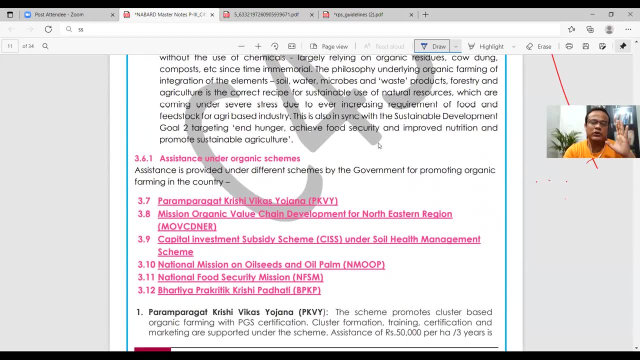 that time period is 3 years. This you can remember. This is very important. Now, coming on to the schemes, All the schemes related to organic. First of all, you should know that Here the question can come: which of the following scheme is not related to? 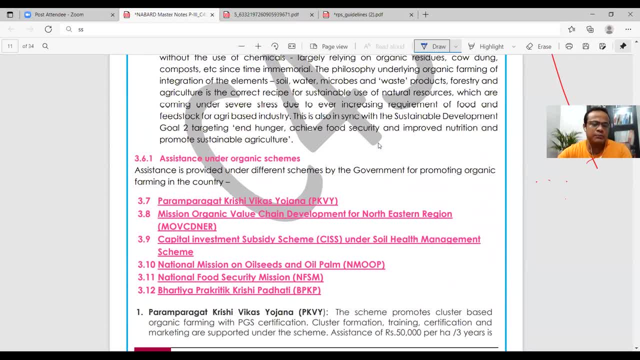 promotion of organic agriculture in India, So you can come quickly there, because we always study about PKVY from organic agriculture, So don't miss all these. All these schemes are promoting organic agriculture, Whether it is PKVY, MOV, CDNER. 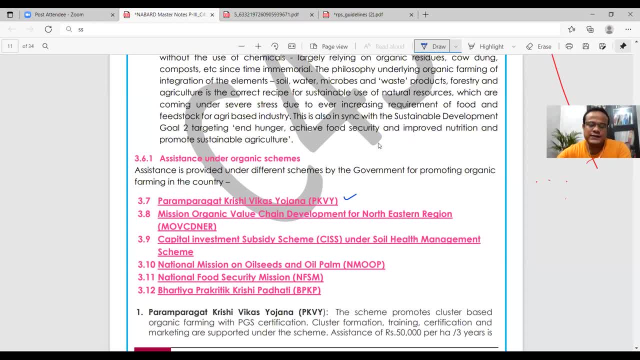 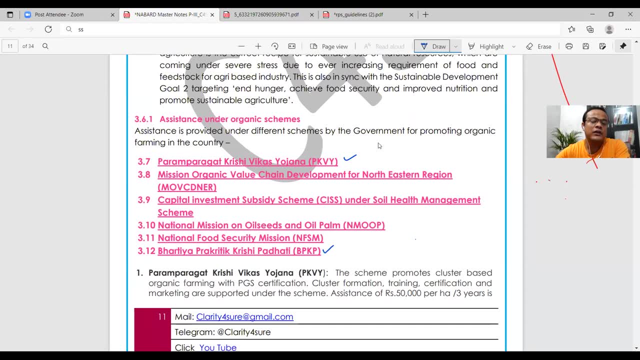 CISS, NAMOOP, NFSM or recently, there is a lot of news about this. So BK, BP, KP, you can see about this Very, very, very important, Especially what assistance they are giving in all these schemes, Or what assistance they are giving. 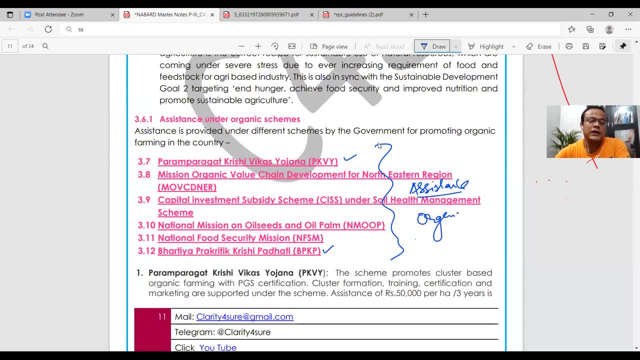 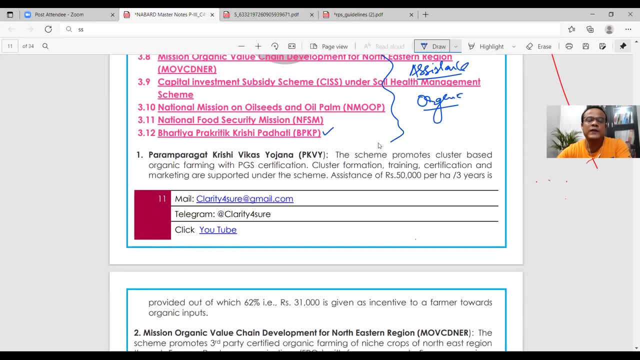 in all these schemes to promote organic agriculture is very, very, very important. Like PKVY, they are giving assistance of 50,000 per hectare for 3 years. So you have to give in examination It can be done per 2 years. 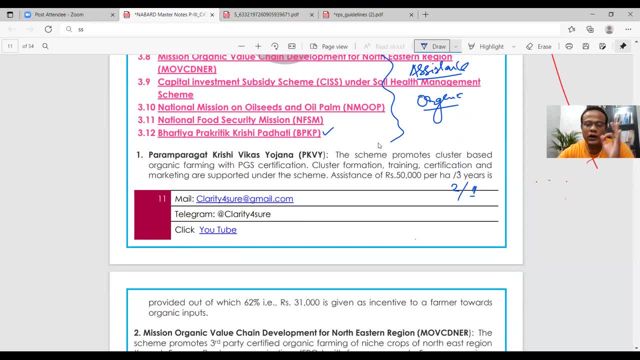 it can be done per 1 year, But you have to keep some patience. You have to read all the options and clearly see that 50,000 per 3 years. you have to tick that. That will be the right answer. Here it is split like: 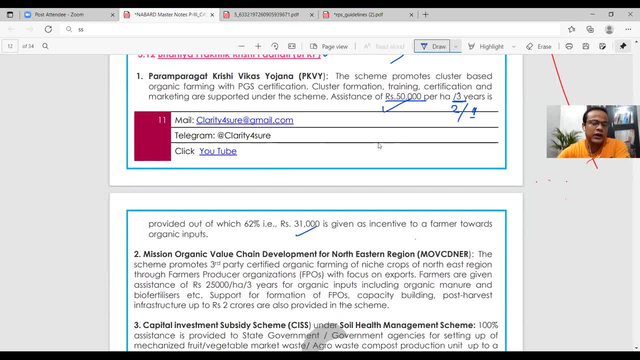 31,000 is given for organic inputs out of this 50,000.. If we talk about cluster formation- cluster formation, PKVY- then how much assistance is given in this Anybody? So cluster formation under PKVY: what assistance do you get from the government? 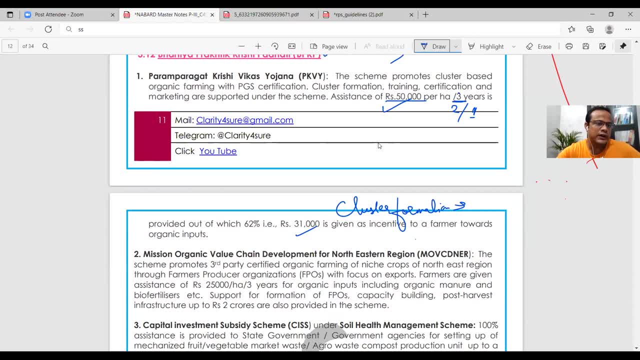 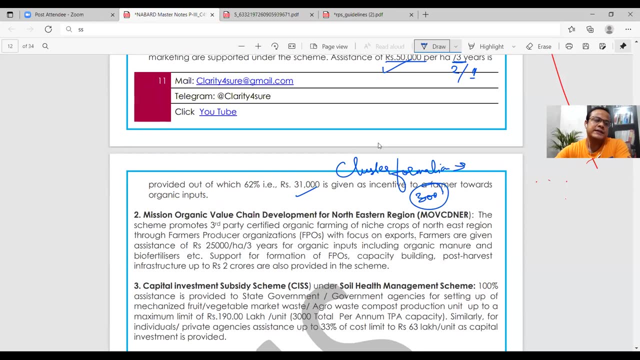 Siddharth: 3000, Venkatesh: 8000. So no, it's not 8800, it's 3000. So you have to see all these facts, you have to revise and see in which you are given the assistance. 3000 is the right answer. 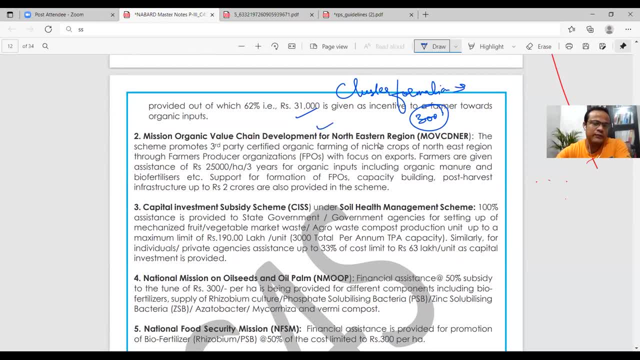 Now mission: organic value chain development for north eastern region. Now you will see in PIB whenever there is talk about organic agriculture, then the government is discussing about this scheme that you are promoting, that you are promoting organic agriculture in the north-east. So you can see when this scheme was launched. 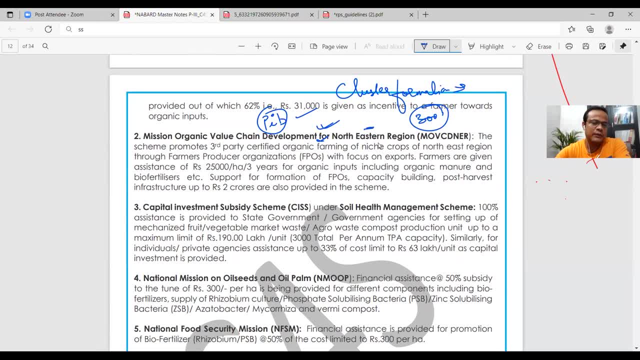 you can read a little about it in detail. I have already given the details about it. And look at the assistance in this. there was 50,000 in it, so here the assistance is 25,000 per hectare for 3 years. So you can see a little difference in this. 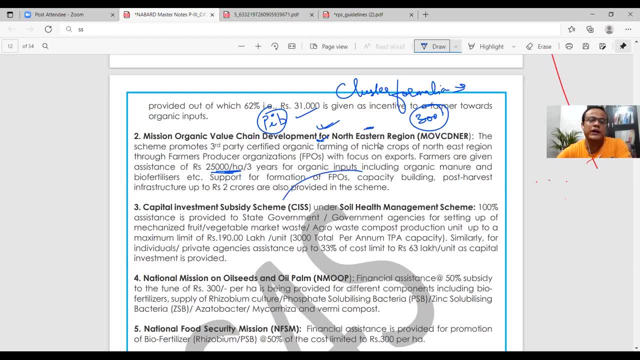 Capital investment or CDA scheme that is more important. it comes under SHM Soil Health Management Scheme and there is some difference in SHC. that I told you in the group. what is the difference between Soil Health Management Scheme and Soil Health Card Scheme? what is the basic difference? 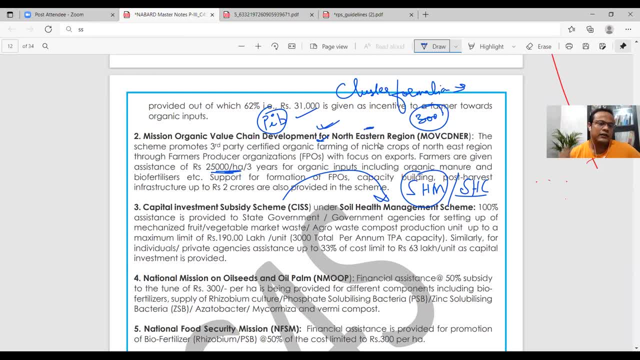 a very beautiful card was given in the group. who has read that, he or she can easily tell the answer for this question: What you are promoting in SHM, what you are promoting in SHC- Forgot, Not covered. So please go into the channel. Telegram channel at clarity4sure. 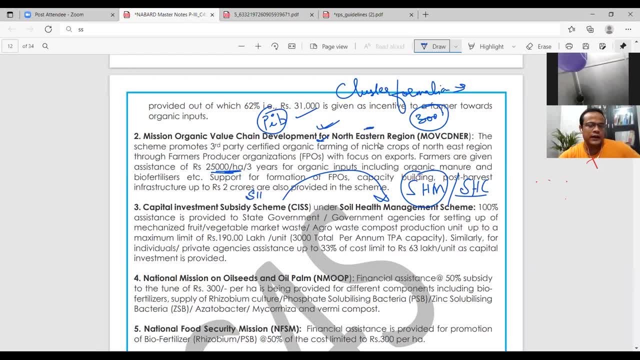 go there and see- very beautifully it is explained in a card- what you promote in SHM, what you promote in SHC and what is the difference in the basic two. So don't forget all these important things, very important. now coming on to the next, that is: 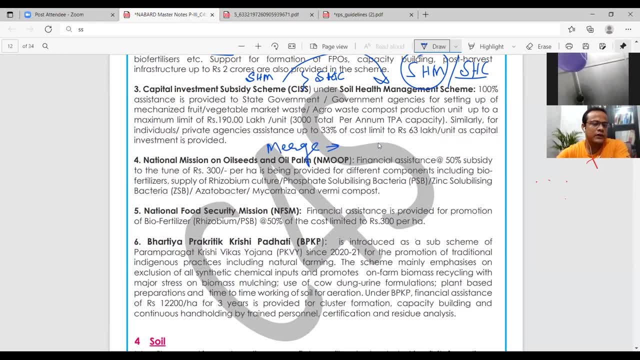 NAMOOP. NAMOOP has been merged. under which program? It is National Mission on Oilseed and Oil Farm. but why this is promoting organic agriculture. because it is promoting bio-fertilizers. NFSM, very good. NFSM has been merged, so it is promoting bio-fertilizers. 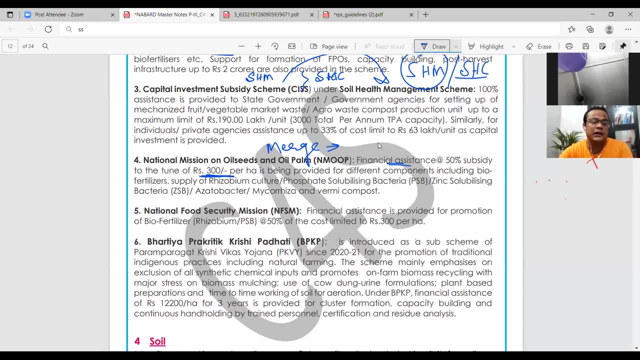 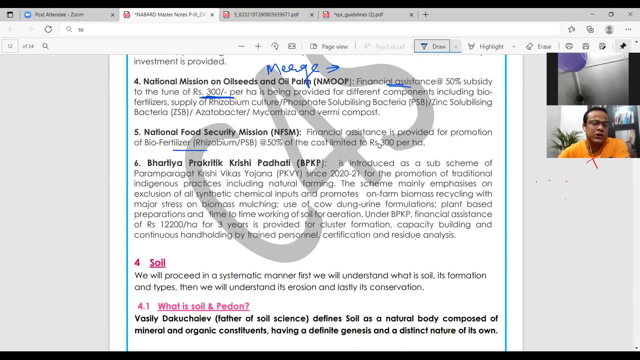 what subsidies you are getting. you can see in this. if we talk about National Food Safety Mission, there is a subsidy for bio-fertilizers, and what I was lastly talking about is BP KP. you can see about this. this is also important because this is being covered daily. 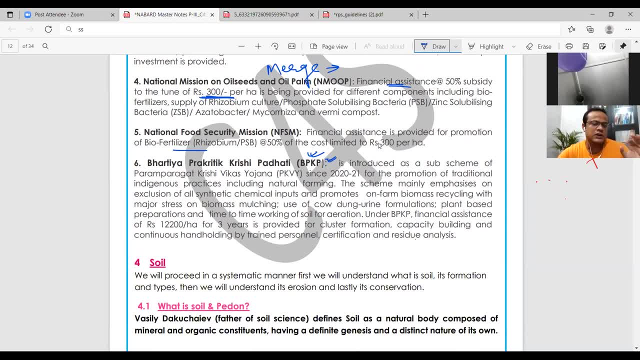 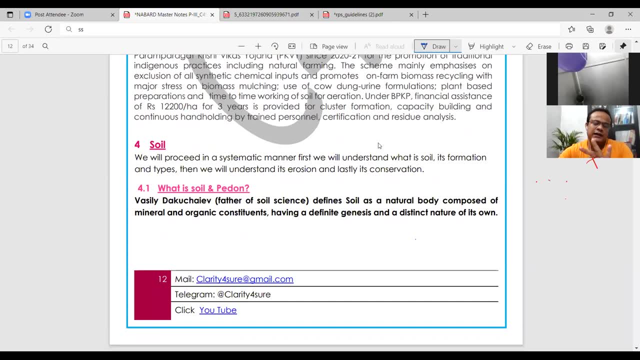 whenever there are reports of Ministry of Agriculture, they are always covering about this scheme. this year, this scheme can be important. this year this scheme can be important. now, coming on to the basic of soil, we have seen three topics. you understood from where you can get questions. now we are moving on to the soil science topic. 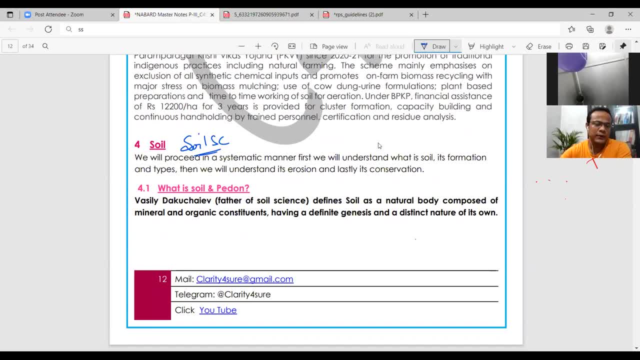 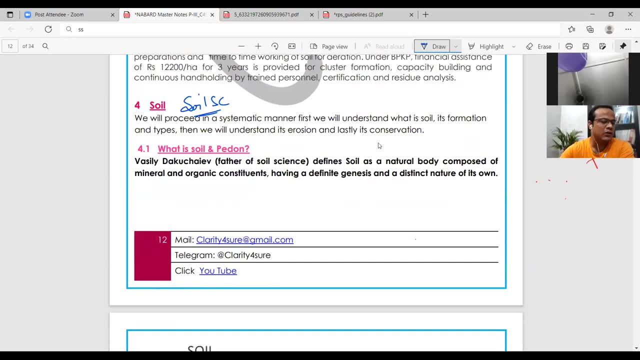 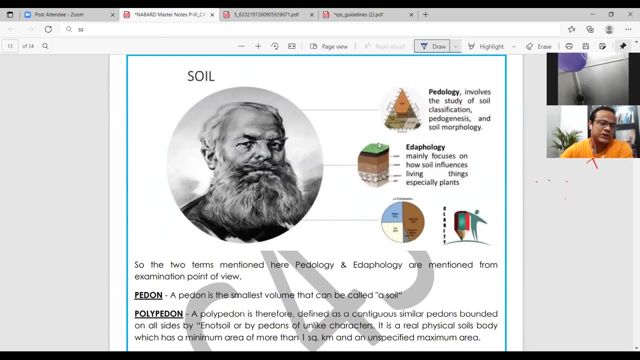 you have to see some basics. you don't have to go in detail for agriculture generalist students. if you are preparing for land development, you have to go in detail, not in the prelims. who is called father of soil science, DAKU CHEV? now coming on to the soil: 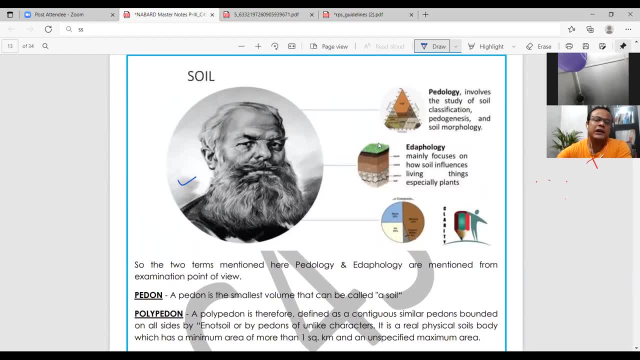 this is DAKU CHEV. you have to understand these terms clearly. generalist people: you can get questions from here. what is PEDOLOGY, what is EDEPOLOGY, what is PEDON and what is POLYPEDON? these four terms are very important for you. 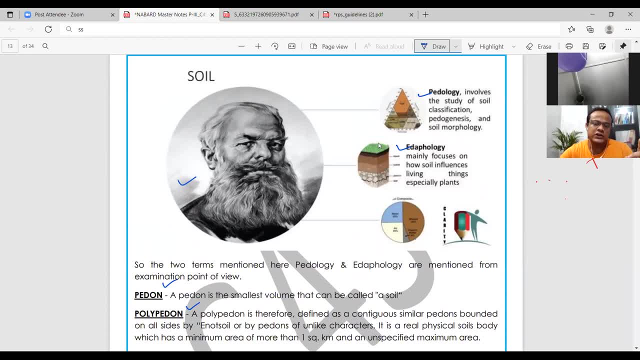 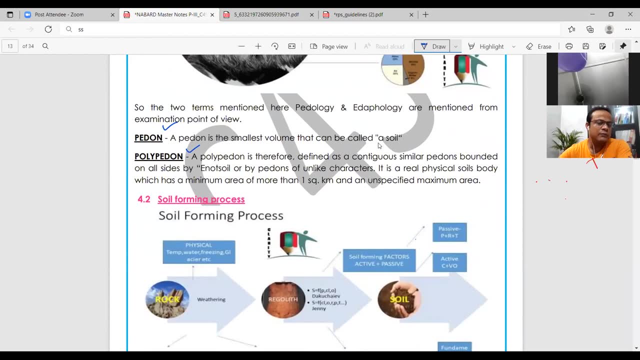 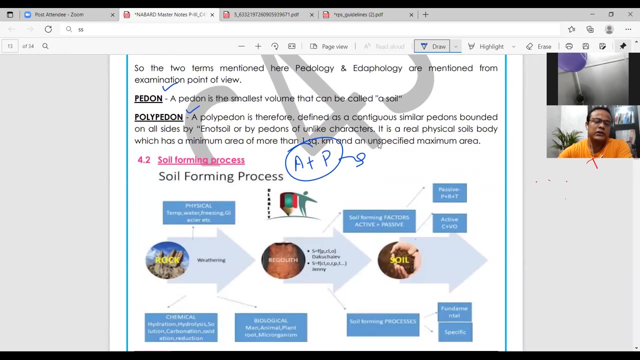 by looking at the definition, you can get all the options. what does the definition is defining above? so it is very clear: what is PEDOLOGY, what is EDEPOLOGY, what is PEDON and what is POLYPEDON? now, from the soil forming process. 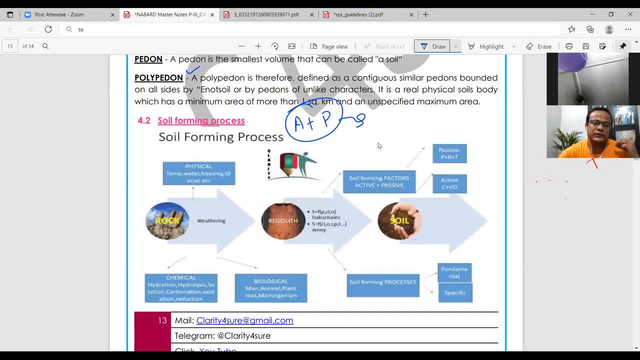 only one question comes that can generate energy. so here climate plus organism are active forces. here climate and organism are active forces. if we talk about passes, parent material and parent rock, topography and time, these are passive forces. so remember the classification of these two. generally, a question is asked from here. 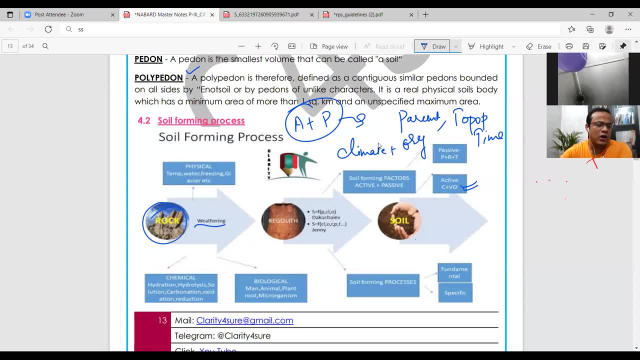 rock will be withering. after withering of rock, it forms the regolith. generally, a question is asked: what is the precursor of soil? what is the precursor of soil? the precursor of soil is- you have to remember this term- that is, regolith, again an important term, like EDEPOLOGY. 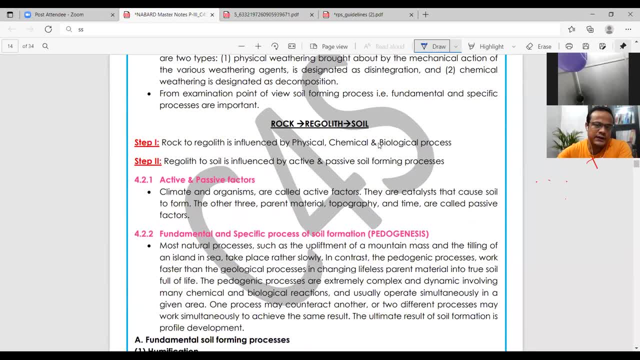 this is also an important term. now we come to the formation. this is a basic process: from rock regolith forms, from regolith soil forms. I have just told you about active and passive factors. now two things come here, that is, fundamental soil forming process and specific soil forming process. 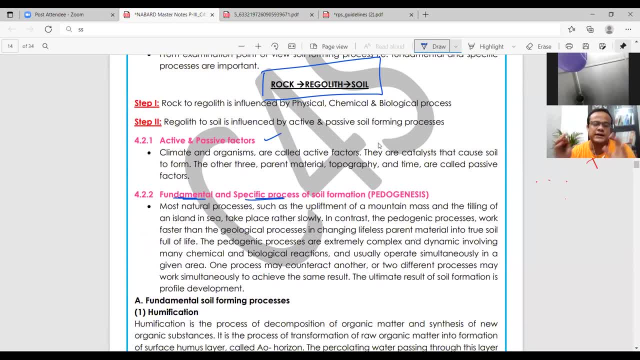 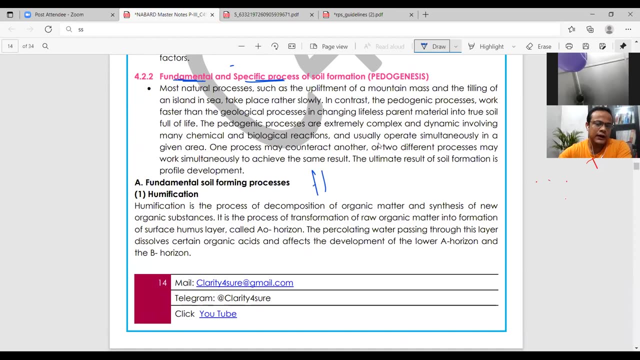 so which are the fundamental and which are the specific? keep a basic idea. this can be given by mixing. which of the following is not a fundamental soil forming process? so what will happen in that? one more out will be given. there are three processes in fundamental, that is HIE. 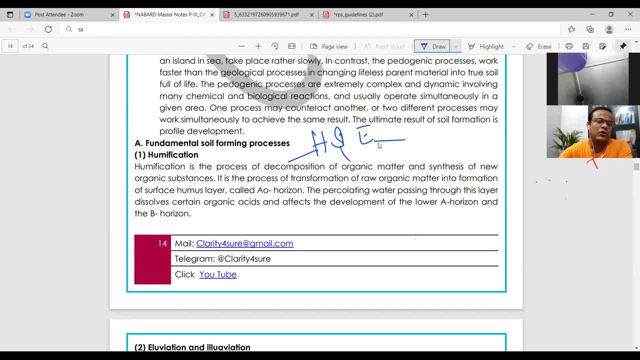 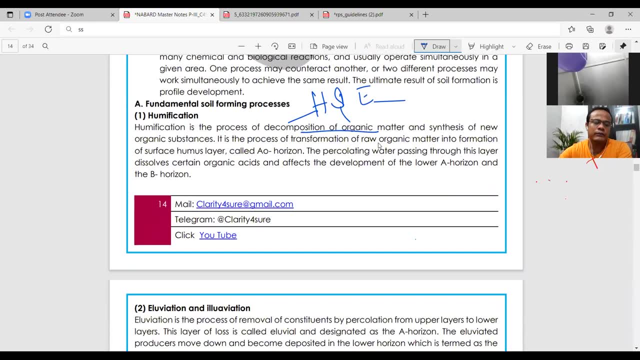 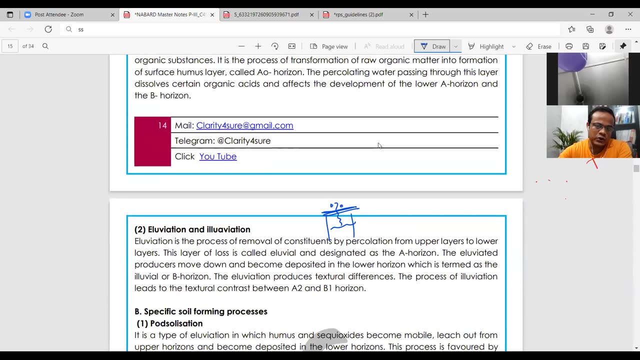 humification, alluviation, these three, you have to remember. that is fundamental. humification is decomposition of organic matter. alluviation is the surface of the soil. from here leaching is done. whatever material is going down. suppose nutrients are in the soil, this is being leached with the water. 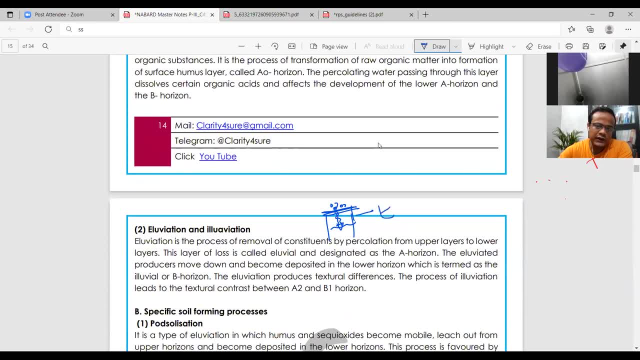 and it is going down. so the process is going down, this is called E alluviation, and when it is deposited, it is called Iluviation. I for in that we call it as Iluviation. so these three are fundamental soil forming processes. Rohit, wait for some minutes. 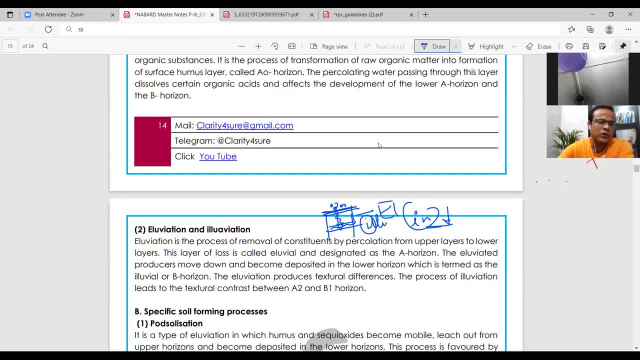 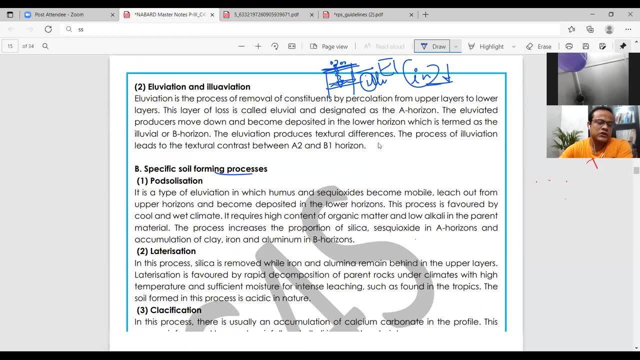 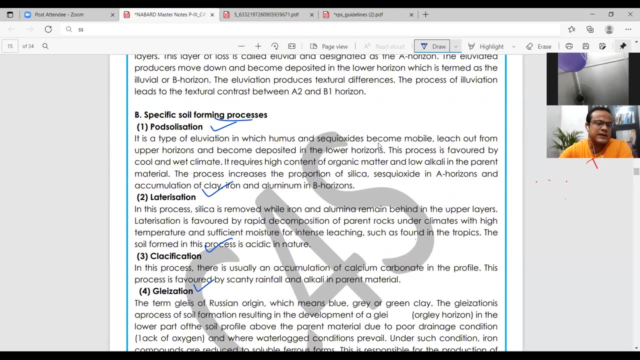 you will get the origination. soil will be formed. after that you will read the origin or you will read the origin first. now coming on to the specific soil forming processes. in specific, what will happen? porzolization, lateralization, calcification and glagization. 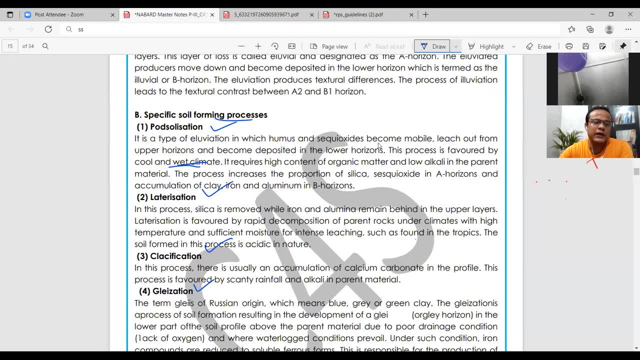 so when we talk about porzolization, it happens in cool climate areas. when we talk about lateralization, it happens in hot areas. so lateralization itself denotes that is deposition of calcium. what happens in porzolization? it is a type of Iluviation. 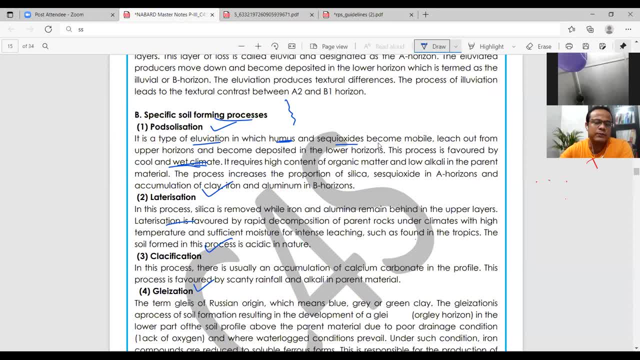 we understood what is Iluviation. material is going down in which the humus and sesquioxides becomes mobile. the humus content in the soil, or sesquioxides, move down. now the question comes: what are these sesquioxides? sesquioxides are such compounds. 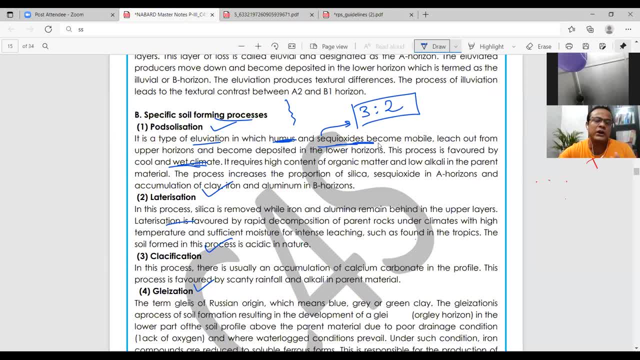 in which oxygen is 3 sesquioxide. what is the movement? porzolization, that is, in cool climate areas. if we talk about lateralization, this process of silica is removed. the iron compound or the silica in the aluminium compound comes down, so we call it lateralization. 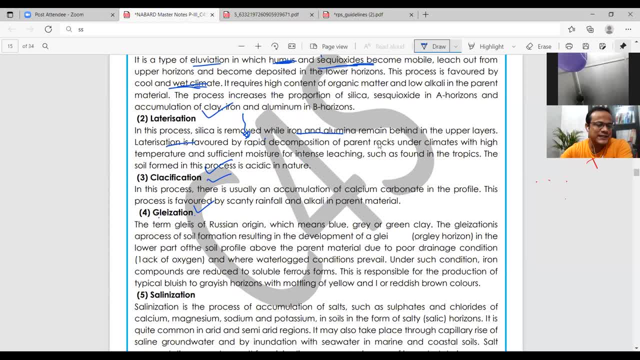 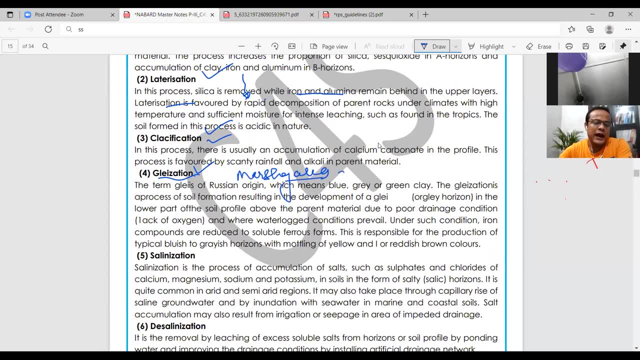 calcification is the formation of calcium. another important question: what is glagization? this is the case in marshy climate. marshy climate and this is in anaerobic condition, where there is a lack of oxygen. in the marshy areas generally, oxygen is less. 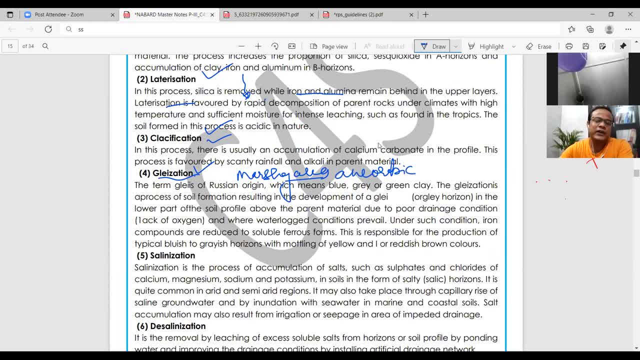 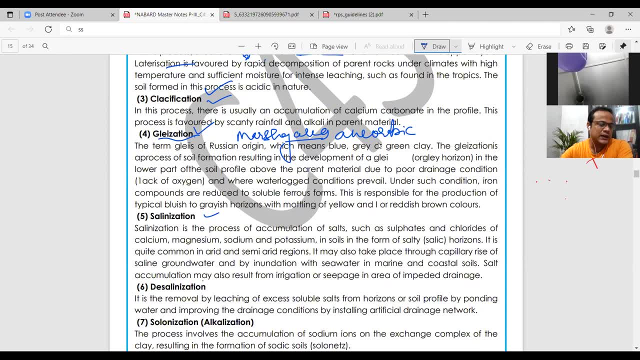 So the color of the soil changes there. that is very important. We will deal with soil coloration in the future. Salinization and desalinization are just opposite of each other, as the name only indicates. These are some specific soil formations. just look at their definitions once. 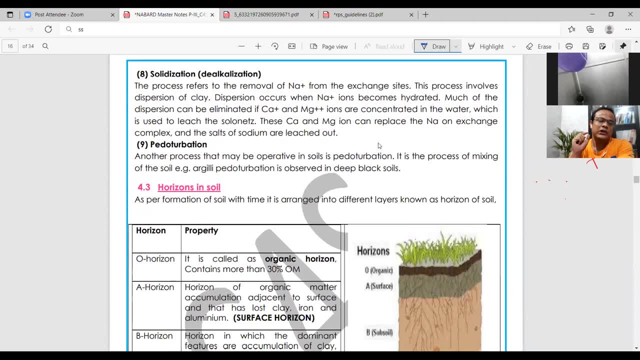 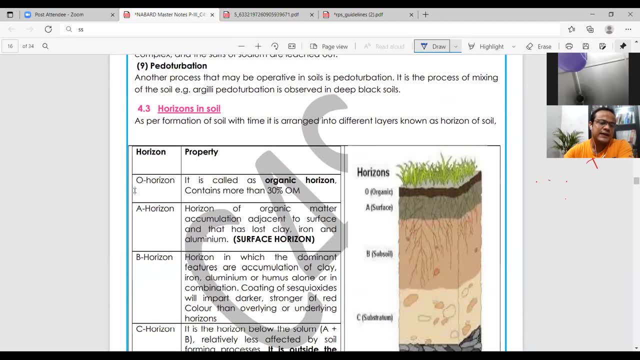 Try to understand what the process is. you don't need to look into it in detail, As Rohit was asking the horizon of soil, it comes now The top of the horizon, as the name only indicates: O horizon, it is organic. 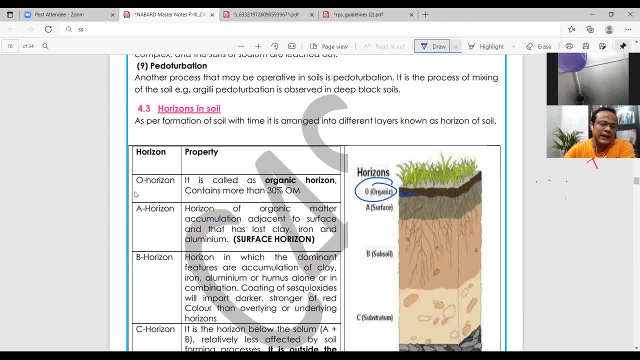 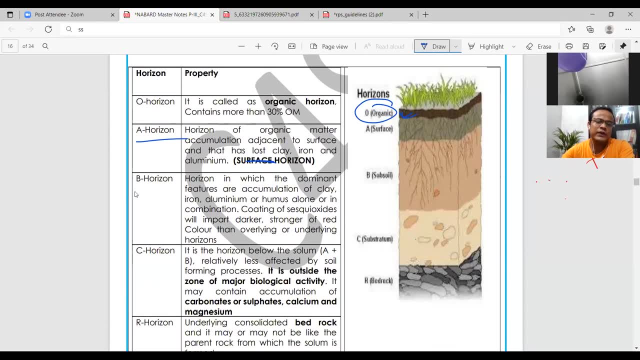 Most of the organic content will come here. After this comes A horizon below it, which we also call surface horizon. After surface horizon, it is B horizon, which you can see, C horizon and lastly is the parent rock layer. You don't need to see much in this. 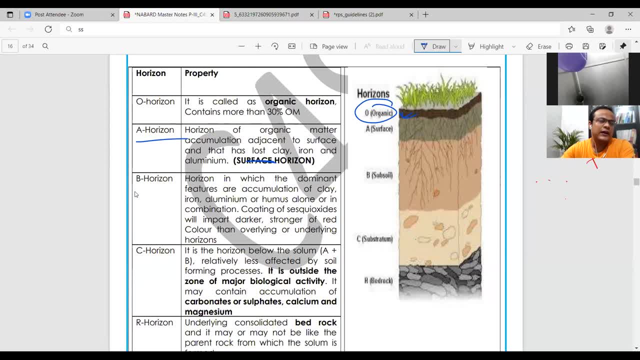 Just the first two layers. generally the question is asked from this, Which is the organic layer, O, A, B, C. So you can know by name What is the surface horizon, The A layer that you can see here, that we call it as surface horizon. 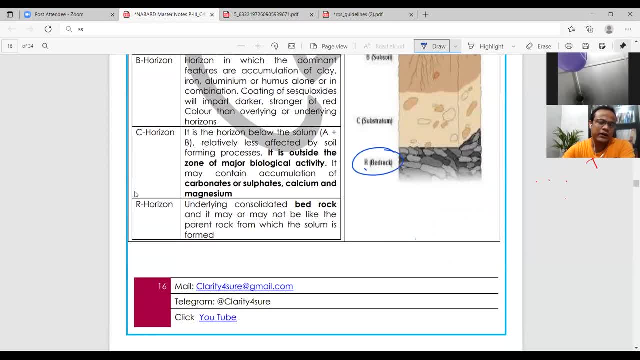 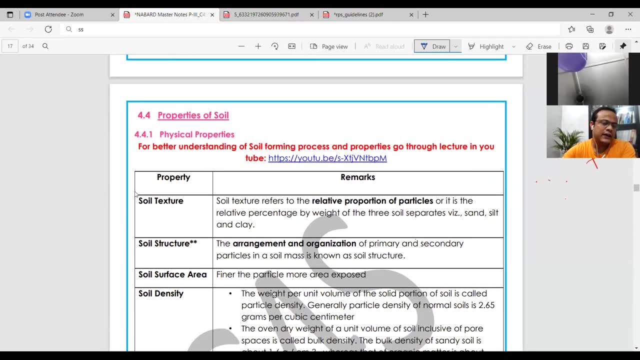 You just have to remember this. R horizon is the last layer, it is bedrock. We also call it bedrock horizon. Now, coming on to the properties of soil, Where does the question come from? They ask the question, basically the difference between texture and structure. 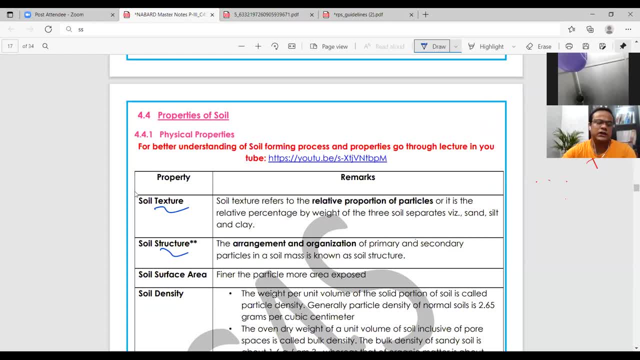 You may find it easy now: what is texture, what is structure? But when the question will come in the examination it will become difficult for you. In that situation you can make a wrong mark. So remember one simple thing: Whatever the term is in- both texture or structure- you have to place A in it. 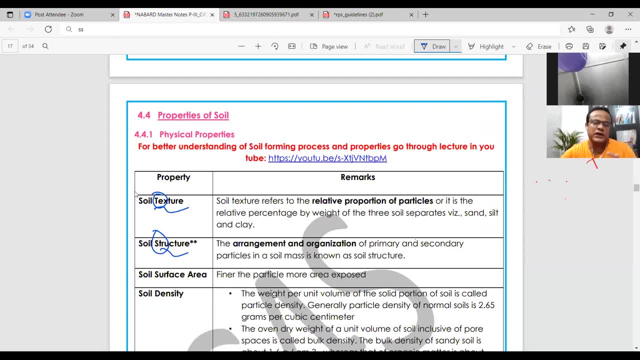 You need to place the word A where A fits, the answer will be the same. So A I mean arrangement S T. if you put A here, it becomes Saturday S A T. So remember that structure deals with arrangement, whereas texture deals with relative proportion. 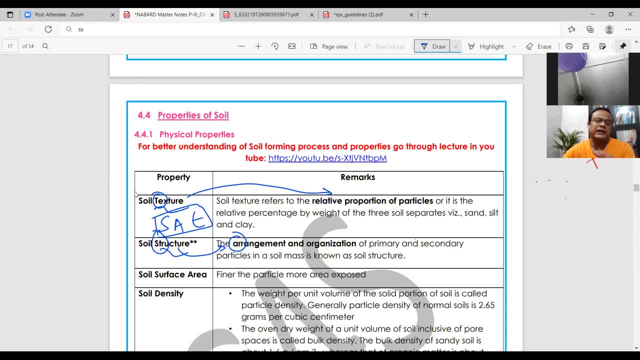 So, if the definition is asked, what is the relative proportion of particles in the soil, is referred as What is soil structure, texture, density. If we talk about the proportion, it defines as soil texture- Very important- And if we talk about soil structure, it defines arrangement and organization of soil particles. 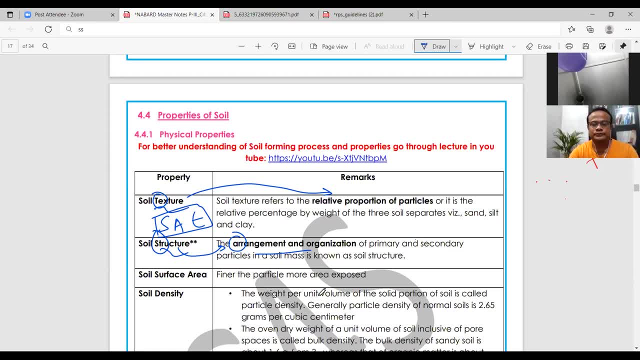 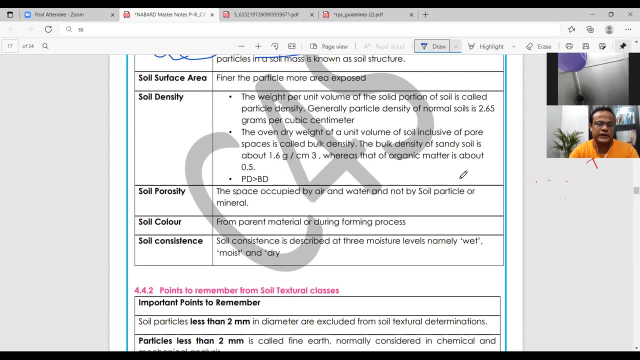 You have to remember this here, Right? Let's move on to the next thing: Soil density. We have seen this. Soil porosity, Soil color: Soil color is decided by your Munsell chart. We remove the soil color from the Munsell chart. 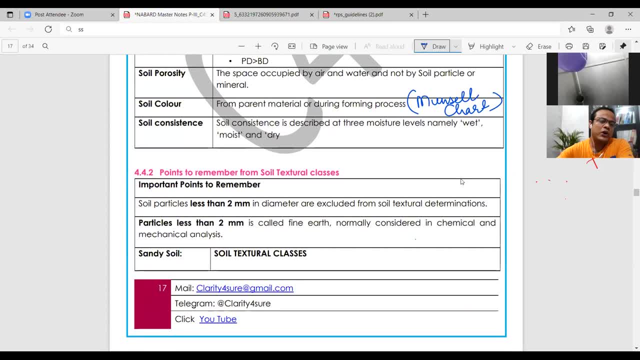 Remember this term at least. Okay, Now coming on to the points to remember, There are some important points related to soil texture. Here the question related to size is asked. We ignore the size from 2 mm. We do not consider those size. 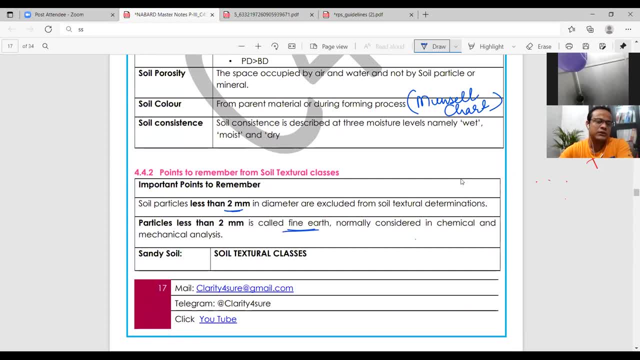 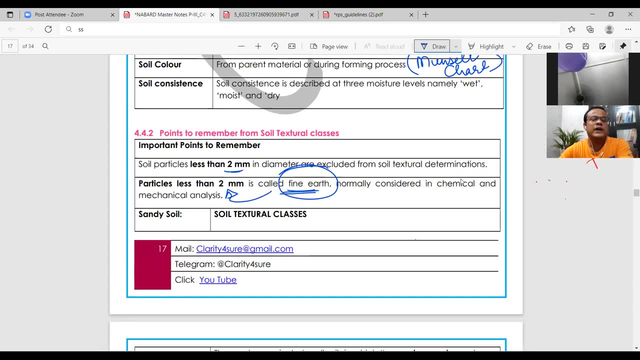 So particle less than 2 mm is called fine earth. This question is asked: How many particle size should be there in the definition of fine earth? So we consider the size less than 2 mm in the definition of fine earth. You have to remember this. 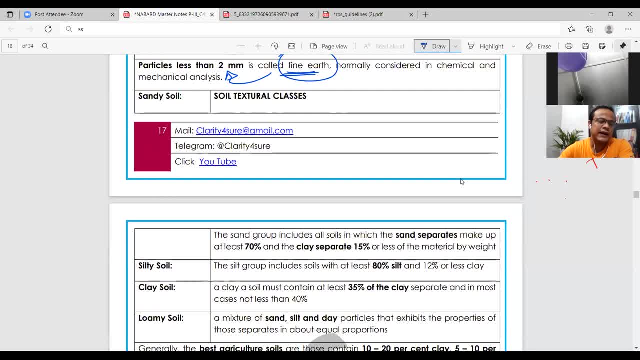 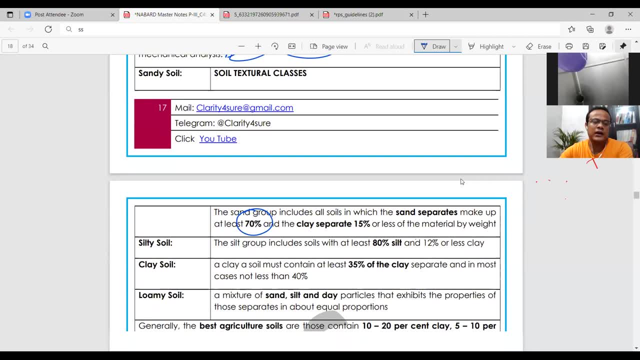 Next, Sandy soil. Compositions are asked in that How many percent sand should be separated in the sandy soil. So it is sandy soil. That means 70%, which will be basic will be sand. If we talk about silt, then what will be basic? 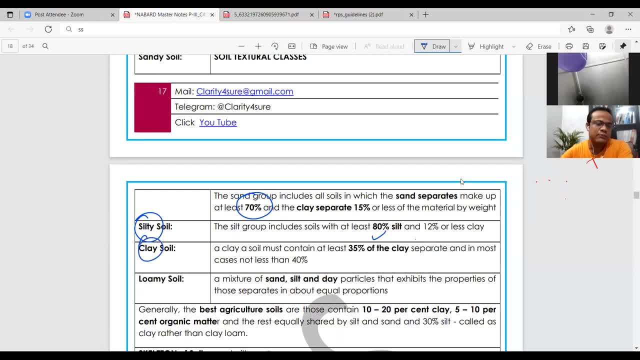 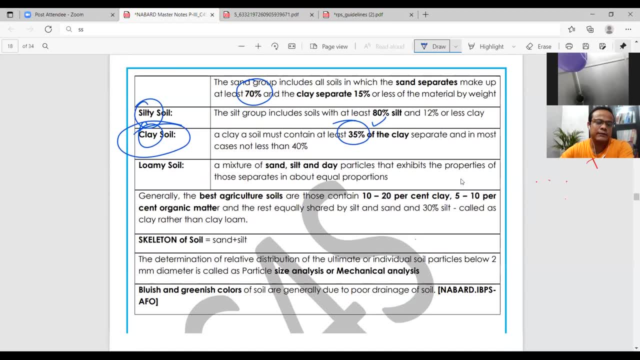 Maximum will be silt. If we talk about clay, then this is the most important soil. That is, 35% will be clay in the clay soil. You have to keep this important. That is Most important. Okay, Skeleton of soil. 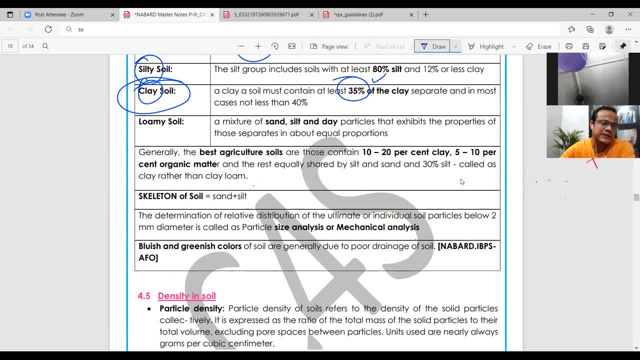 Who knows this? Sand, silt, Don't mix up. clay in this Skeleton is defined by only sand and silt, The clay that is outer covering as of your skin. Okay, Like your skin, clay is covering of soil. It is not skeleton of soil. 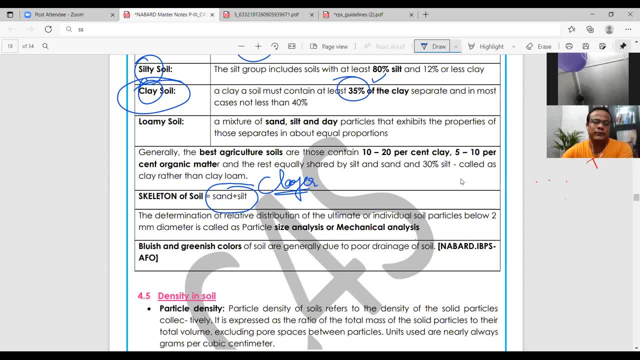 The skeleton of soil is only sand and silt. You have to remember this. Now. bluish and greenish color of soil. As I told you, this happens due to anaerobic condition. We also call it glaiation. This question was asked in NABARD. 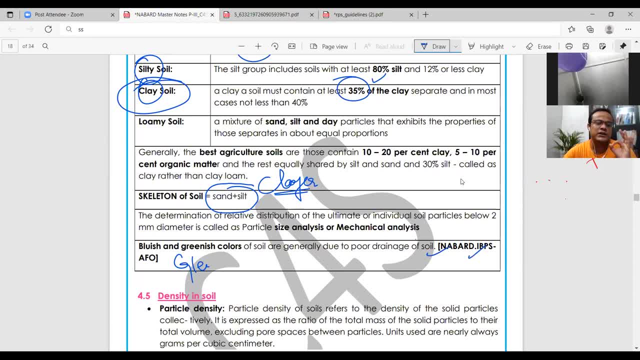 This question was also asked in IBPS AFO. So bluish and greenish color of soil are generated due to poor drainage or anaerobic condition. It happens due to anaerobic condition. Okay, Now coming on to two things. 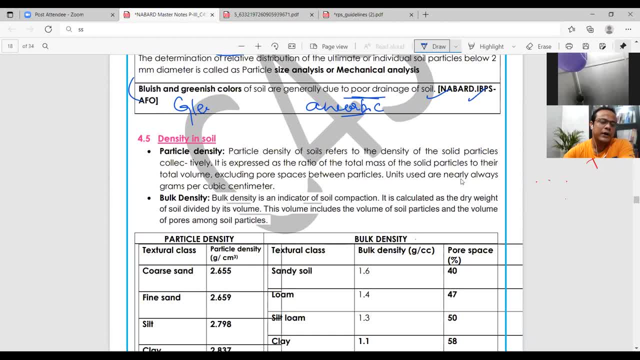 That is, particle density and bulk density. So always remember one thing: The value of particle density is more and the bulk density is less, Because what we are taking in bulk We take dry weight, Dry weight by volume. So what will be dry weight? 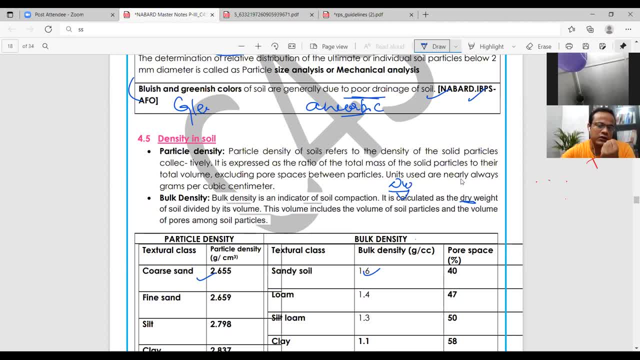 Whenever the weight will be dry, then what will happen there? Its quantity will decrease. Okay, So because of this, the value of bulk density is always more here, You remember this. But the value of particle density is more. When we talk about bulk due to pore space, it is very much. Due to excessive pore space, it does not get compactness. So what is its value? The value of bulk density is less. This range is also asked. So the range of particle density and bulk density, you must remember Its range varies from 2.65 to 2.83.. 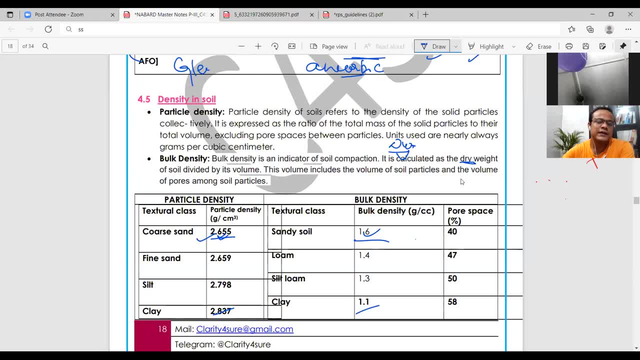 And its range varies from 1.6 to 1.1.. That is why I am telling you that this question has already been asked. They have already asked the question earlier, So remember the range of both. Which is bigger? Which is bigger? 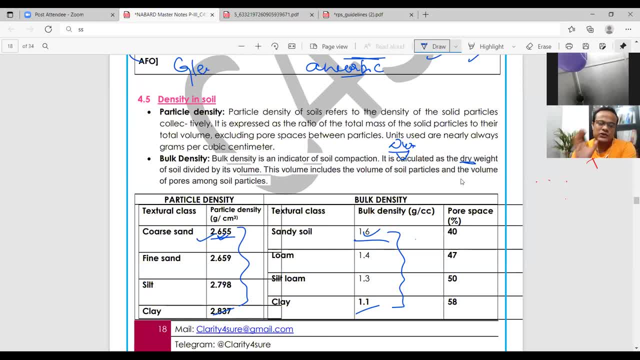 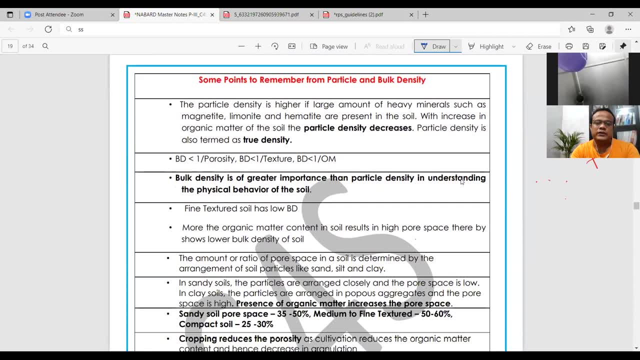 Particle density and bulk density And what are the ranges of both? You do not have to remember the specific. At least you need to remember the range of both the densities. These are some relationships. You can go through this. If there is organic matter, then which one will be more? 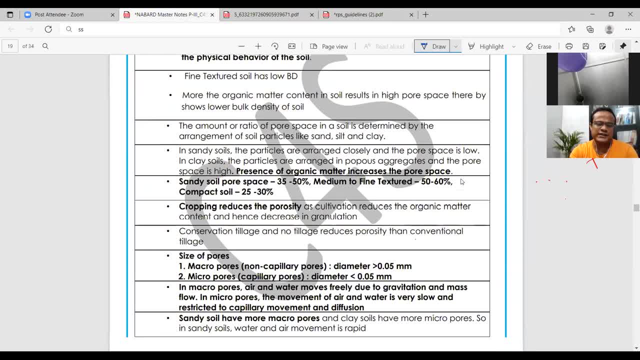 If there is bulk, then which one will be more. When there is more water, then which one will be more. If there is more water, then which density will be more. Read it a little Here. this is the most important. 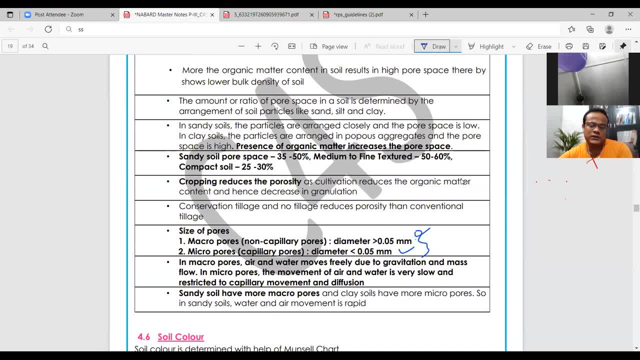 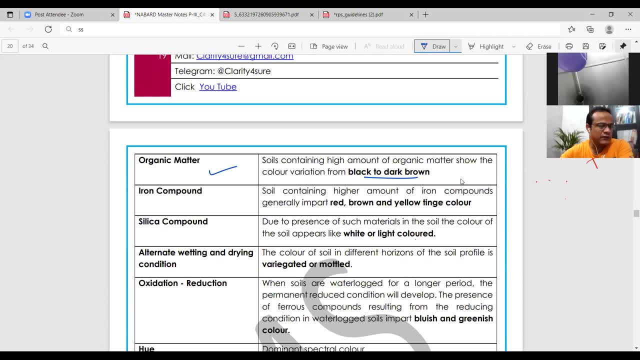 The size of macropores and micropores is asked. You can see these two. Okay, Soil color, which I was telling you is important. Whenever there is organic matter, the color of the soil will be black to brown. This is self-understood. 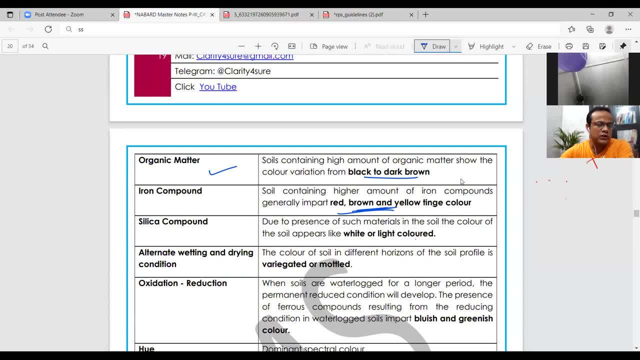 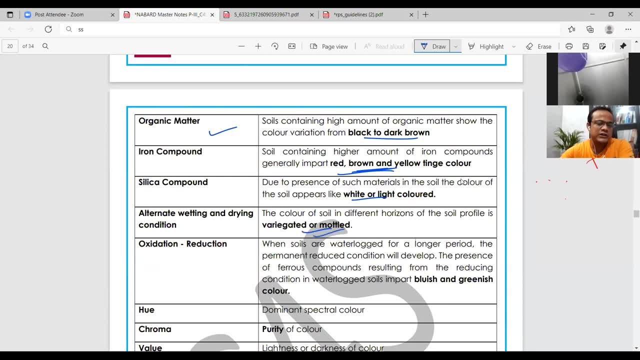 Whenever there is iron, then red, Reddish, brownish color comes in the soil. If there is silica, then silica. already you know It will be white. Okay, It will be light colored soil Alternate and wetting. We call it variegated or mottled soil. 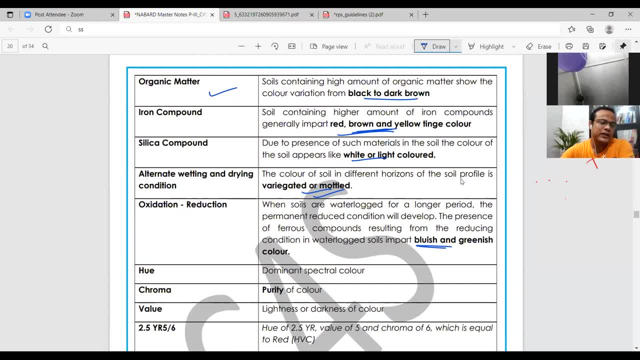 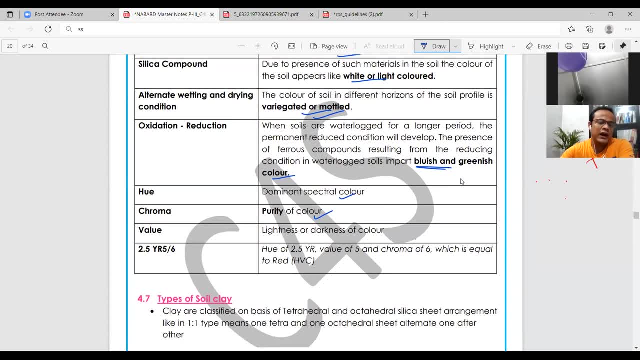 Oxidation reduction. Due to oxidation reduction, there is blueish and greenish color in the soil. Hue is the dominant spectral color. Okay, Chroma is the purity of the color And value is the lightness of the color. What is this? 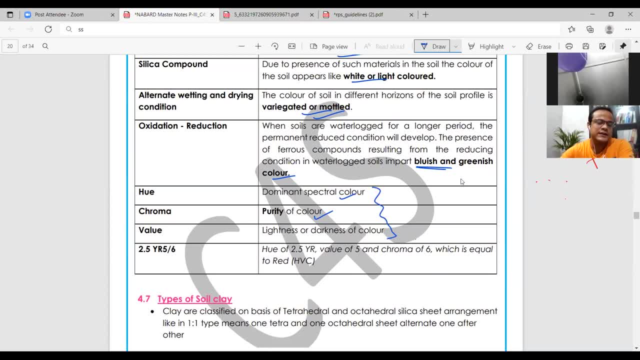 Huma, chroma and value. This is defined by the Mansell chart which we just discussed. If you are given this term that soil color is being represented by this, then you have to remember the first 2.5 yr: 1,, 2,, 3, the first three letters. it defines your hue. 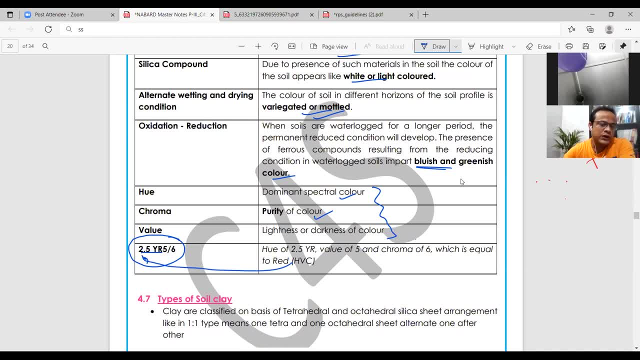 HVC. it defines your hue, The second term of 5, it defines your value And the last term defines your chroma. So these four things can be remembered by HVC code. First three defines your hue. The second last defines your value. 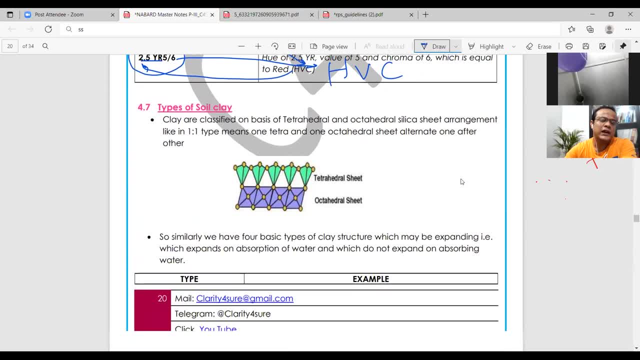 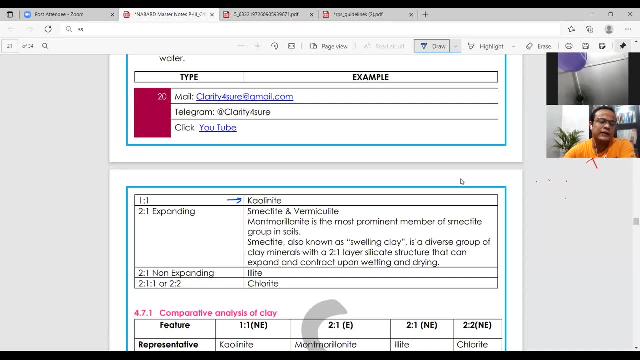 And the last defines your chroma. Now, types of soil clay. Look where do questions come from soil clay? I am telling you: Expanding, non-expanding type of clay. What is the example of? 1 is to 1, they ask. 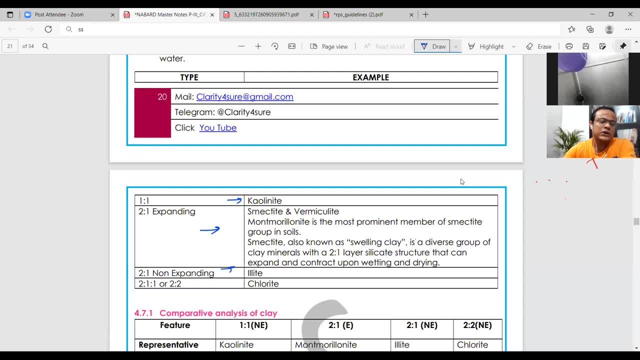 What is the example of 2 is to 1?? What is the example of 2 is to 1?? What is the example of 2 is to 1?? So expanding, non-expanding basis. you remember which clay is expanded and which is not? 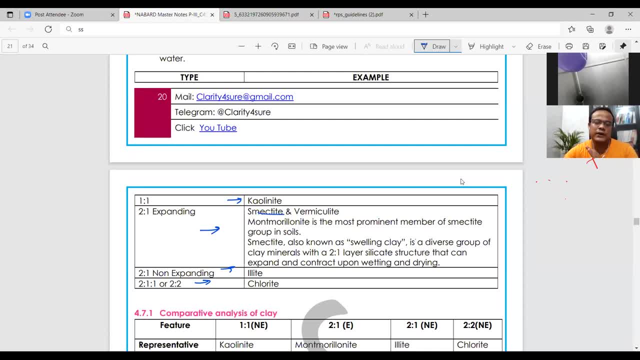 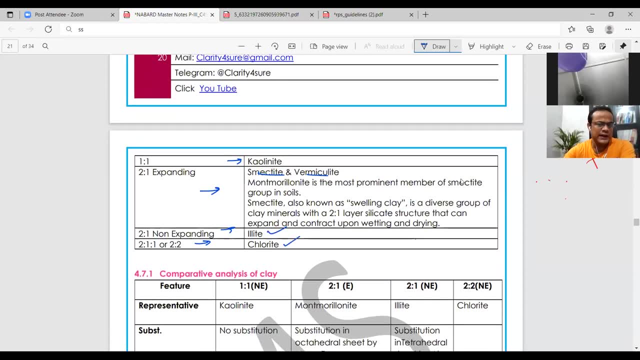 What is the example of 1 is to 1?? What is the example of 2 is to 1?? You remember Okay, from here, questions come generally. So it has elite. Best example is chloride. It has kaolinite. 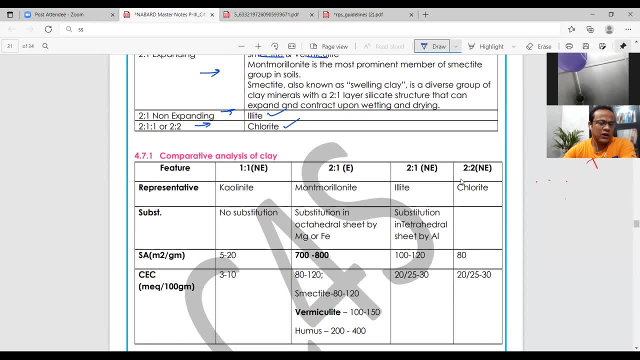 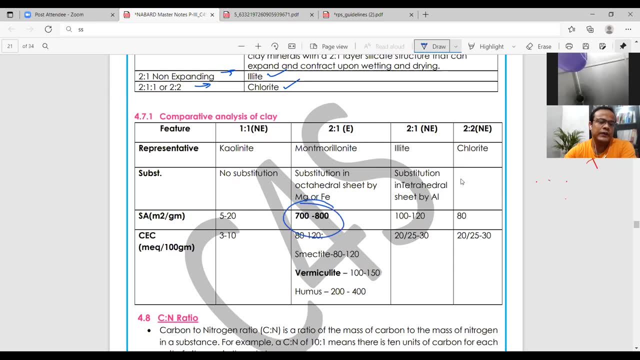 Spectrite and vermiculite comes inside. 2 is to 1 type of clay. Now the question is also asked from the surface area. a lot of times Now we have to see the maximum value, Which clay has the maximum surface area. 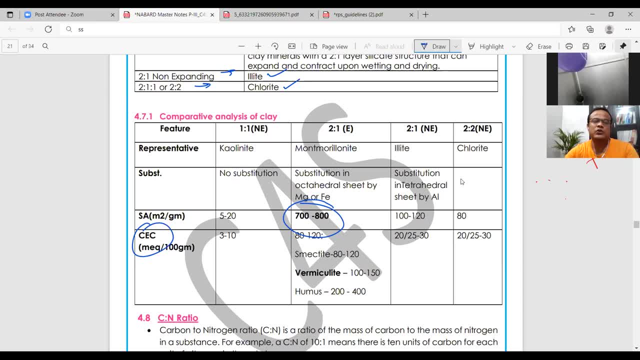 What is the maximum value of the cation exchange capacity? Just, you have to look upon the maximum values. Which type of clay is having maximum mass? Which type of clay is having maximum CEC? Leave the rest of the things. So, if you talk about the surface area, then see. Montemeterlite, which is clay, has the most surface area. If we talk about CEC, then see here: vermiculite, maybe No more than that humus. Humus does not come in clay, But it is given for comparison. 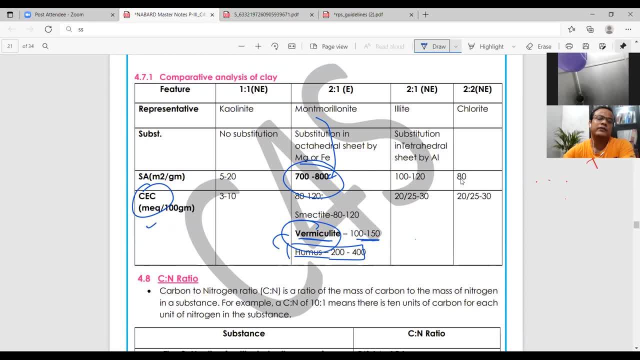 If we talk about clay, then vermiculite has maximum 100 to 150.. Just, you need to look upon the maximum ranges And example of each type. What is the example of 1 is to 1?? What is the example of 2 is to 1?? 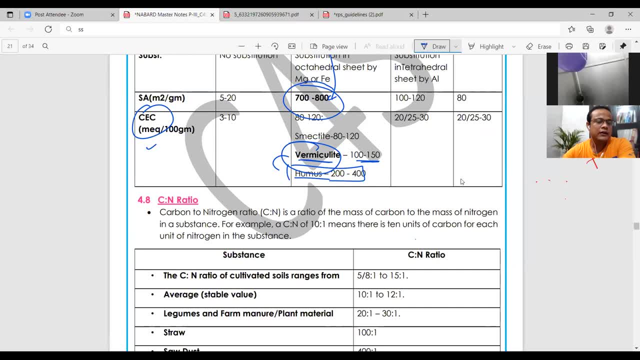 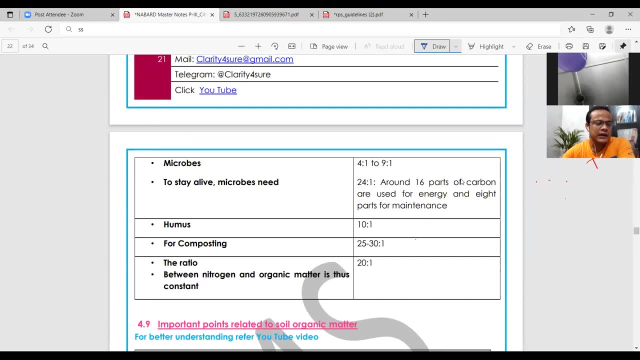 What is this And what is this? You have to see here C and N ratio, again important Carbon nitrogen ratio. So this is asked in examination: Carbon nitrogen ratio, Especially how much is of humus, How much is of compost. 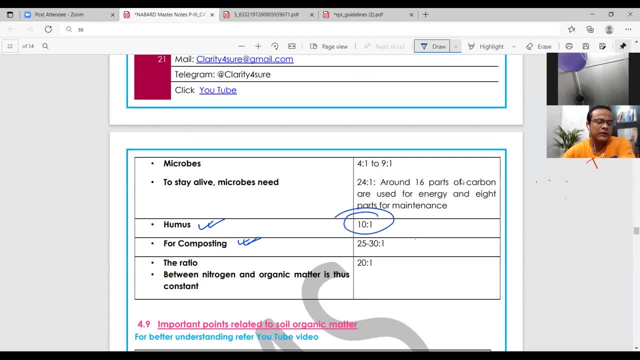 You have to remember this: 10 is to 1 is for humus And 25 is to 30 is to 1 is for compost, C and ratio. Why is it an example for compost? Because if C and ratio is not achieved, that is, 25 is to 30 is to 1,. 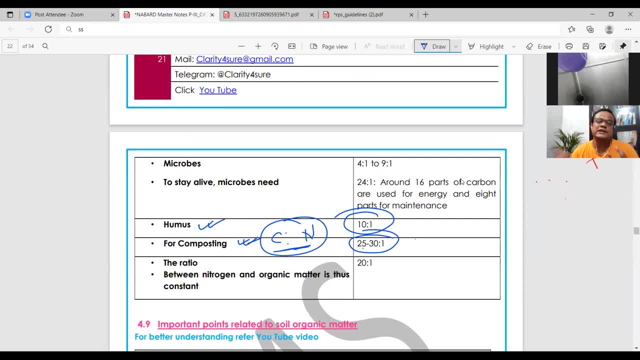 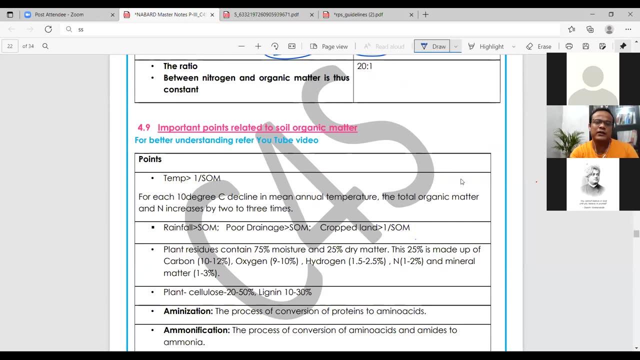 then compost making process will never be successful. That is why, when we study about compost, we always see that C and ratio should be in this range. Then only compost can be formed. That is why C and ratio is important. So I have given some important points. by summing up, 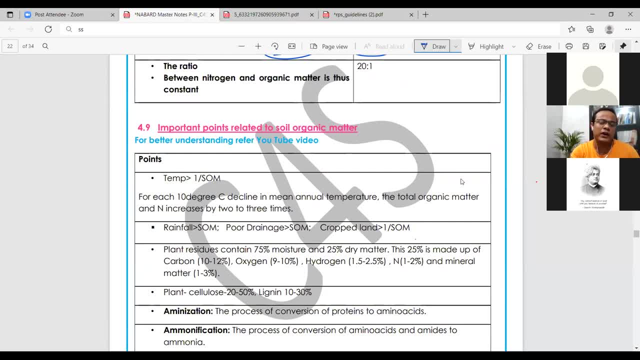 Related to organic matter. When will organic matter be more? When will it be less? What are the conditions? So you can see that once Very easy to remember. Now, coming on to the next topic. This is an important topic of soil science. 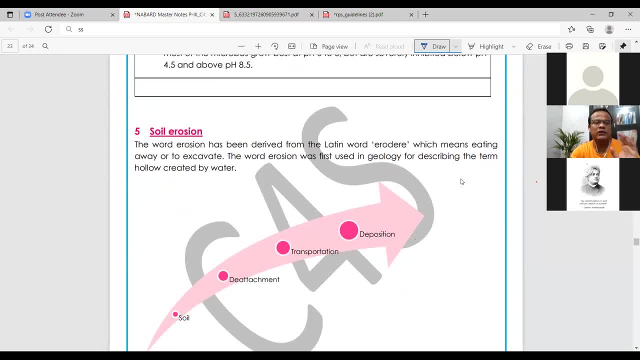 Soil fertility. I will discuss in a separate video Soil erosion: Basically, they have not asked a lot of questions till now. So now see this process. What happens after this? The question will come from here. Soil is done, Deattachment is done. 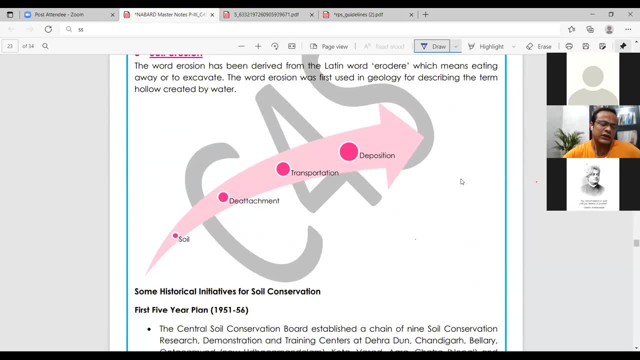 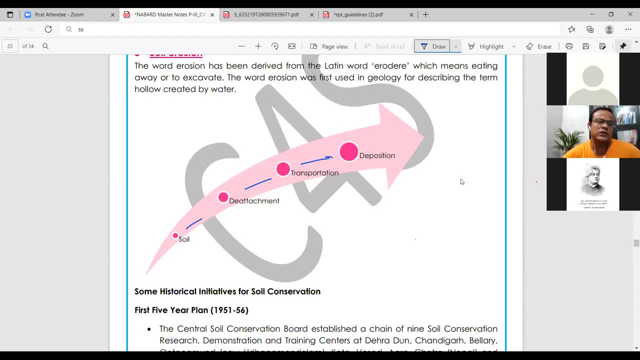 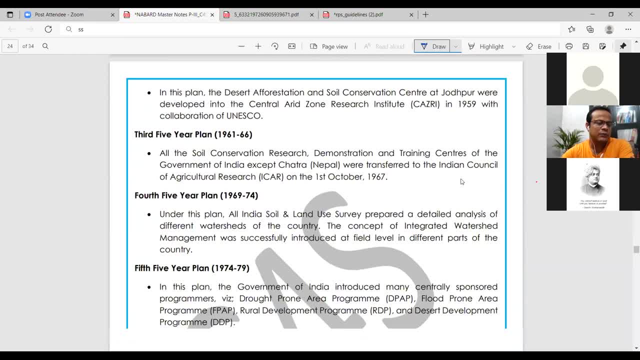 So it is not so important for the examination Now. types of soil erosion. Very easy to remember: Geologic: Wind and water. This is the soil's transportation Now in wind erosion. Again you can see the process. 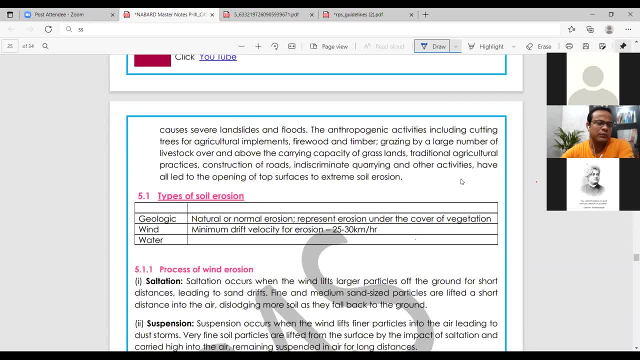 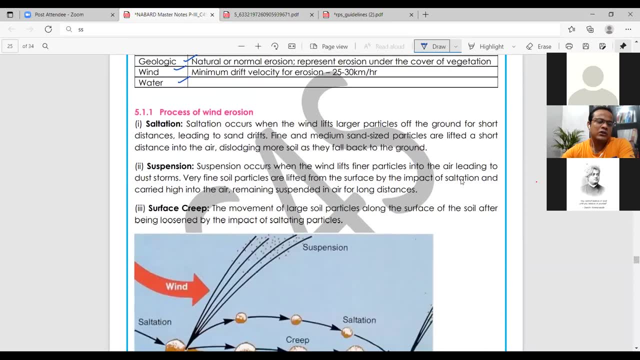 What we have seen in the soil, What happens in this: Saltation, Suspension And surface creep. So this is the process: Soil is done, Deattachment or transportation. Soil is done, Soil is done. Soil is done, Deattachment or transportation. 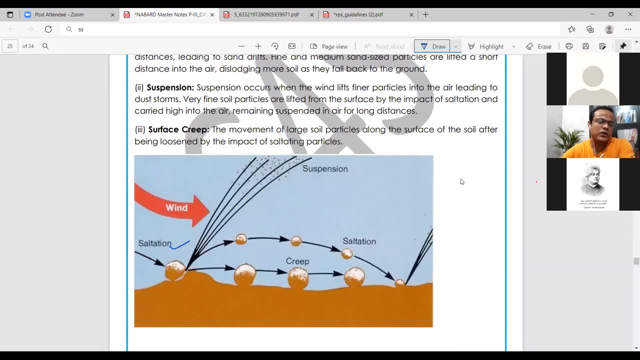 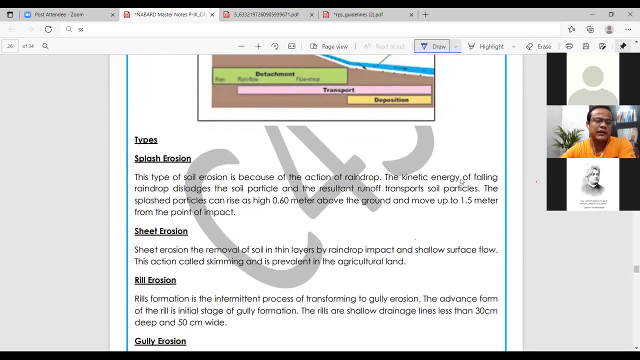 Soil is done. Soil is done and surface tape. So this is the process of wind erosion. When it comes to water erosion, you need to see the size. What is the size in this range? Splash erosion is the most initial form. 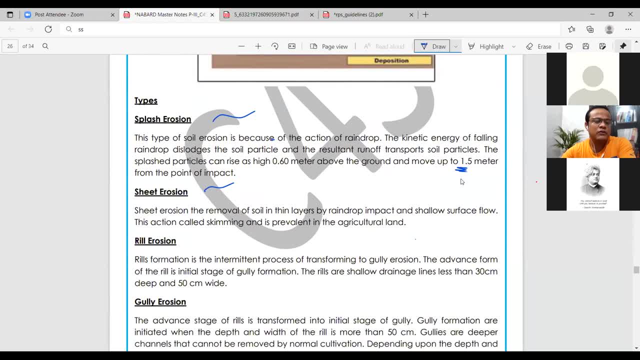 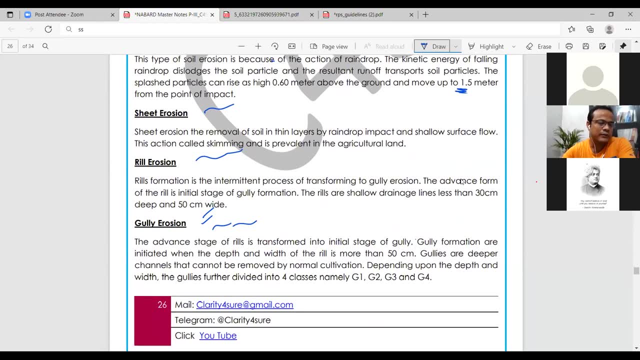 Then, when there is a little more, then it will be in sheet form, Then it will be in the form of rill, Actually Gully, which is the reason for Gwalior-Muraina, why is it the most common there? 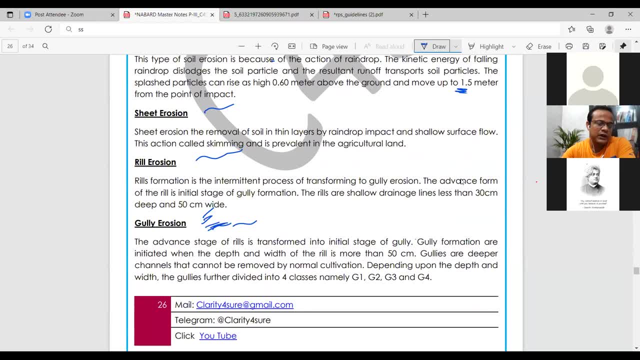 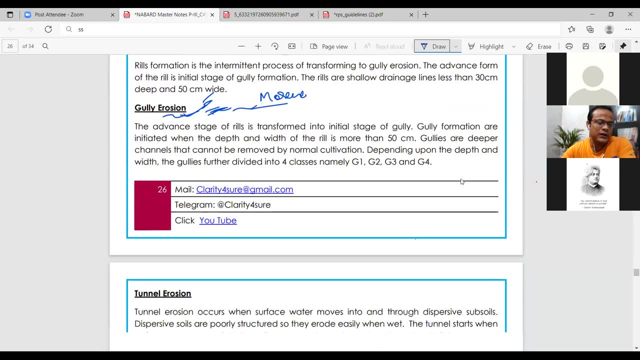 So there you will get Gully erosion. Gully erosion is the reason for Gwalior-Muraina, So Gully erosion is the most common. After that another form comes, that is Tunnel erosion. So mostly Gully erosion stops. 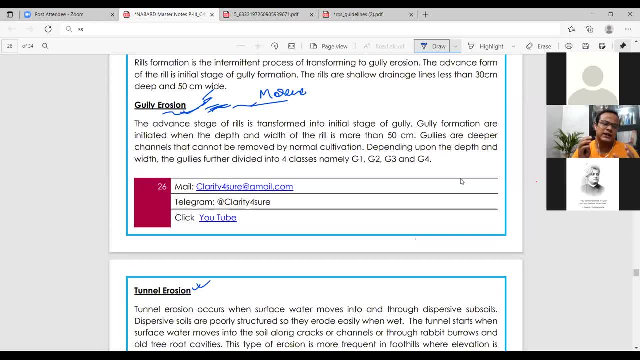 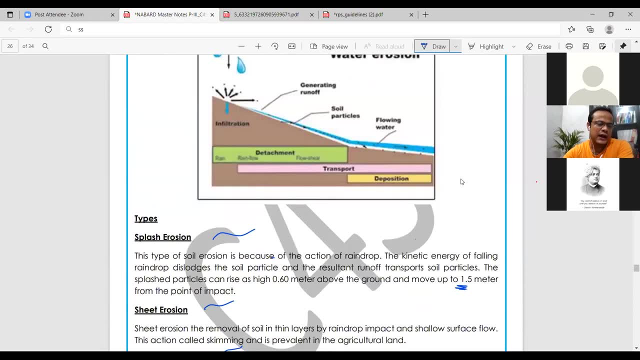 Tunnel formations generally do not occur. So Gully erosion is the most extensive form of water erosion. You have to remember this. The most harsh form is: what is it? Where does it start from? You have to remember that It starts from splash and it goes up to tunnel. 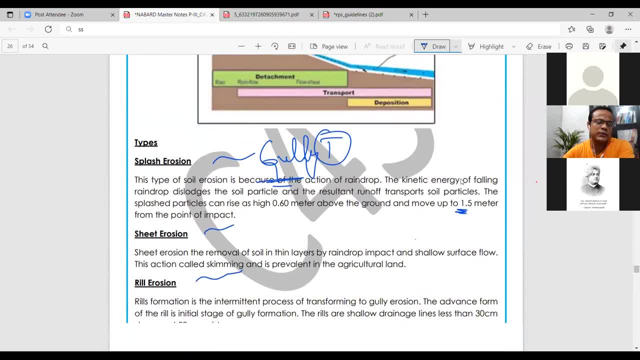 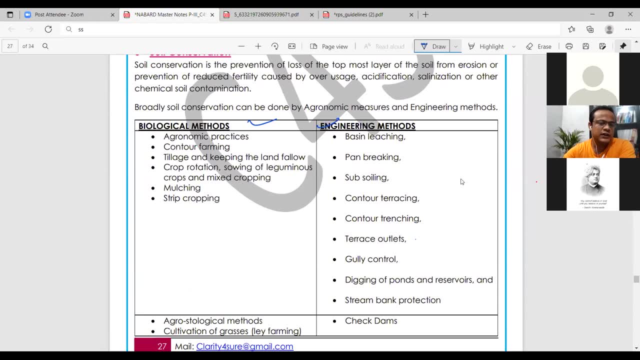 But mostly we see that Gully formations occur. Thank you. If we talk about soil conservation, then what are the basic biological methods? What is the engineering method By mixing up? a question can be given from here. For example, five methods have been given. 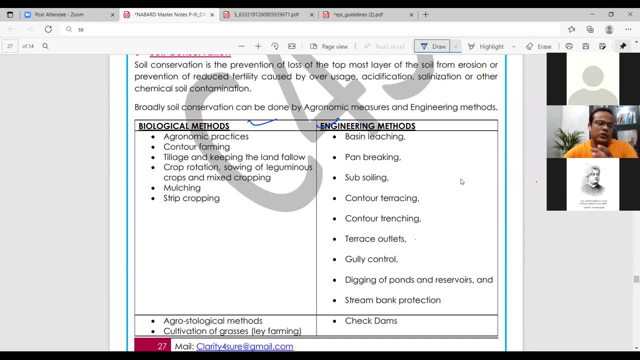 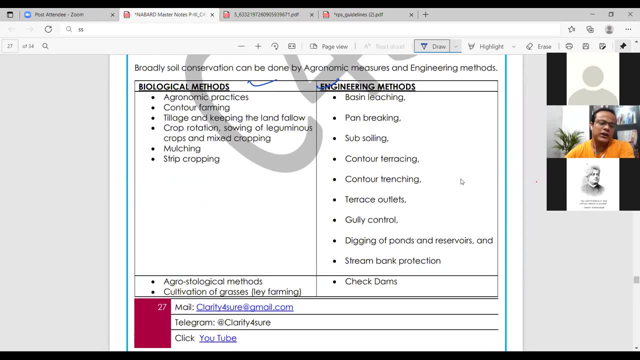 One is mixed up, One biological has been put in the middle, And all the four options are engineering. So they can ask which of the following is not an engineering method of soil conservation? You have to remember this. One term is important here. 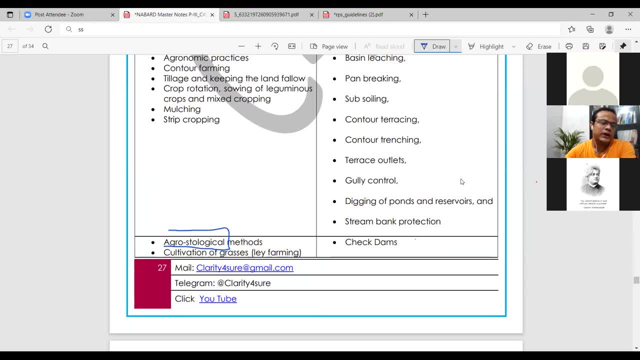 That is agro-strological. What are agro-strological methods? If somebody can comment, what does this term strological mean? Very important. What is agro-strological methods of soil conservation? What is this strological? 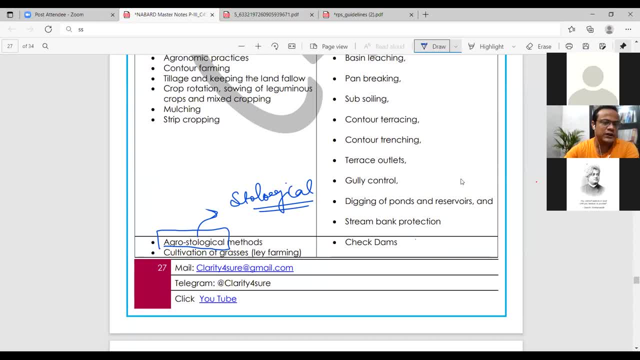 What is this strological Study of grass? Very good, Akshay. So when we do grassing in that area- Suppose we have grown agriculture crops Where there are barren lands, we are growing the grass. So the growth of the grass is called strological. 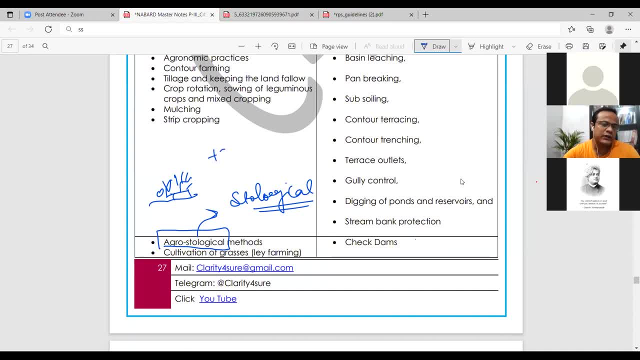 So agro-strological is growing of agriculture, crops along with grasses. So these kinds of questions come up. We relate it with the integrated farming system and ask: So agro-strological method is important. That is related to your grasses. 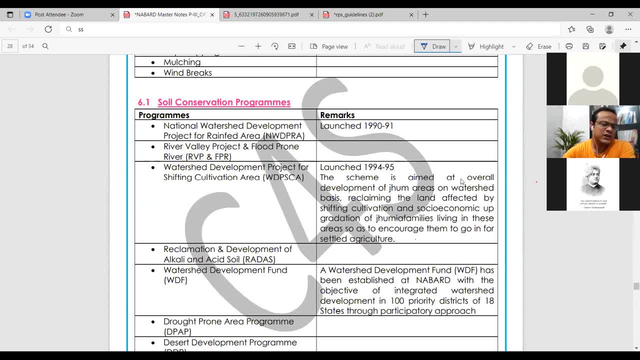 You can see this: Soil conservation programs are not so important Because we have discussed this in the watershed, All the recent things. So, IWMP, Where have we reached from there? We have reached WDC, IWMP 2009.. 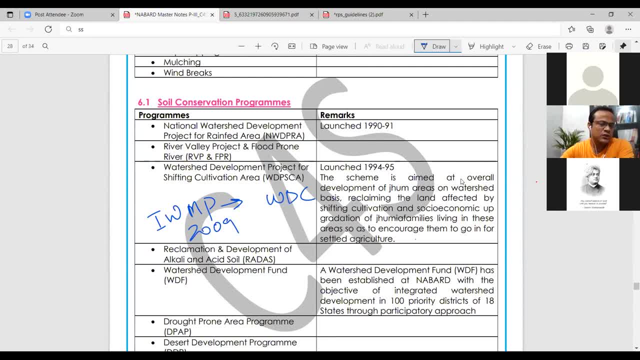 And when PM KSY came in 2015.. So this becomes its component. Okay, So what questions come from here? You already know What is the financial assistance given for watershed development. How much is it Revision Already? I have told you earlier also. 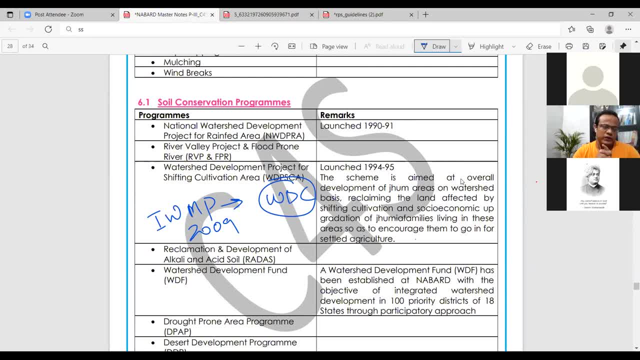 In the watershed development program under PM KSY? What is the financial assistance given per hectare for development of watershed In hilly areas and in normal areas? What funds are given per hectare? I have already told you this. I have given this in the first lecture. 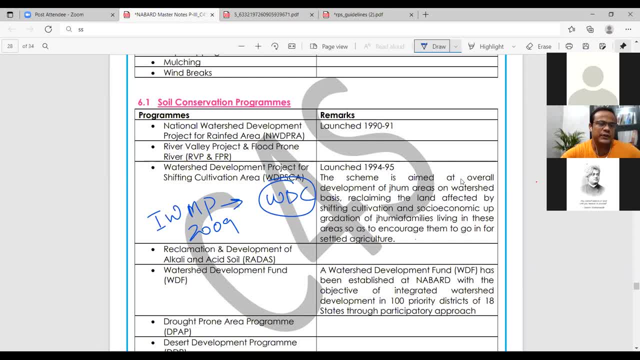 So I am telling you again: Please, please, please, Read it well, Revise it, Don't forget this point. I have given this question in the 10 at 10 quiz also. So it is 15,000 per hectare for watershed. 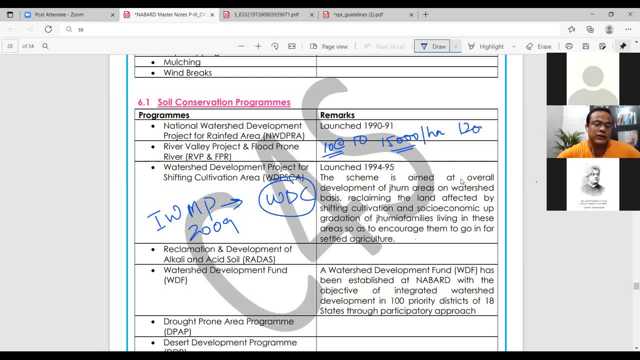 In general areas, In hilly areas, In general areas, it is 12,000 per hectare. Remember this. This is the financial assistance given for watershed development. And one more thing I remembered from watershed, Very important. I think this question has come up for a year. 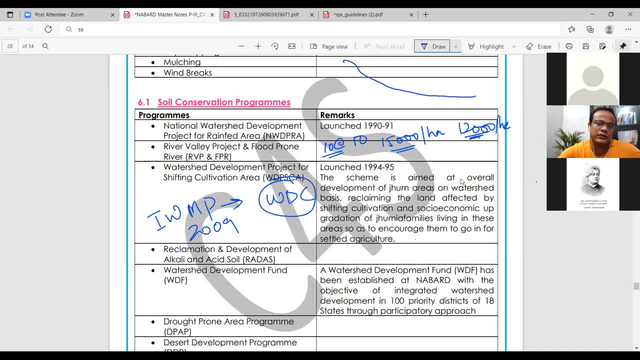 When we study watershed, You know that watershed, what it is, All the drain offs happening here. All the water is in one place. Here water is deposited. So by the water being deposited It becomes a water table. All right, The water table formation has happened. 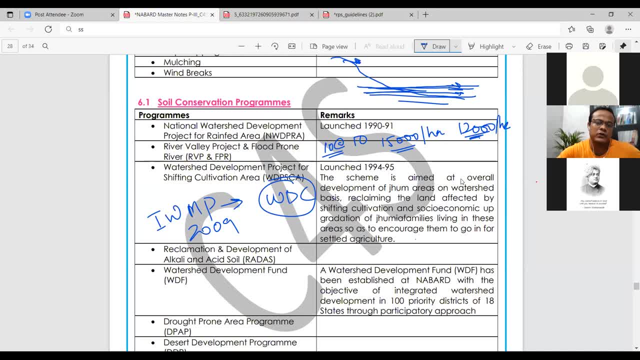 This is a hydrological source. The discharge is coming from here. See, the question has come from here. That is why I am discussing. So from here, you understand. This is the water table. From here water is flowing and coming. 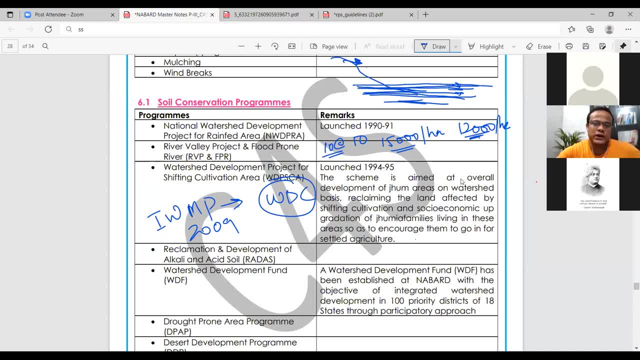 So where the accumulation of permanent water happens, This area Where water will always be in the ground, All right, This is called saturation. What happens? So here is the water, So here is the water, This is the water. 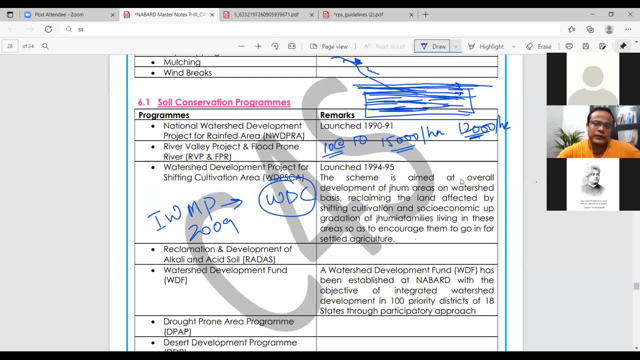 What happens? Here is the water. Here is the water. Here is the water. This is called saturation area: Saturation area Where the water is flowing, Because here the water is flowing. the water will not be always available over this part. 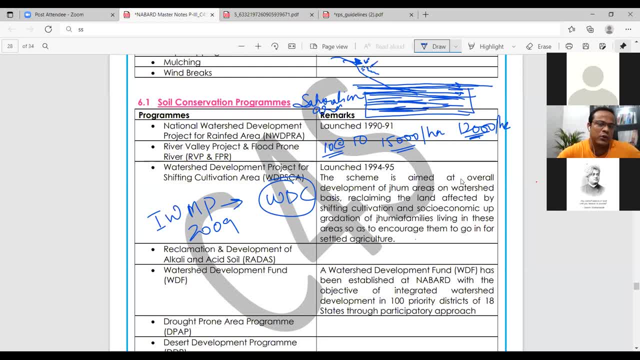 So some part will be aerated, Some part will be aerated, Some part will be moistened. So we call this area as aeration area Or zone of aeration and zone of saturation. So water table, that is ground water. 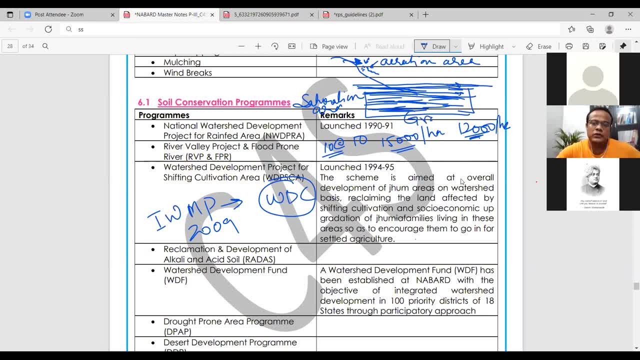 that comes in zone of saturation. Remember that, The ground water that comes in this saturation zone And the question that was asked. from here I am telling you that the ground water zone, the saturation area where there is a point where, again and again, 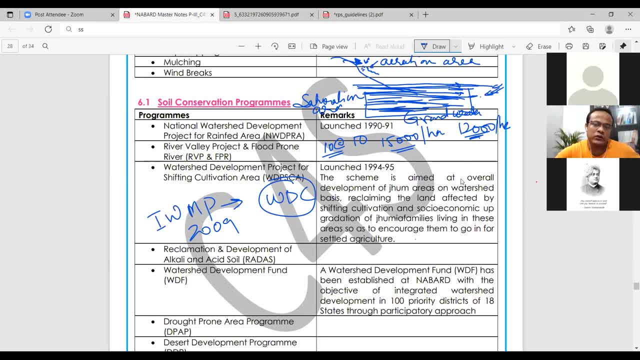 water is coming from somewhere, Recharge is automatic, So we call this area as aquifer. This was asked in the examination. What are aquifers? Definition was given From here. this question was taken. That is, watershed development. When you will read the zones of watershed development. 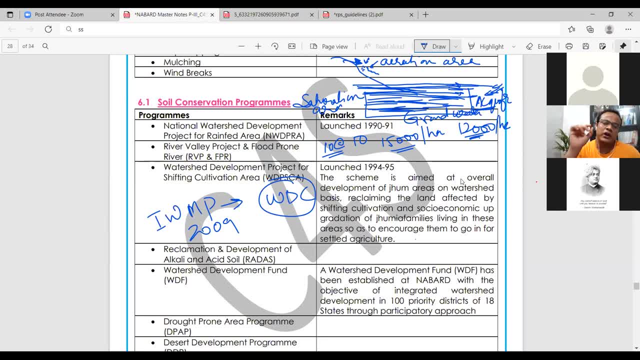 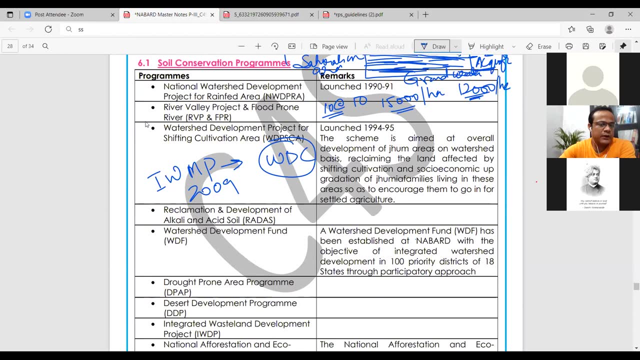 as I told you, saturation zone. We know saturation zone by another name, that is re-hetic zone. That is re-hetic zone also we know by the name of re-hetic zone. Okay, You have to remember this. I told you about WDC. 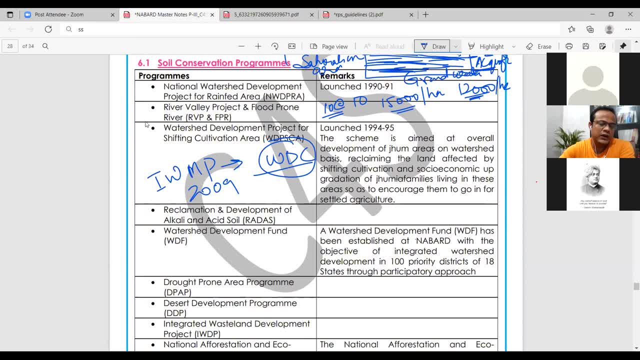 One more thing: that the whole project of WDC one is to develop a watershed, One village. you need to develop one watershed. So what is the time period given? What is the time period given by the government for this, For developing the watershed? 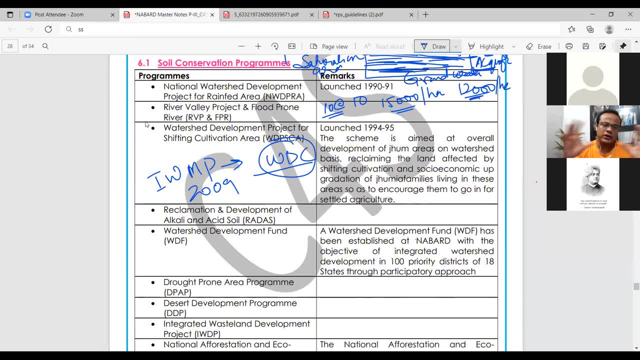 What is the time period giving government is giving for developing a watershed in an area? How many years, Please? what is the time frame? Four to seven years. Four to seven years, Remember this is given- In which there are phases. 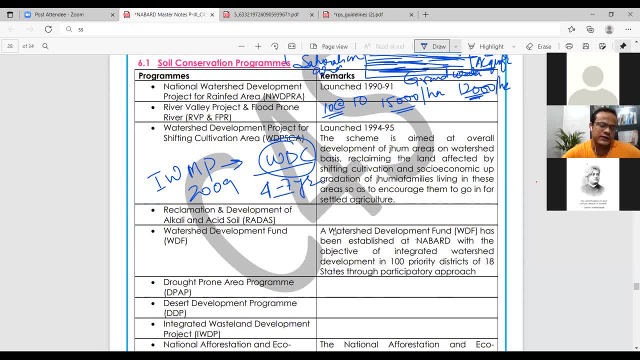 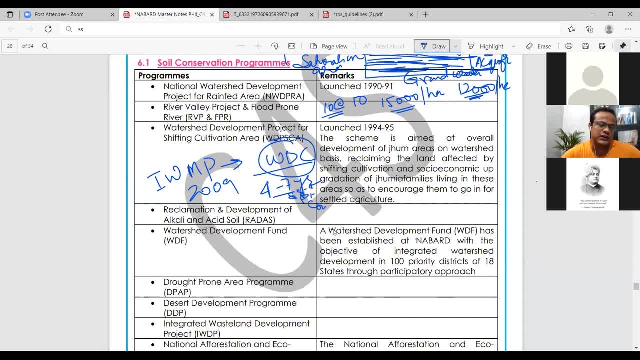 Then there is a consolidation phase. So there are three to four years, one to two years. these types are there. You can see that overall is more important. Four to seven years is given. So the important questions from WDC. I have told you about the watershed. 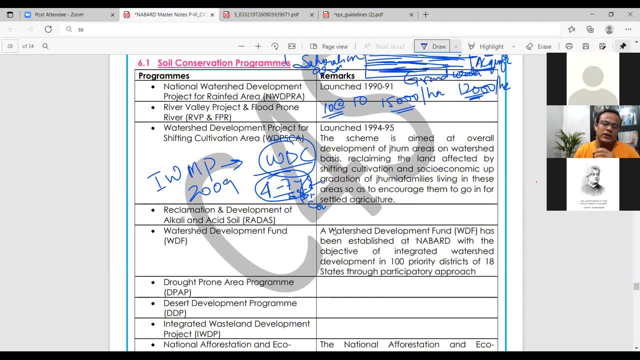 There are other things that I have already discussed in the first lecture. So you can see that there is a Nilanchan project, there is a World Bank assisted project. In how many states are we implementing the Nilanchan project? How many states are we implementing the Nilanchan project? 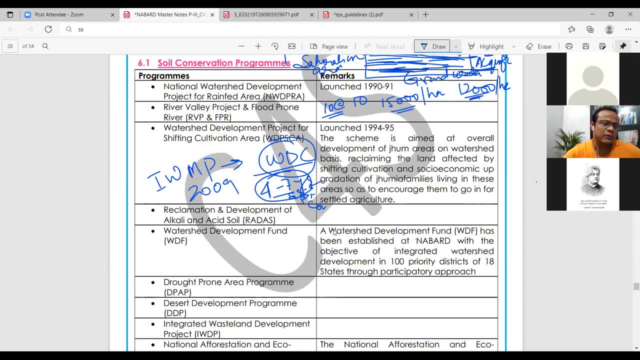 related to watershed development. In how many states are we implementing the Nilanchan project? In how many states are we implementing the Nilanchan project With the help of World Bank? Nilanchan project: nine states. So WDCC is the area from where the questions will be asked. 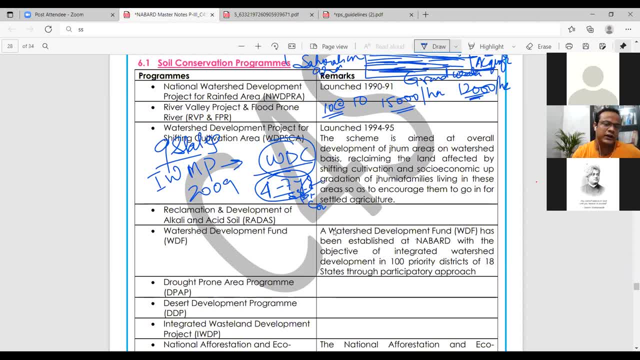 First is assistance. I have told you that there is a point of 15,000 and 12,000 assistance. Next, I told you that these zones are important. How did the question come from here in one year? I also explained that to you. 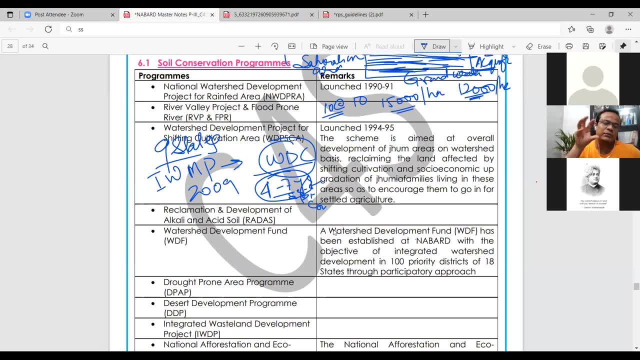 And lastly, four to seven years is given by the government to develop WDC in one area. This is important. There are some old points. if you leave them, it will be fine, Not important. all the DPAP and all those things. 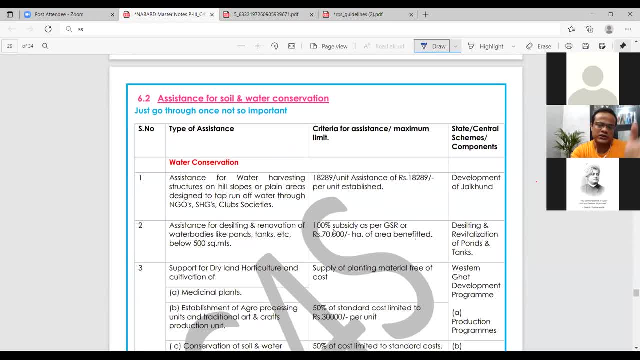 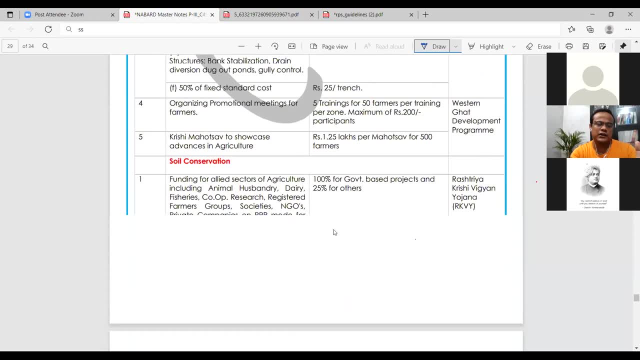 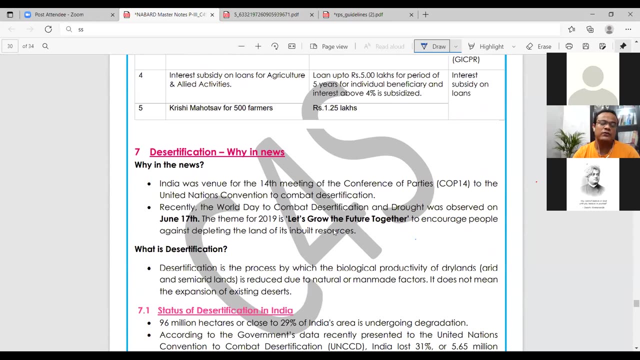 You can leave this. You can leave this as well. This adjustment information was given for the purpose that how much assistance is required in water conservation, Not required for your examination. You can skip this chart Now, moving on to desertification, because you know that the venue related to desertification. 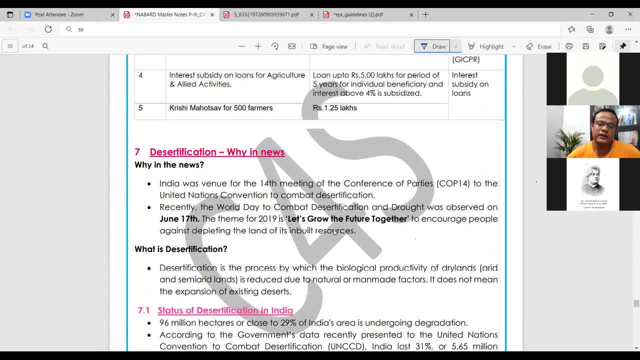 for the 10th COP was in India. That's why we have taken this question. and erosion is you know, because you know that the venue related to desertification was in India. Erosion is part of your syllabus. You have to remember what its motto was and all these things. 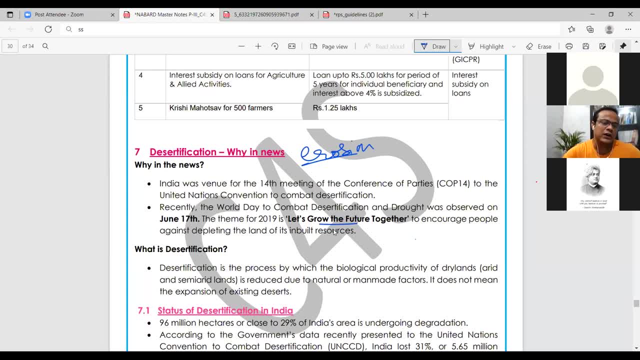 You have to see what the venue was. What was the venue of this COP? Where was the venue of COP 14 in India? What was the venue of COP 14? New Delhi or Noida? Noida, It is in Noida. 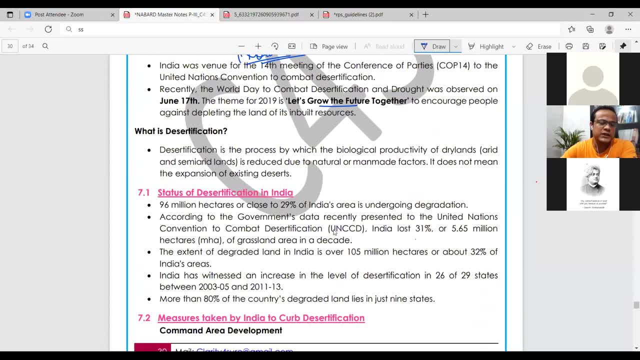 You have to see where it is. It is in Noida, I think it is written in Noida. So you have to see the status of desertification. And what are the promises made by the Prime Minister? How much? 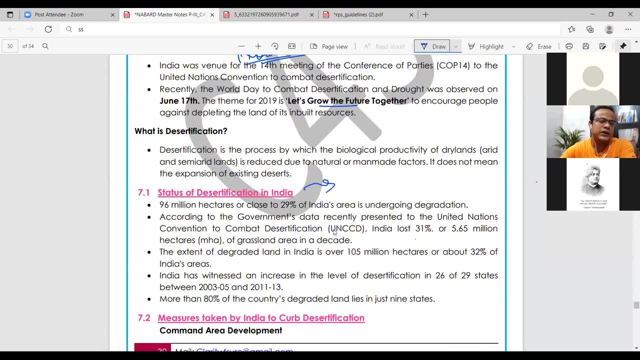 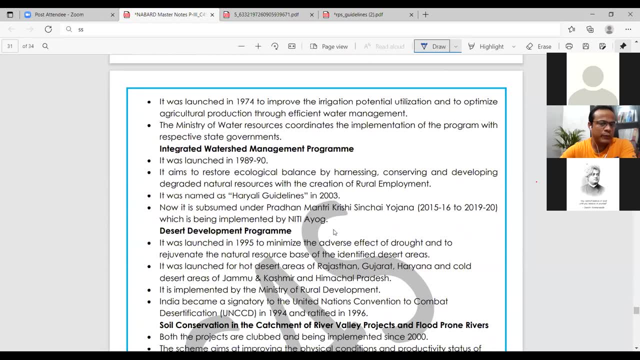 How many years How much land will be taken out of degradation? You have to see that target That is important for this year. Measures to curb desertification. So I will not discuss command area development right now because in the first lecture I have already discussed. 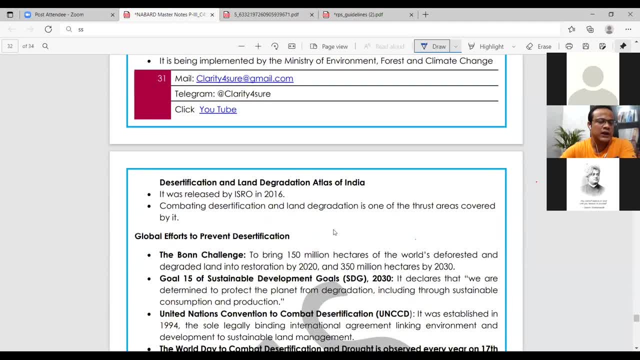 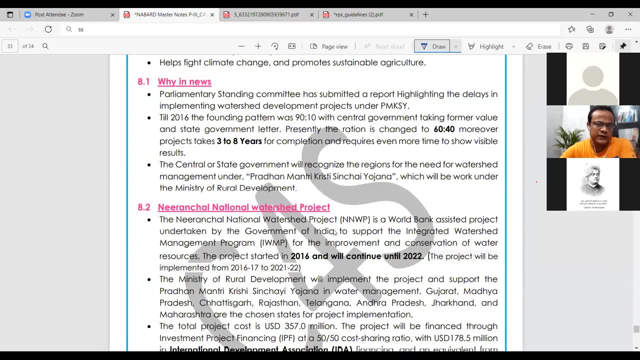 about watershed in detail. Okay, I have just told you a little bit about what I had not done. The area of the water zone, Watershed, watershed. Look, there are three to seven years, Three to eight. Both are written. 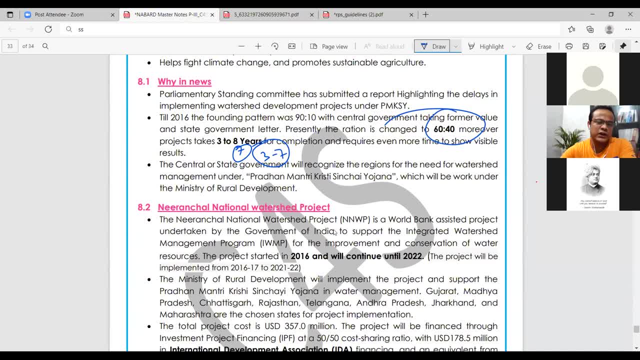 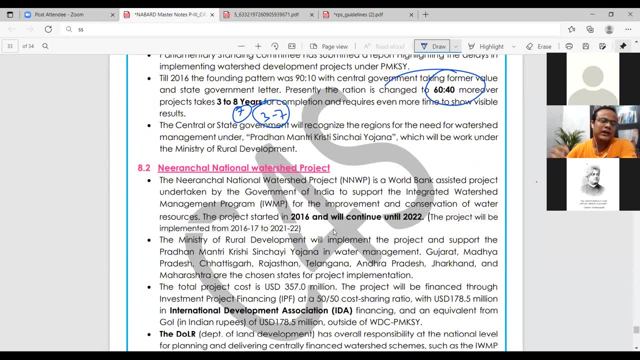 Three to eight. Three to seven. This is the general range: 60 to 40.. Okay, You have to see this, Akshay Singh: 26 million hectare by 2030.. Okay, Good, We will change the degraded land. 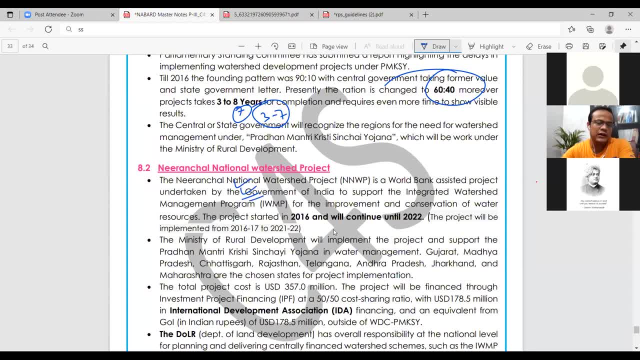 Good land. Okay, The Ranchal project that was discussing- You have to see this a little bit- Who is implementing about this? Where is it being implemented? So this one part is over. That is soil Science related And there were some small topics. 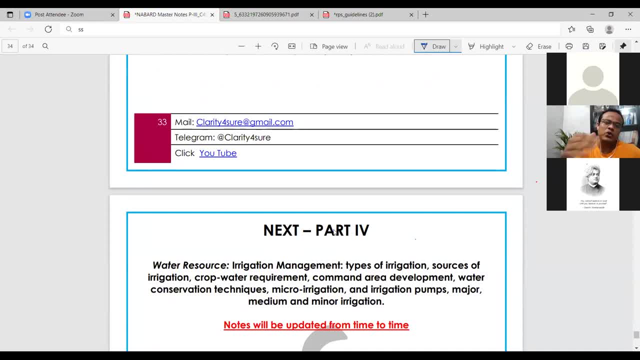 Now the more important topic is soil fertility. is more important What we will discuss right now: Soil fertility, So there is a presence. Soil fertility, Soil fertility. So there is a presence, So there is a presence, So there is a presence. 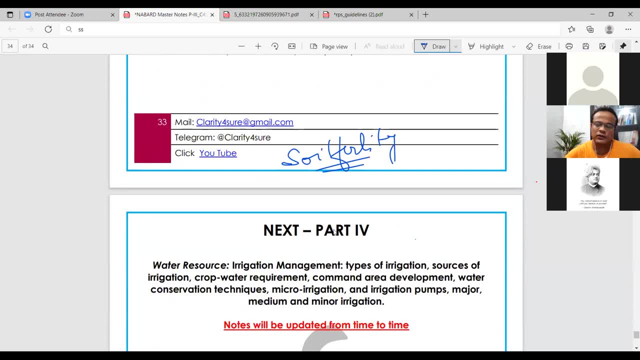 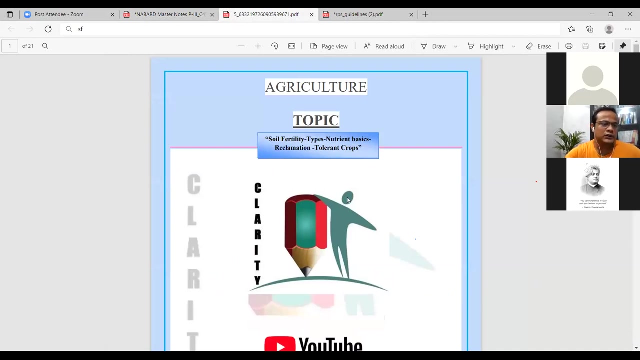 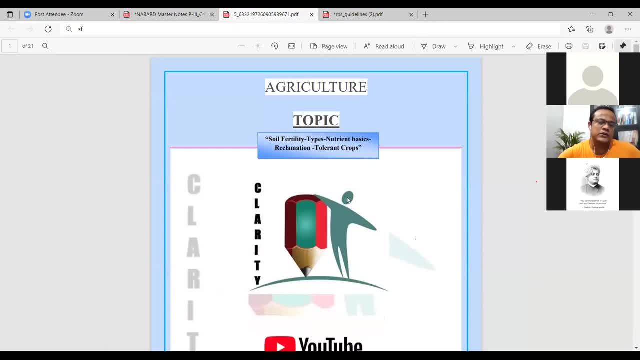 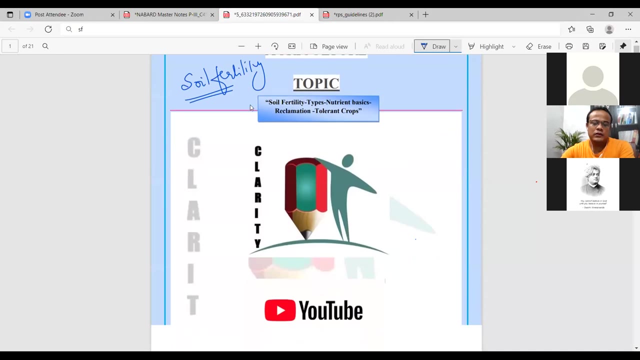 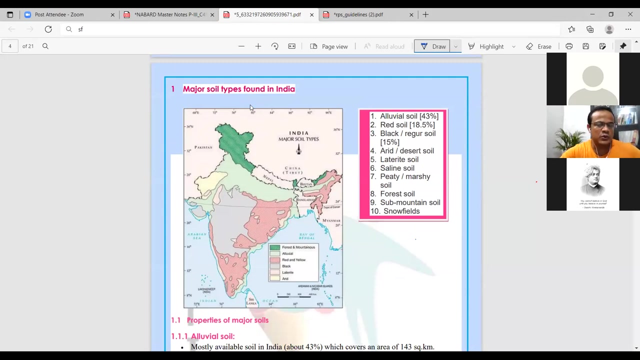 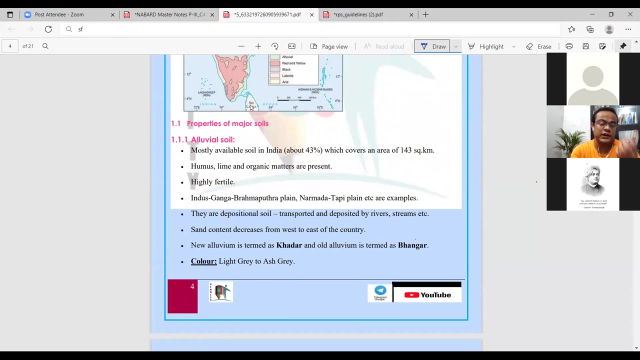 okay, fine, so we'll go with the soil fertility part of the talk we discussed here, that is, soil science or some of the organic agriculture related. now i will discuss the soil fertility. now i will discuss today also. lastly, Alluvial soil is the newest and most fertile soil in India. 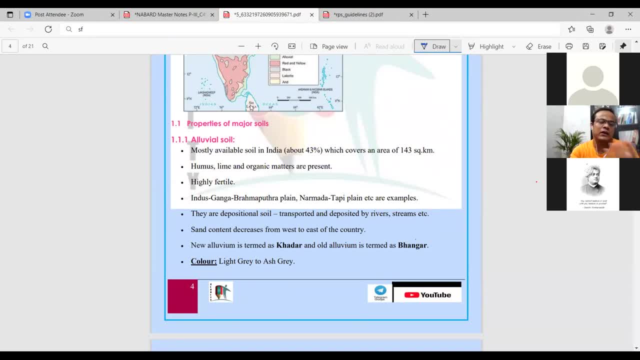 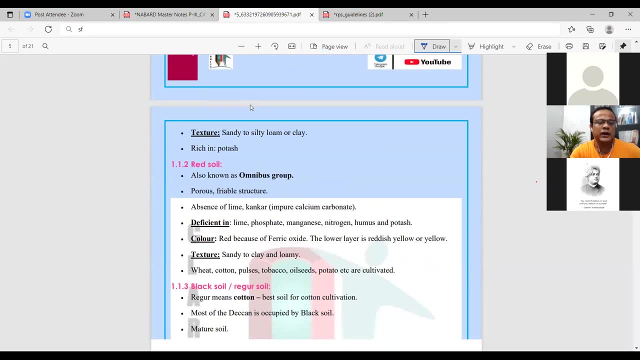 Its local names are Khadar and Bangarh. It is found in Ganga, Brahmaputra Valley region. Alluvial soil is found where rivers are present. I gave notes last year and a question came from the same note: Self-flowing soil. This question was asked last year. 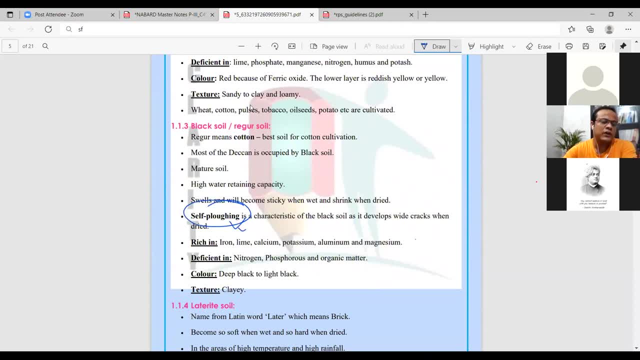 It was directly from this note. Self-flowing soil, which of the following is called self-flowing soil? That is, black soil. Black soil swells and sinks due to its clay content, So we call it self-flowing soil. This is important. 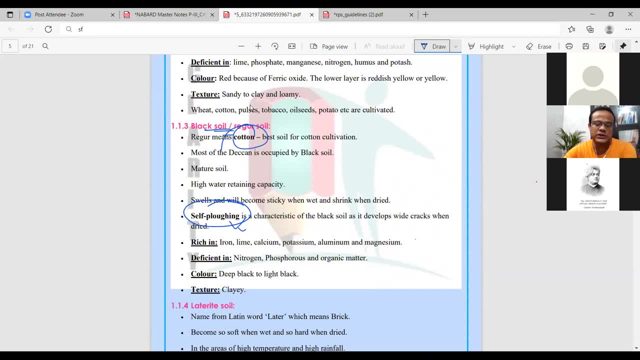 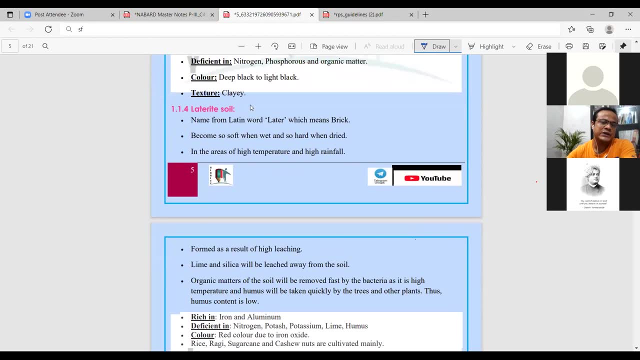 This is very helpful for cotton growth. You should remember this. You have to read these facts here: Which soil has more nutrients and which soil has less Laterite soil Laterite comes with the word brick, You have to remember. They can ask you questions. 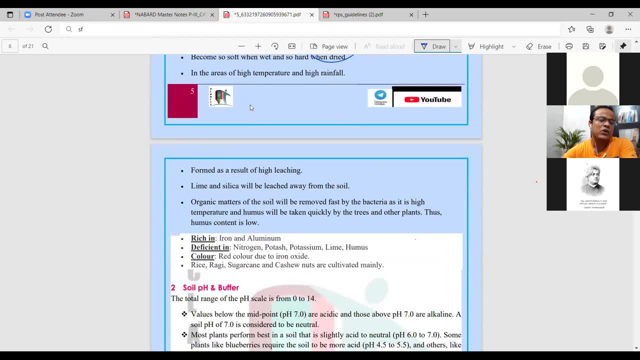 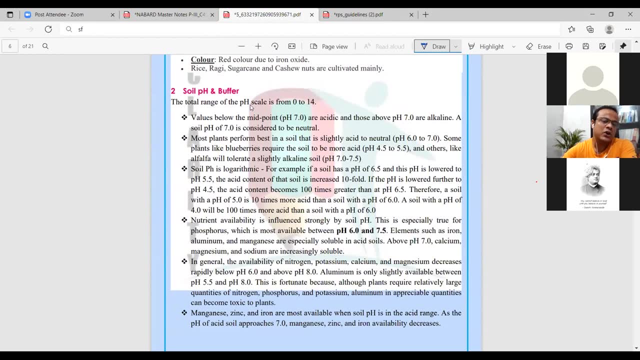 Which of the following soil is related to bricks? It is laterite soil, Which soil is deficient and which is rich? You have to see that When we talk about soil pH and buffer, the most important point to remember here is pH 6 to 6.5. It is the best pH where nutrients are most supplied to plants. If the pH of soil is 6 to 7.5, then this is called as the best pH of the soil for producing or providing the nutrients to the plant. In this range, the nutrients can be easily absorbed by the plant. 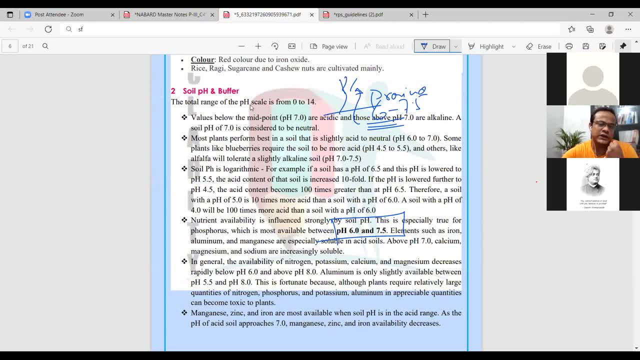 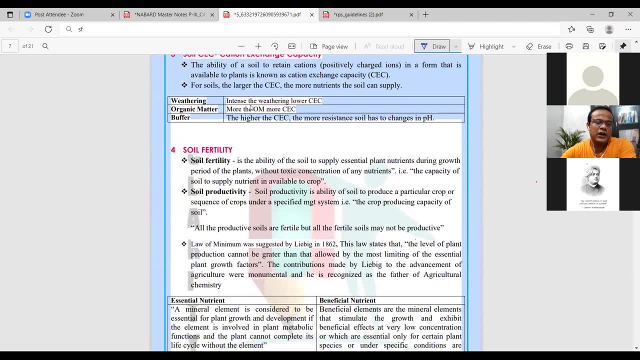 If it is more or less than this, then the absorbing capacity of the plant decreases. You have to remember this. This range- they can ask in the examination Two terms in soil fertility. Remember these. two clearly Definition-based questions can come from here. 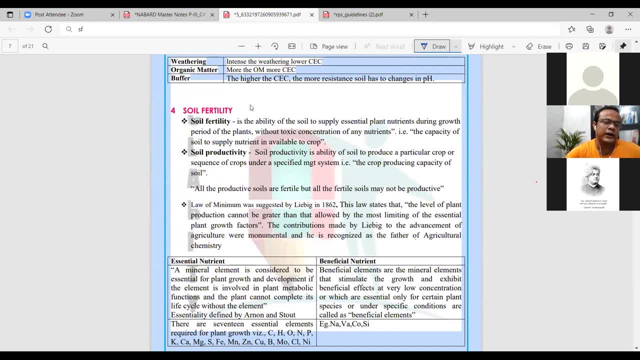 When we talk about fertility, we talk about the capacity of soil to supply nutrients and productivity- The crop producing capacity of soil. Be clear in both. There should be no confusion And you can mark the right answer. Make it clear And look at this definition. 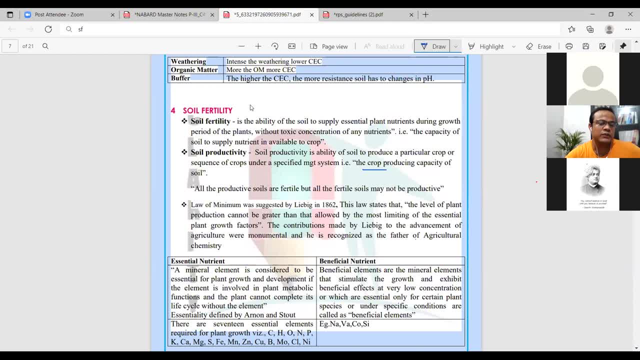 It is self-understanding. In the last class I explained that all the productive soils are fertile, but all fertile soils are not productive. What is the reason behind that? You can understand it yourself. The concept of pH is related to that. 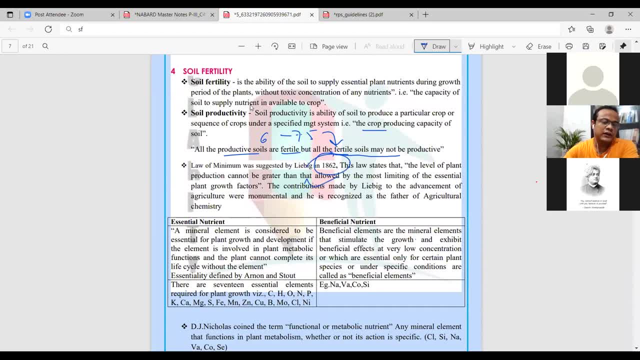 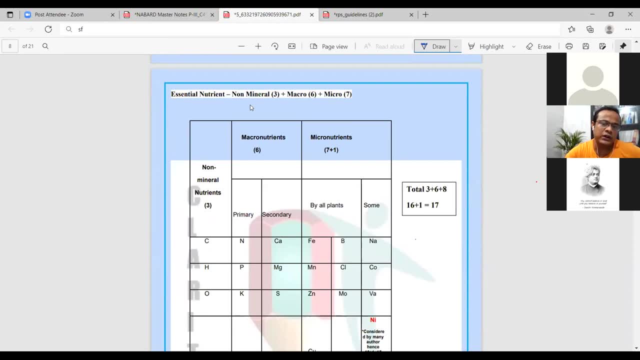 Who gave the law of minimum and in which year. You have to remember this. Now. look from here, Questions come from here. When we divide the essential nutrients, it can be divided into three parts: Non-mineral, Macro And micro. 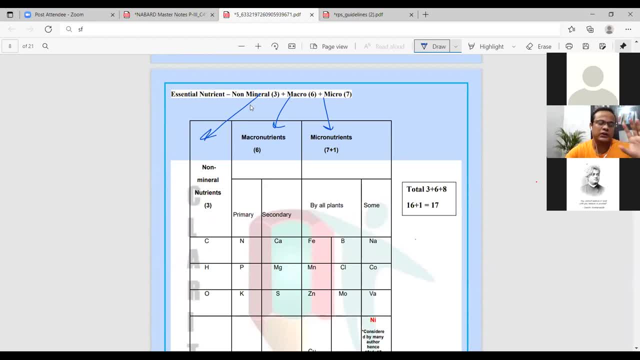 Questions come from here. You get one or two questions every year from here. Which of the following is not a non-mineral? Which of the following is a macronutrient? Which of the following is a micronutrient? What are the numbers of which? 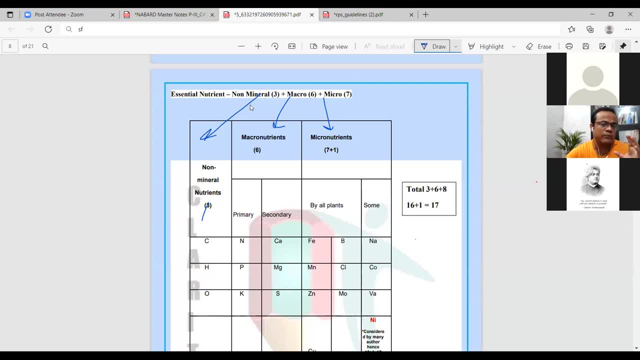 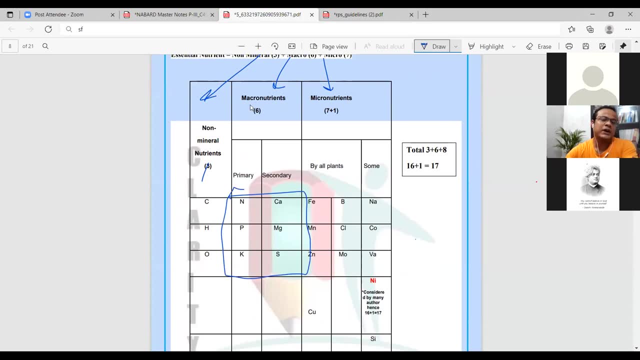 You have to remember this. There are three non-minerals: C, H, O. In macro, there are six: N, P, K, C, A, M, G, S. Remember it well. Here comes the question, by mixing up. 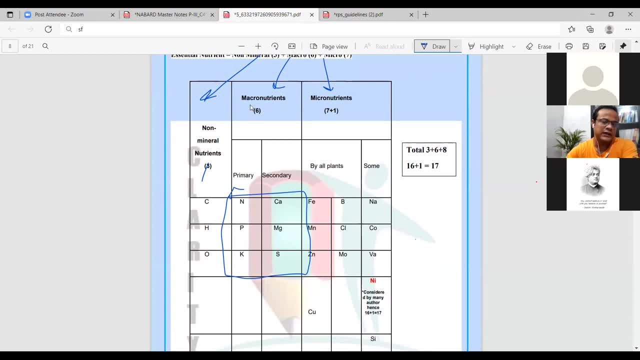 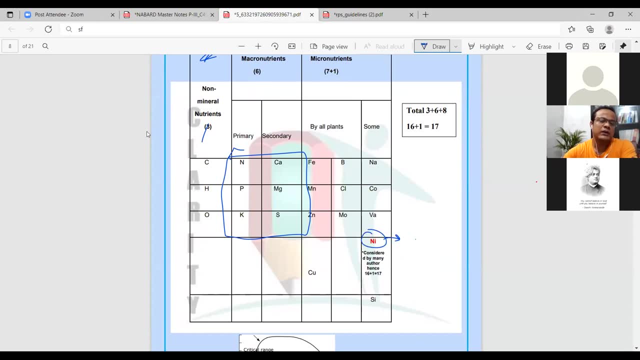 Which of the following is not a macronutrient. One micro will be added from there, Seven plus one in micro, Because one position, that is, that position, is considered by the author and none by the author. So seven plus one was written. 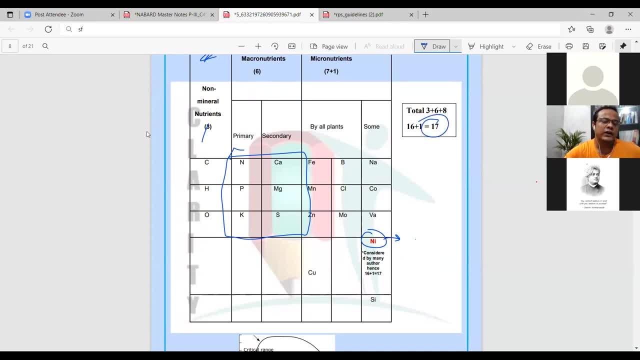 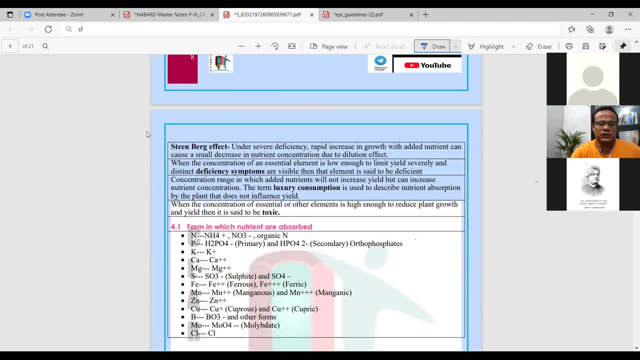 So overall, you have seventeen essential nutrients. You have to remember Sixteen and seventeen. If you take nickel, you will take seventeen. If you don't take nickel, you will take sixteen. Next, again, a question comes from here. They have asked many times question from here. 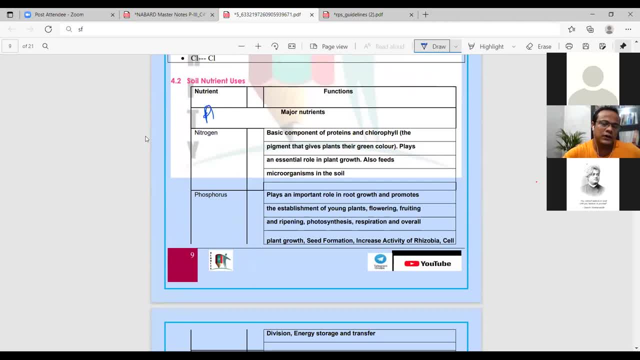 And you have to go to this chart in red. well, Mug up this chart, Go from here. you have to select keywords and you have to remember keywords. last year also, we have discussed and directly question came from here- which of the following nutrient helps in feeding the microorganism in soil? 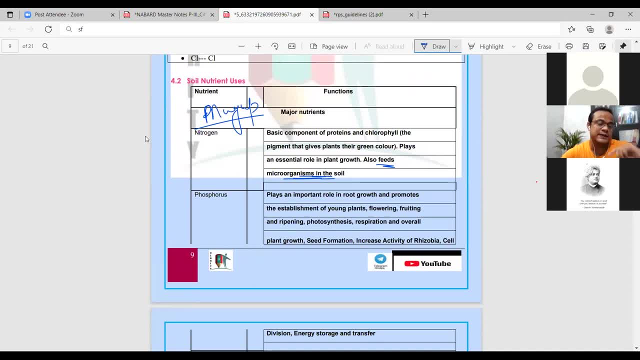 so this was the question. next is self-flowing question. so from here, you can remember as many keywords as you can and try to relate. if it is related to phosphorus, then what is it promoting? so remember all these points from here and remember keywords one by one. 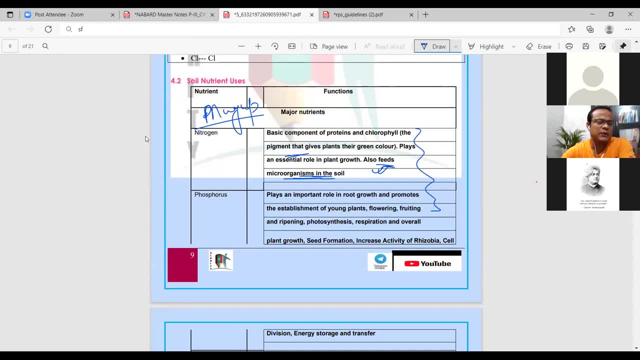 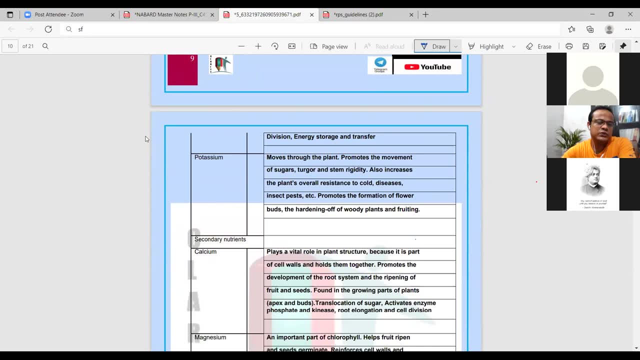 if not, then I have taken a lot of classes related to this last year. it is still available on YouTube. you can search and see those classes. if we talk about potassium, then it promotes the mucus. the movement of the sugar is this. and one more thing comes here you have to keep in mind. 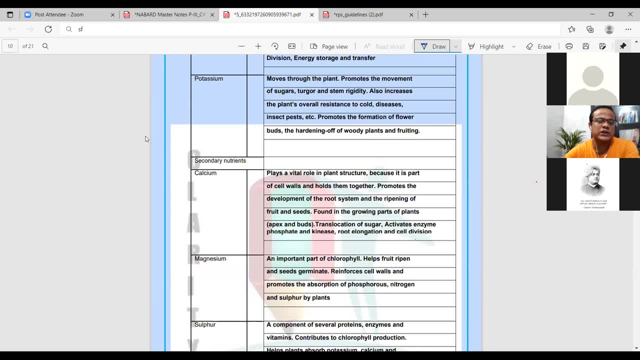 here it is given translocation of sugar, see movement of sugar and translocation of sugar are two different things. when we talk about translocation, then if you get the first option- boron- so you go for the boron, because this is very important question. it has come many times in many examinations. 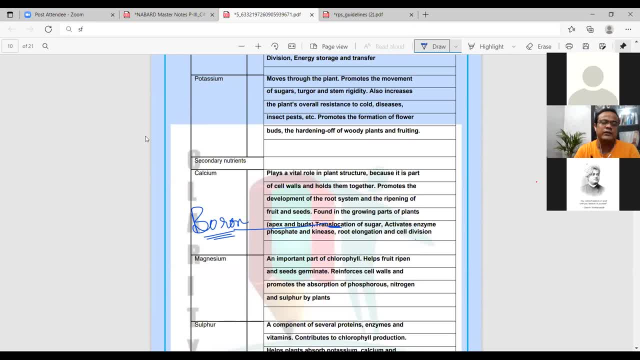 translocation of sugar. what is the keyword? it is translocation. so translocation is related to sugar whenever you get the first option. so if you get boron, then you go for boron. if you don't have boron, then you can go for the calcium. 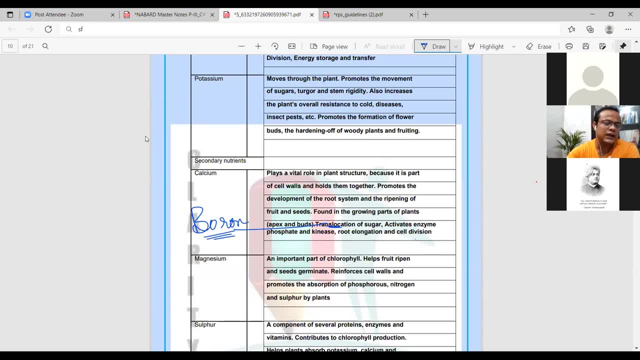 so if you get boron, then you have to remember well, if you don't have to go with boron, then you have to go with calcium. how do you remember keywords? then, what is cell wall? what is cell wall? it is a basic structure. 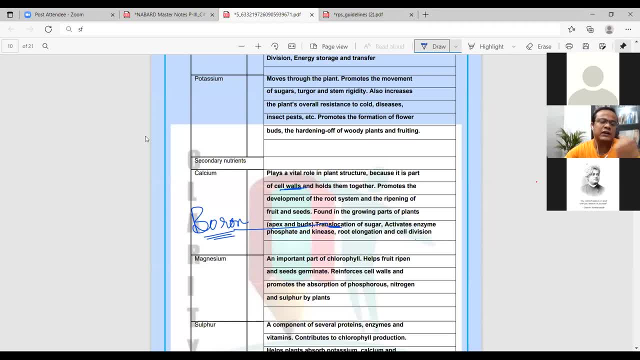 what is the basic structure of our body? it is a bone, so cell wall is the basic structure of the plant. so that is being formed by the calcium. so what is the keyword here? it is cell wall. if it is a question related to cell wall, then the answer will be calcium. 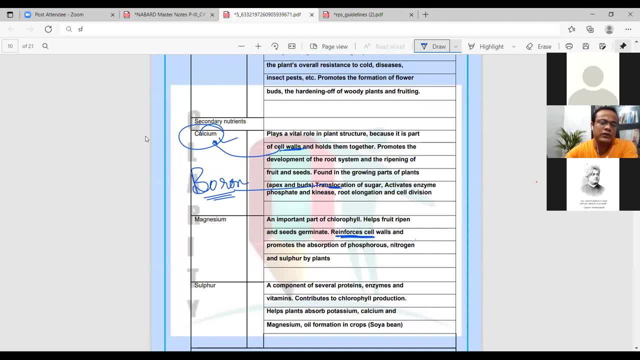 it is related to magnesium. it reinforces the cell wall. it is a part of cell wall and holds them together. but if the keyword reinforces the cell wall, then the answer will be magnesium. if you can write this chart, then write it. it is possible that this question will come again from this year's chart. 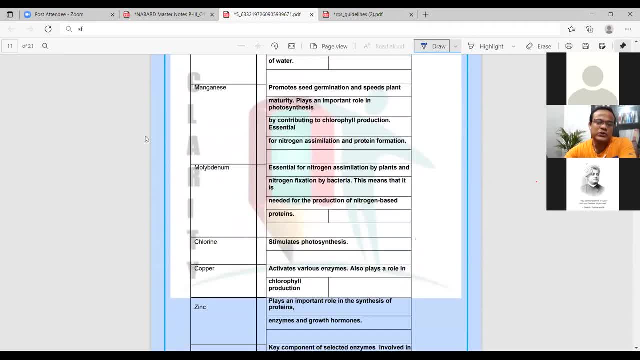 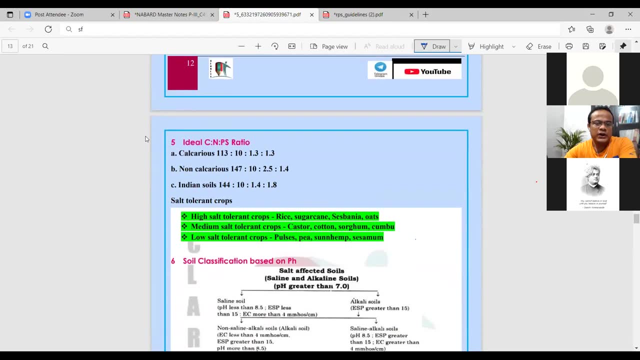 so all these are important. you go through them one by one. there is no need to explain it. the more you remember, the more it will be helpful for you in the examination. not so important now. this part is very important. remember these ratios. in grade B I think they have asked one of the ratios. 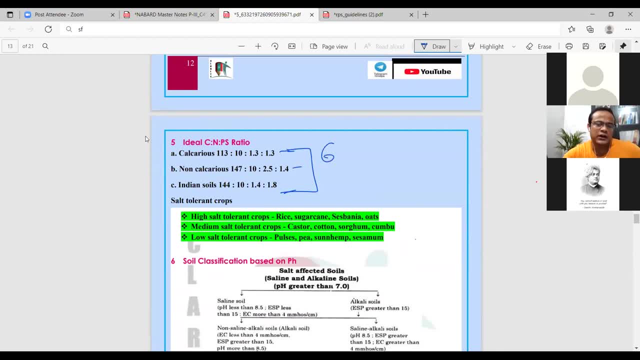 from here to here, from somewhere. a question was asked in grade B. I don't remember exactly. remember these ratios, especially what is the CNPS ratio in Indian soil. you have to remember this: 144, 10 is to 1.4 is to 1.8. 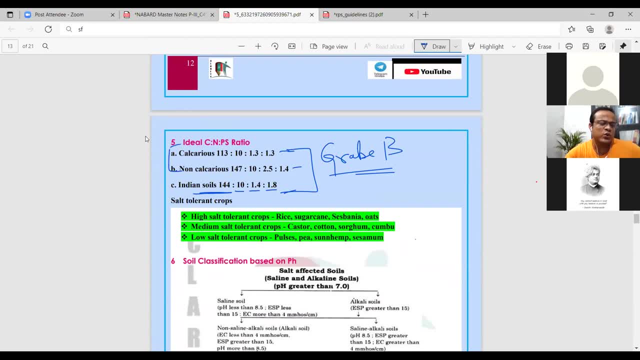 these and you can remember these two together. remember any one or two data so that you can mark it by looking at the options. that's it. it is very important. if we talk about NPK ratio, then what is the general NPK ratio for Indian soil? this CNPS ratio is given. 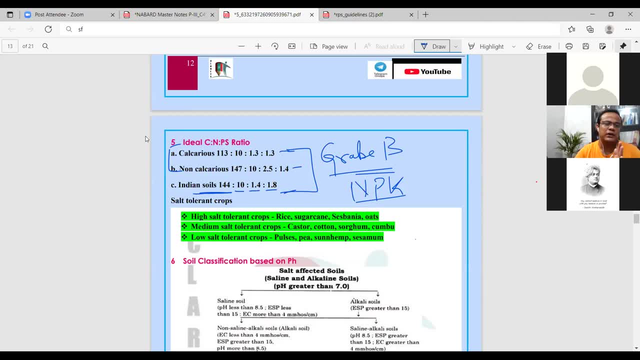 if we talk about NPK ratio, then what is the ratio of NPK in general? what is the value today? I gave you the PDF. this is also given in the fertilizer association of India recommendation. it is very good. I think you have gone through that notes. it is 4 is to 2 is to 1. 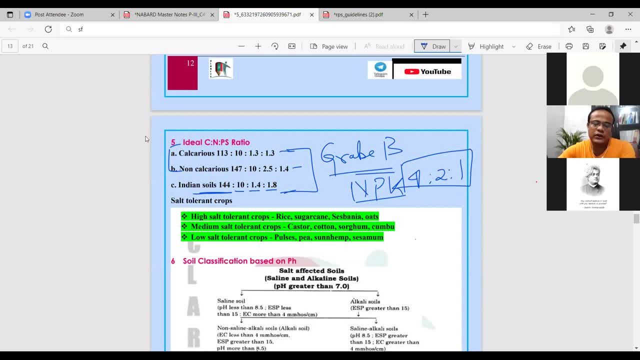 very important. you have to remember this ratio. this is what happens in Indian soil. no, there is something else. this is the ideal ratio. this is the ideal ratio of NPK. there is something else in Indian soil. you can go and see it. what is the ratio they have given for the Indian soil? 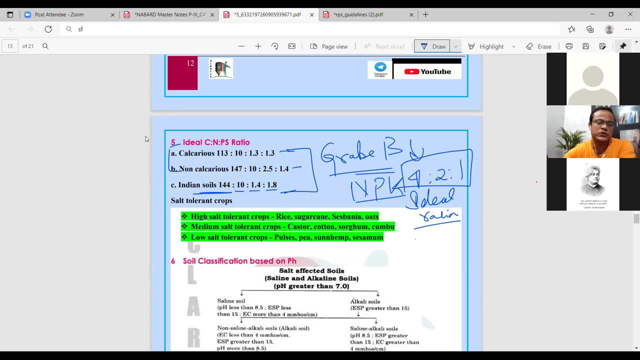 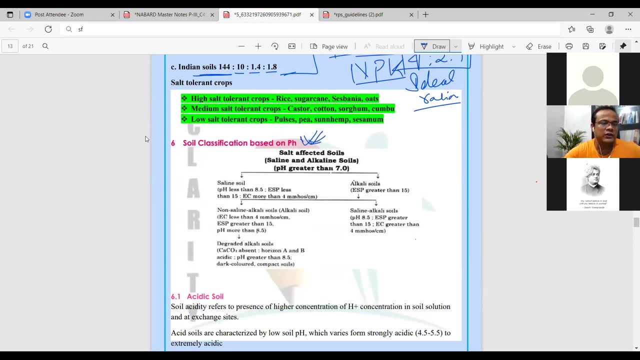 and this is the ideal. what needs to be achieved? 4 is to 2 is to 1. next we come to soil. this classification is very important. we know a little about this classification. yes, Samriti, very good. the Indian condition is 8.2 is to 3.2 is to 1. 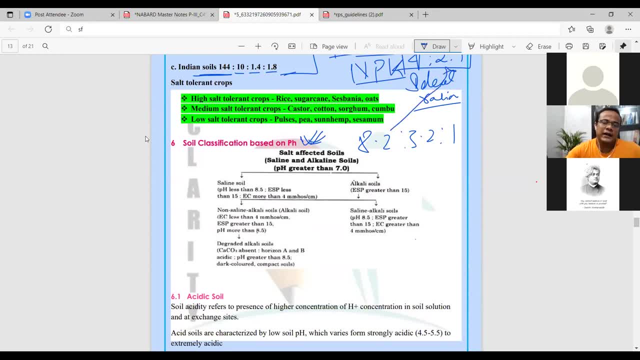 this is the condition we have to reach. 4 is to 2 is to 1. we also get questions from this classification. you can see this classification. don't skip this. how do we classify soil? look, there are two types of soil: acidic- we see basic acidic. 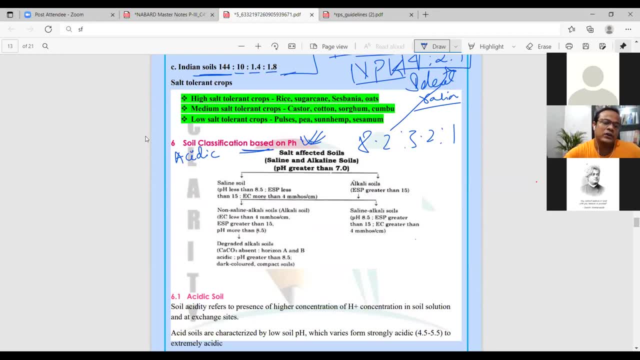 and other is saline, which is salt affected soil. ok, so acidic is that soil where pH will be less than 7. where pH will be greater than 7, we will call it salt affected soil. so again, when we take salt affected soil, pH greater than 7. then, according to ESP, we divide it into two parts: less than 15. more than 15. if ESP is greater than 15, then we call it saline soil. if it is less than 15, we call it saline soil. then when ESP is greater than 15. 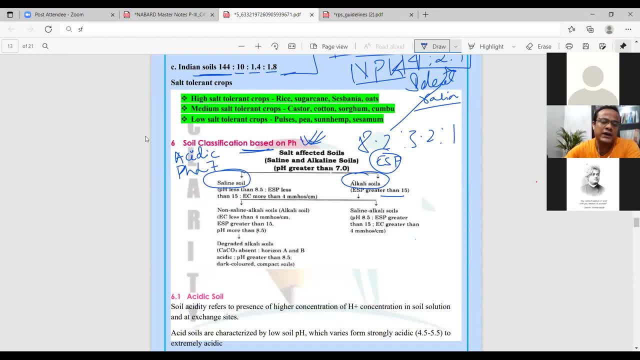 then again, division happens on the basis of pH, on the basis of electrical conductivity. so you must see these classifications. this is very important. this comes in your examination. you can make a clear chart: write EC, write pH, write ESP, write their values here and here, write type of soil. 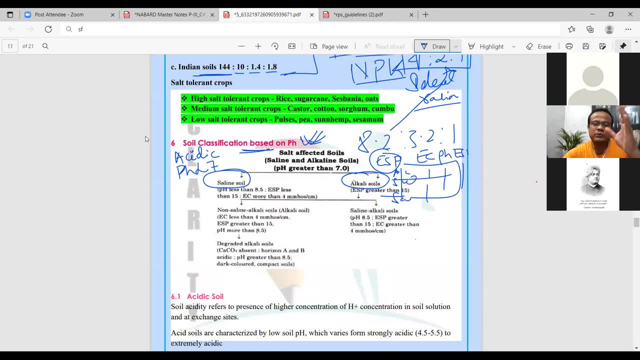 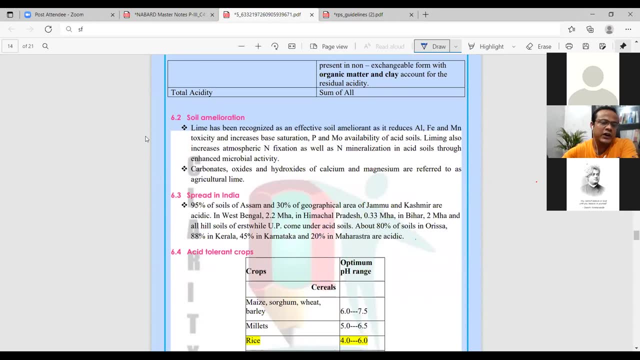 acidic soil, saline soil, alkaline soil, you will remember this from one chart. ok, see this. this is an important part, ok, next, coming on to this soil amelioration, how you can correct the acidic soil. which soil is good, which is bad? so, maximum cases, gypsum is used. 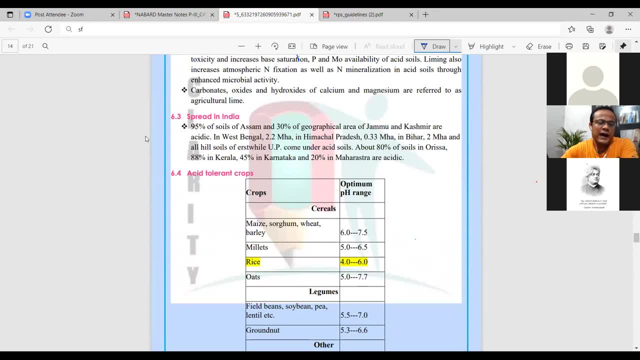 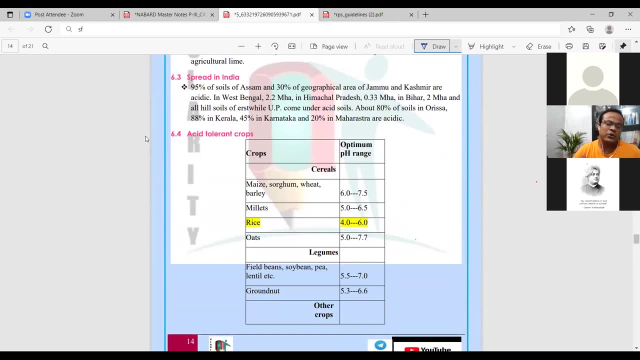 remember. ok, see the soil amelioration. what are the acid tolerant crops? see in this? you will get a green color box. you will get a little ambiguity, but when we grow crops there are many conditions for the growth. so these are the exact values which have been taken out. 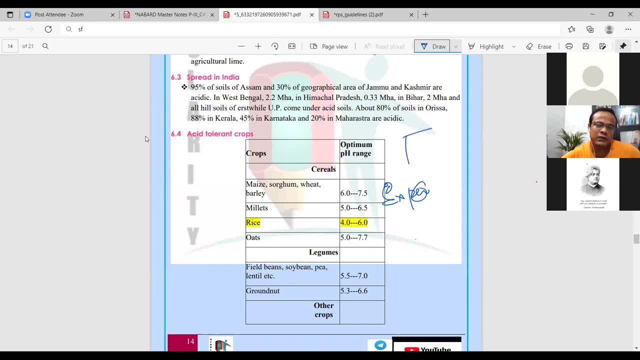 from different experiments. do not compare this with the green color box. there is a little ambiguity in the data, but since these are given in the books, it is taken from the books. so remember in both the forms, because when you grow the crop, so this experimental data does not work there. 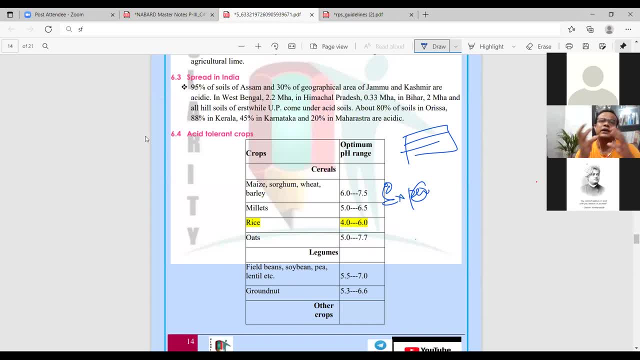 many more things are there which affects the growth of the plant, so they are affected by that too. so here you have to see the maximum and minimum values. whose maximum is whose minimum value is? you can see from here, and one more column you will get later on. 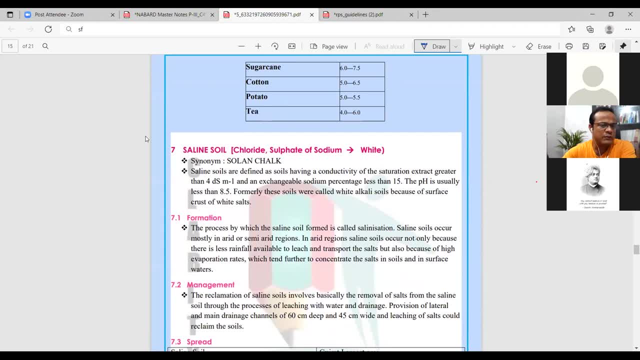 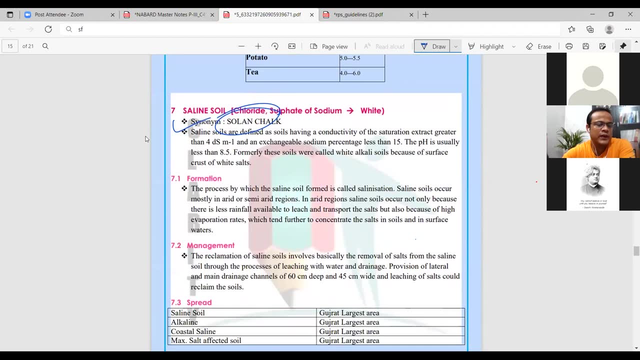 that is green box. different types of you will get there. that is also important. saline soil is called solen chalk. it is chloride of sulfate and sodium. see this type of soil which is saline or alkaline. you have to read this by relating from where you have to read by relating. 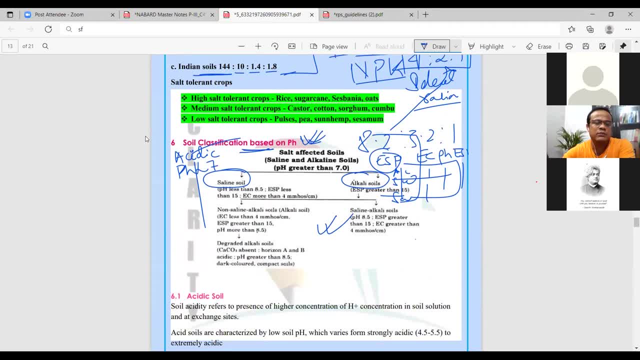 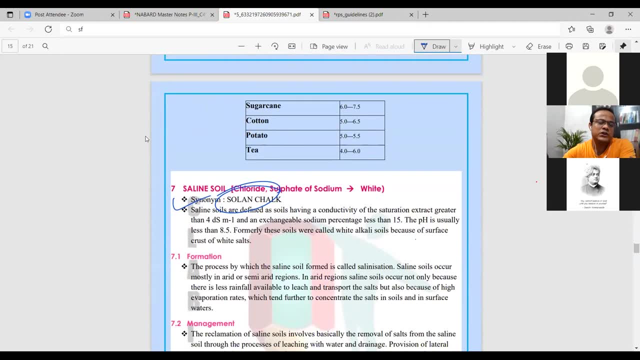 from this box that we discussed. you have to read by relating from this box, you will understand everything very well. ok, there will be no confusion. so, different types of soil. what are their alternative names- you have to ask questions from here- and what is the basic form? you have to remember these three things. 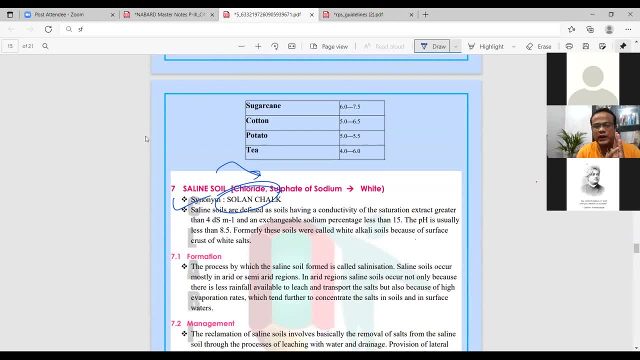 their ranges. what is the range of pH? remember that, remember their synonyms and what with. they are made up of basic components. you have to remember from here: saline soil, because there are chlorides of sulfate and sodium, so the color will be white only. ok, you have to remember this only. 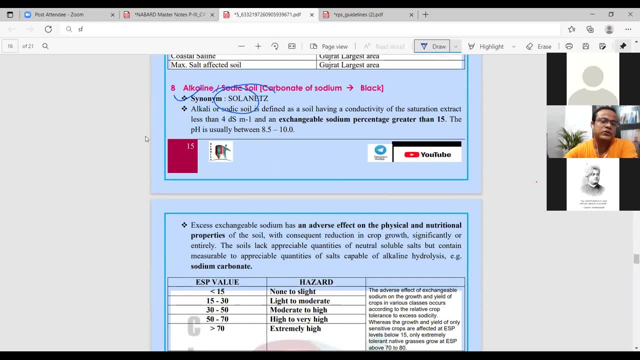 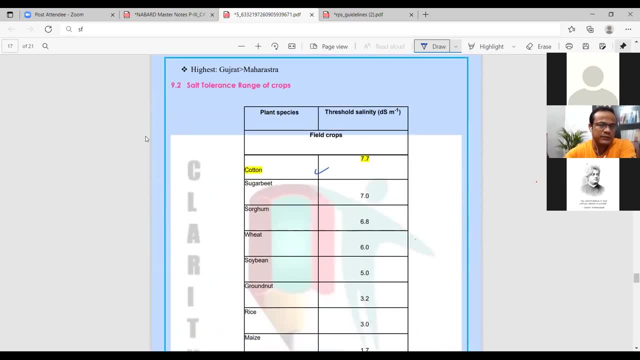 alkaline or sodic soil is called solanates. these are carbonates of sodium. these are black colored. ok, now coming on to next part. next part: salt tolerant cloth. you have to see its ranges. we have seen acidity ranges. these are salt tolerant ranges. you have to cover maximum and minimum value. 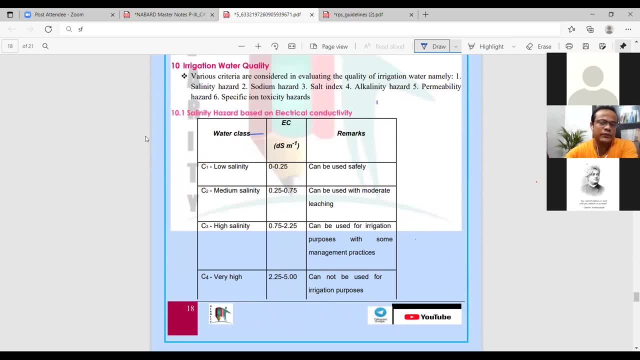 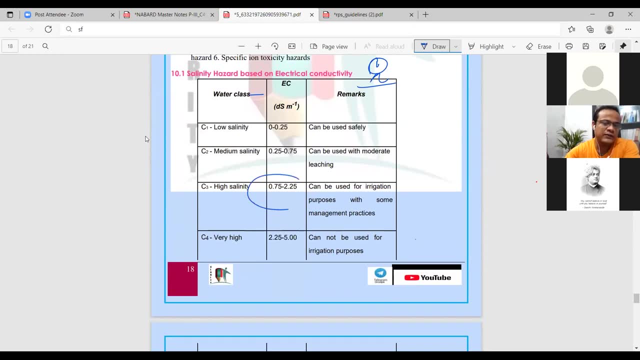 irrigation water quality. again question has been asked. again they have asked question from here, so now you have to see irrigation water quality. they will give this value. if it is 0.75 to 0.25 EC, then what type of water class it is? salinity range. 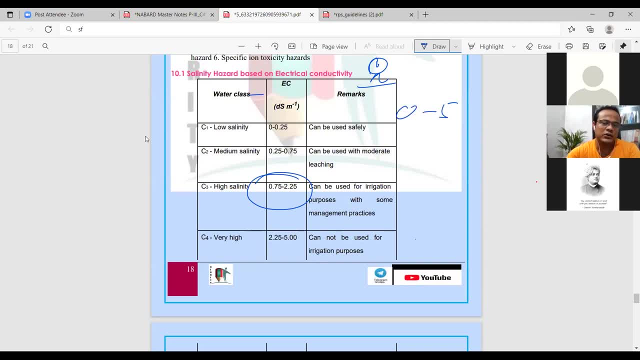 so you have to remember these ranges from 0 to 5 values. from 0 to 5 values. so if you have a little idea then you can mark by looking at the options. you don't have to remember the exact data by looking at the options. 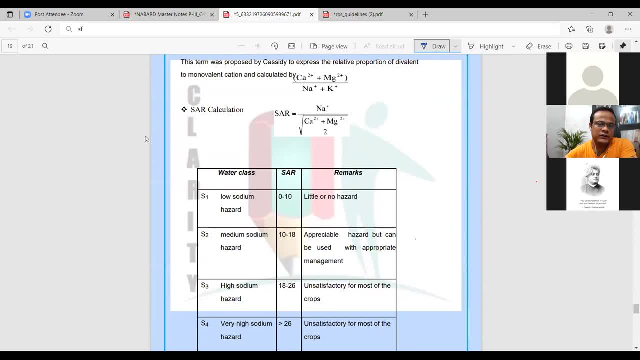 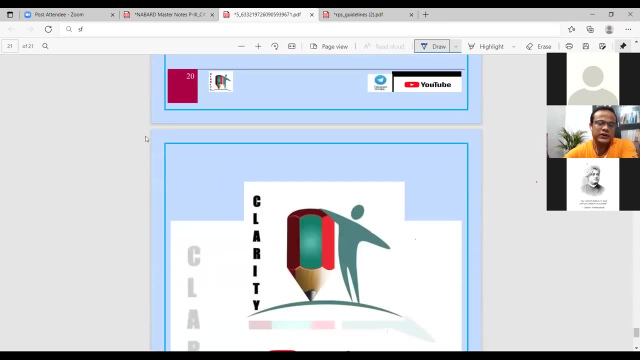 you can easily mark for this. ok, its formula. land development people. this formula. they have asked in the examination what is the formula of SAR? some land development people is there. they have asked this formula of SAR: first, residual chlorine. ok, these are the ranges. you have to see this in this. 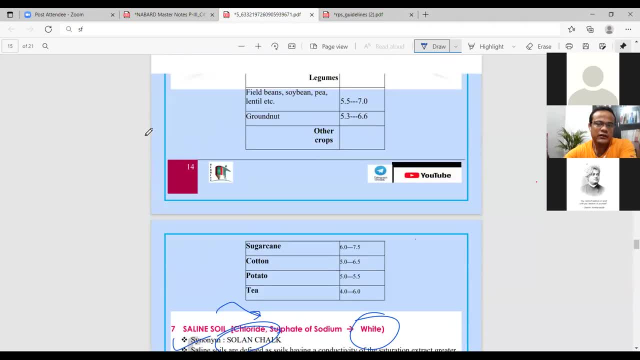 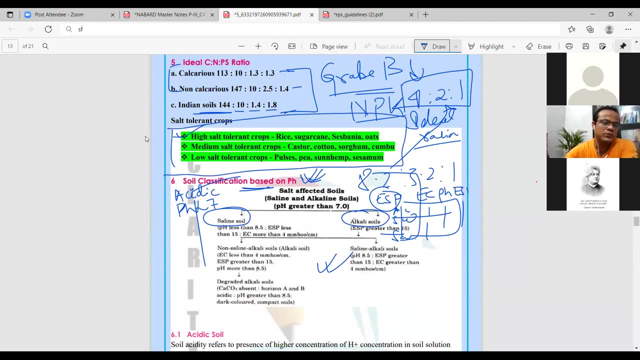 and one green box that I was missing. ok, from here. question. yeah, this box. see, the question has come from here. you have to remember this box well, that which are the high salt tolerant crops, which are the medium salt tolerant crops and which are the low salt tolerant crops. 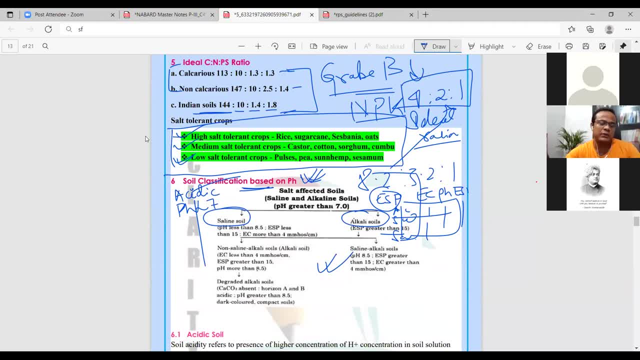 you have to remember these. ok, you will get ambiguity from those data, but I have told you the reason why you will get ambiguity. but the form in which it is given you remember in that form for examination that will serve the purpose here. don't use scientific mind. 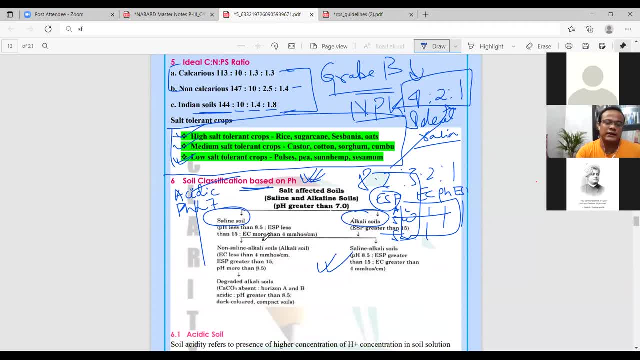 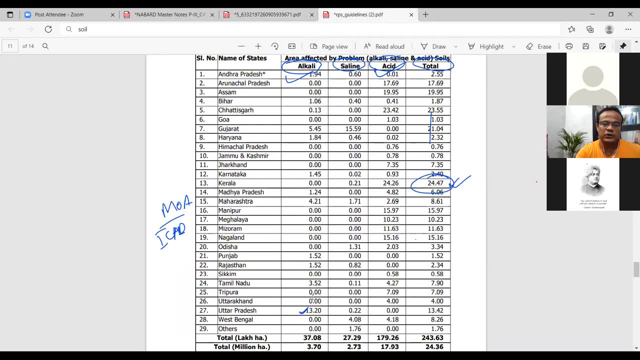 you will get confused. that's why I am not saying: now the area thing comes. some questions have been asked from the area area that will tell you area portion also. I am sharing with you the new screen for you. new screen is visible to everyone, yes or no? 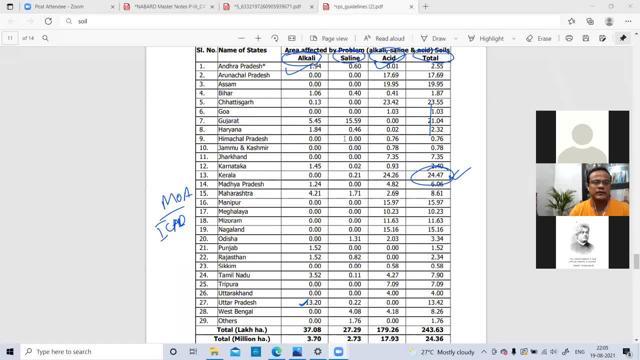 this is very important from here. also question generally: they ask yes, so see the data in pdf. it is little bit old in that don't see that. in which state is the most alkaline soil? in which state is the most acidic soil? in which state is the most total affected soil? 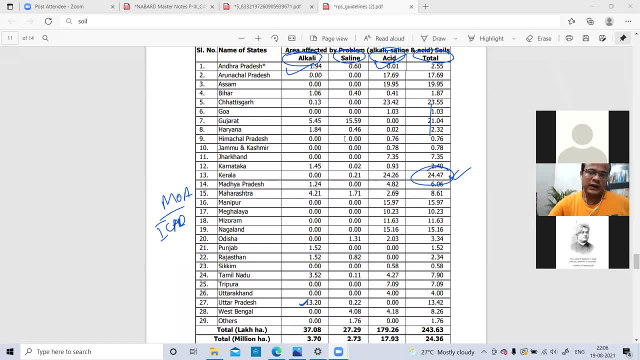 you don't look into this data through that pdf. see from here. this is the latest data as per ICR I have taken. ok, when alkaline soil, remove it now. see from here. one question will come this year, also 100%. one question will come: will come in prelims or mains. 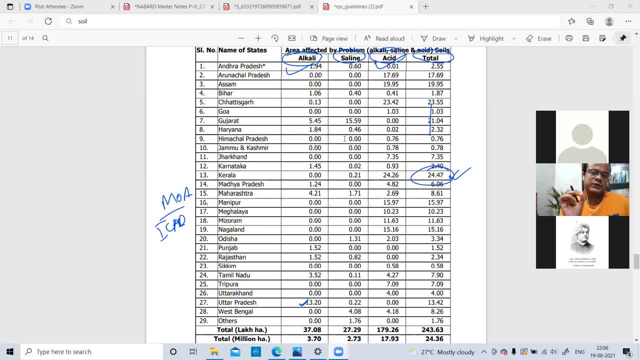 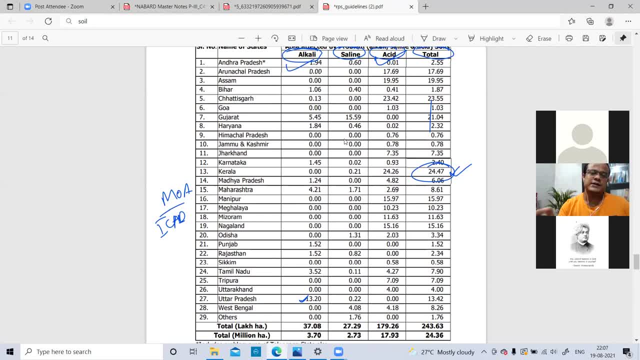 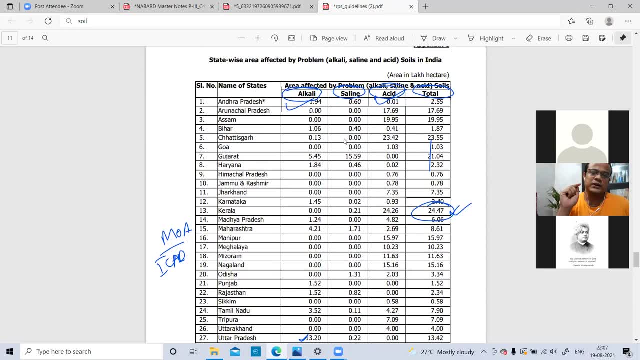 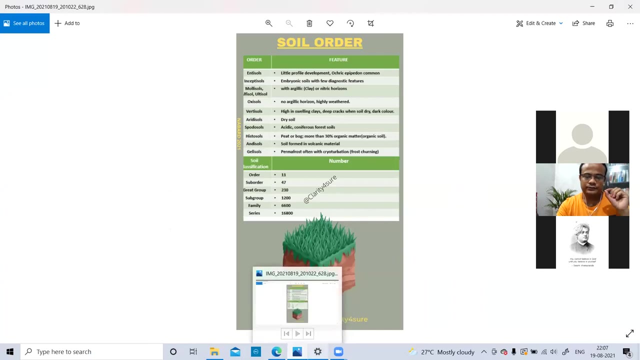 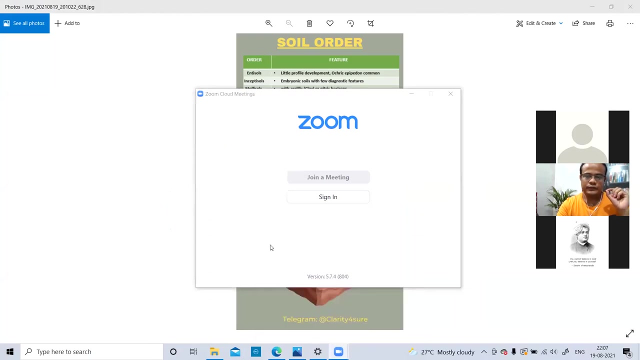 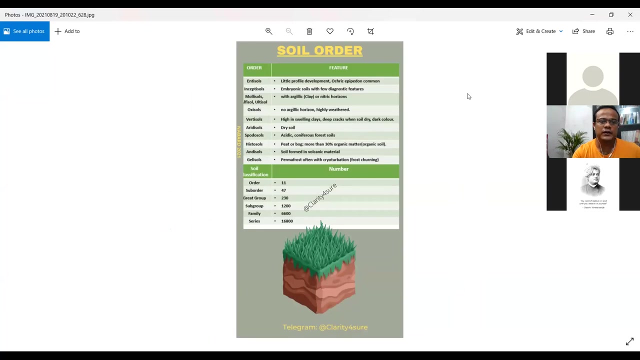 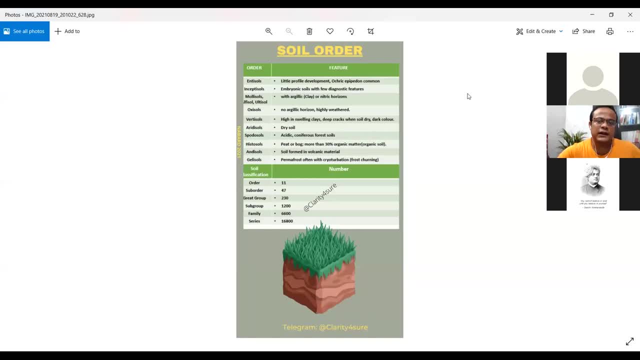 figure, yes in this. look at how many orders any of these are. at least remember it is 11 order, are there? if you remember, you don't have to remember anything. we have 11 orders, all the orders 47, remember this much. leave the lower one not important. 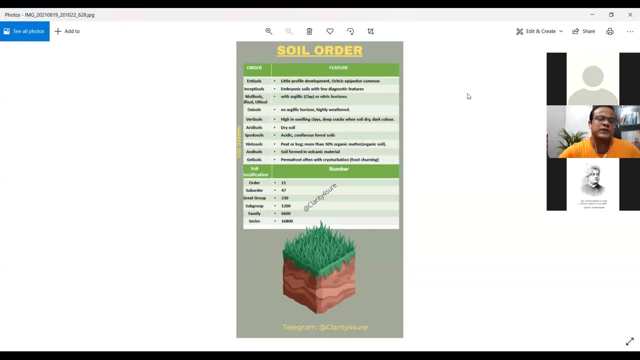 This is Entisols. Here you can see some specific features. This is Entisols. It is called Ochric Epipedon means it does not have stratification soil, The layers O, A, B in the soil. 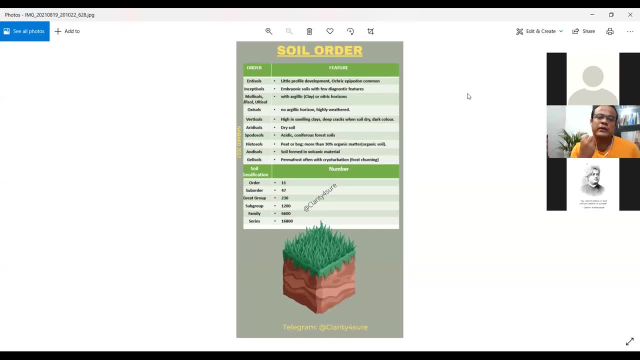 you will not find those layers in the soil, Because this soil is very new. If it is new, then I would like to ask you- it is a basic question- which type of soil it will represent. Entisol order will represent which type of soil. 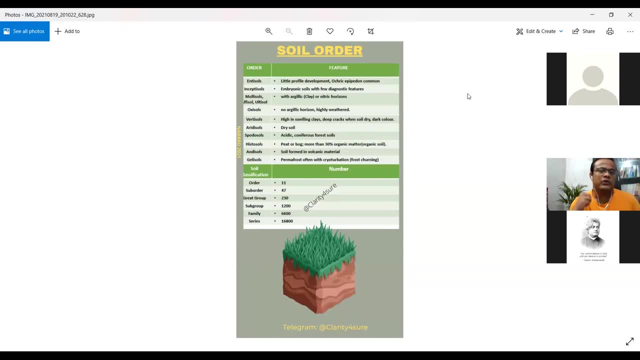 Alluvial black laterite: Very good, alluvial. Now I have explained that Entisols are newer soils. Newer soils are also alluvial, So alluvial soil represents your Entisol order, Very important. you have to remember this. 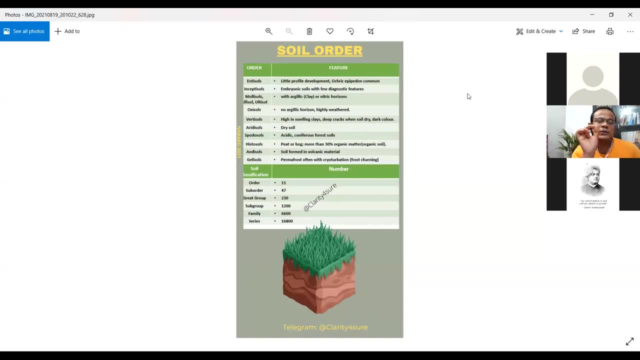 Remember this unique word, Ochric Epipedon, Always relate it with Entisol. Ok, If the stratification of Enceptisol is a little more, then Entisol comes after Enceptisol. Ok, Molysol, which is the third column. 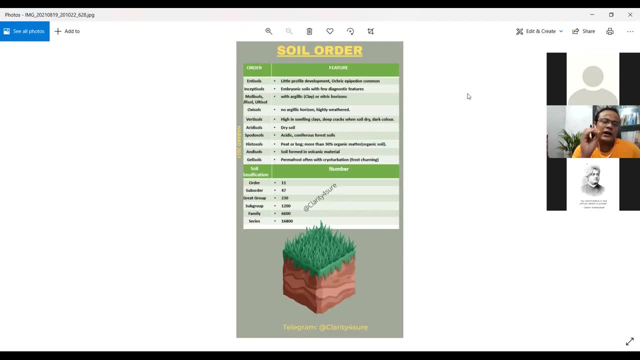 Molysol, Altisol and Alfisol. it is called Argylic- Argylic soils. Why? Because these three have clay formations. So if you are asked which of the following is not Argylic, then you have to remember the names of these three. 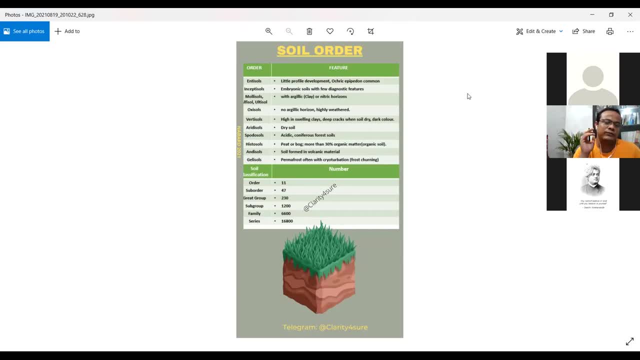 Ok, Molysol, Altisol and Alfisol. Ok, One more question is there? Ok, Which of the following is most weathered? order of soil: Which of the following is most weathered, If we talk about weathering the most? 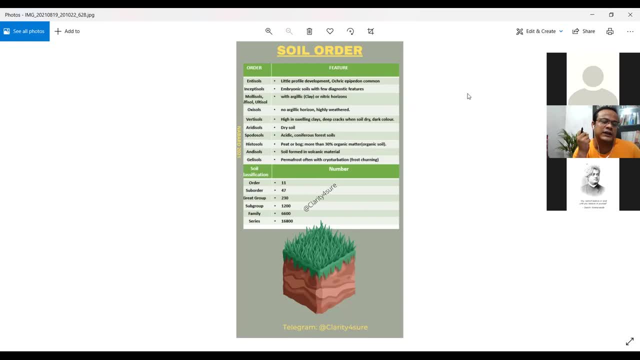 then oxyzole has the most weathering. Ok, Most weathered soil is oxyzole. If we talk about black soil, which order represents the black soil, So its vertizole order represents black soil, And if we talk about red soil, 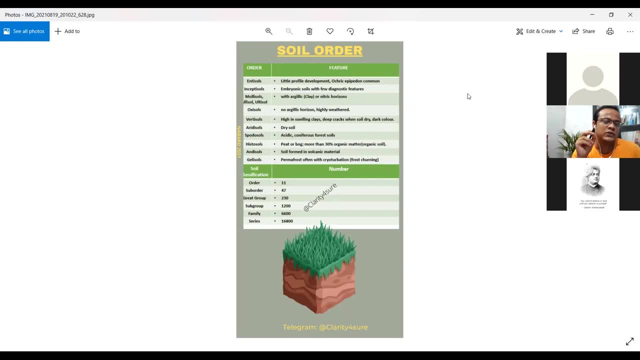 then that third number block, that is, Molysol, Alfisol and Altisol, represents your red color soil. You have to remember this. Rest of the things are easy. Histozoles are the marshy areas where the water is accumulated. In that area you will get histozoles. 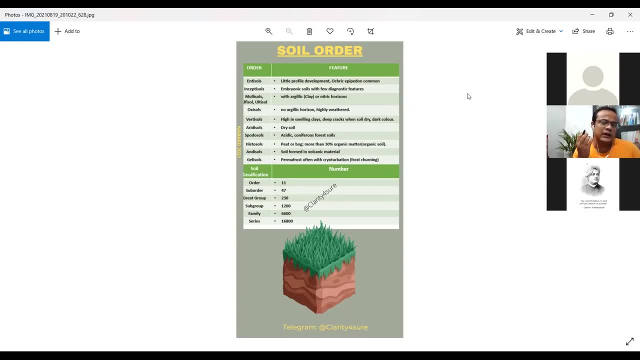 Andisole is the name. Ok, You will get it in volcanic areas. Gliazole, permafrost- you get it in very cool regions. Aridizole is the name. Arid means you get it in dry regions. 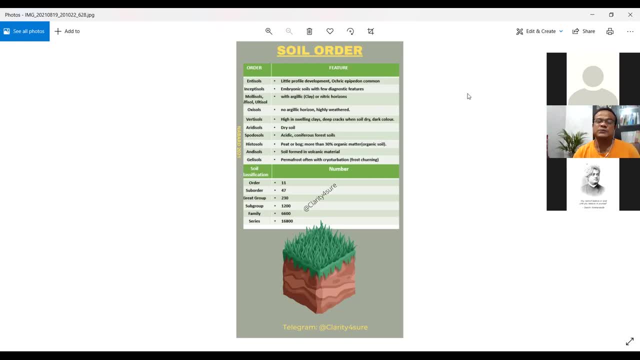 So this was the overall structure that you have to cover in soil science, soil fertility. I think I have tried to cover all the things Within, I think, more than an hour. So these were all the points That you have to cover. 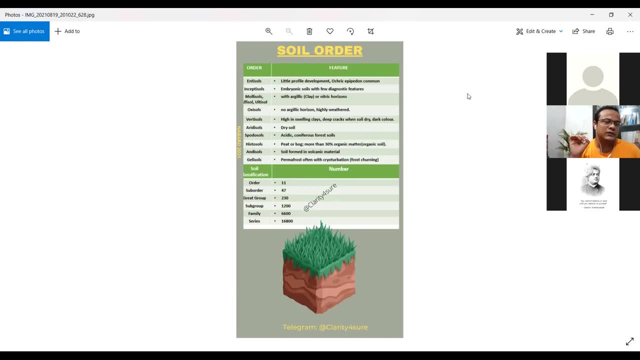 From where, basically, questions are asked in the examination. Ok, So I think this will suffice And overall, I have given the view. Is it ok for everyone? Is it ok for everyone? Ok, So I think you should not have any problem in the soil science chapter. 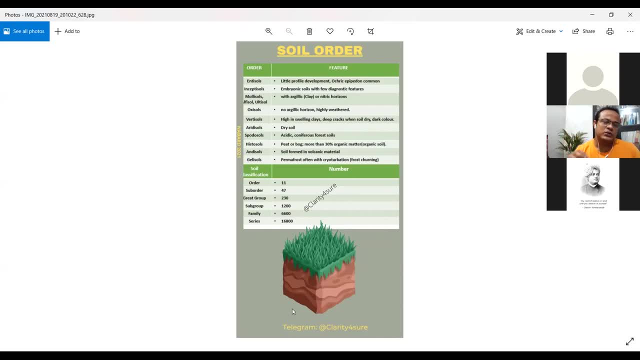 Now you can cover it easily And, after covering it, give a test. Whatever you have missed, you will get to know in the test that this is missed. Even I missed it in the session. You don't remember everything right, So from there you note it down. 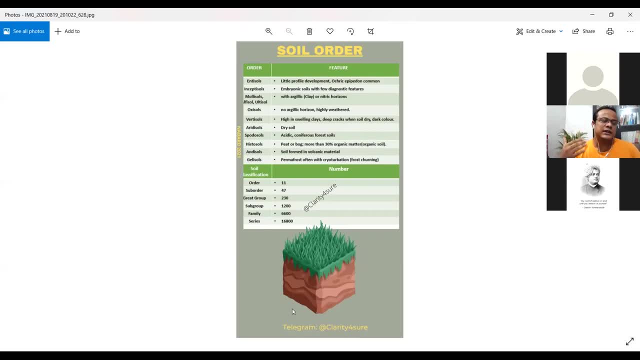 and remember it a little. Now see why the competition is less. Please stay on. I would like to tell you one more thing. See, so many students sit to watch the competition. So many students sit to watch. There is no competition. 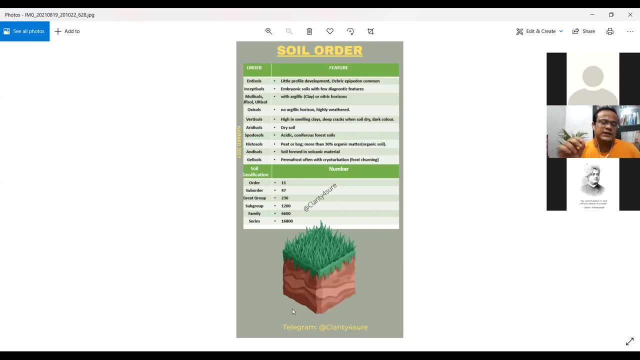 There is competition only in these children in the examination. Now see in the sessions. when we started the session it was around 100 persons we were watching, But they did not have so much patience that they can complete this overall important topic. 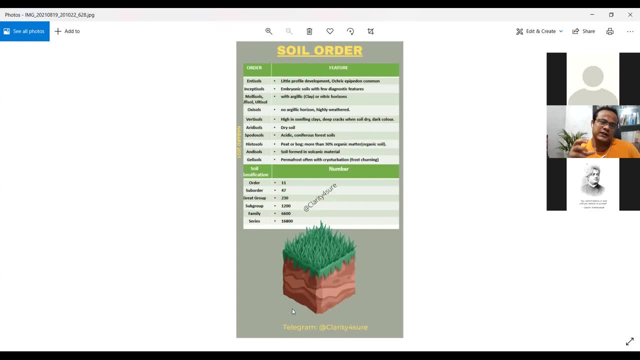 They left it out. Around 60 persons are there in this session, So this is what happens: The one who is preparing. I say this because if you are consistent, children, if you remain consistent, you will get the benefit till the end and you will succeed. 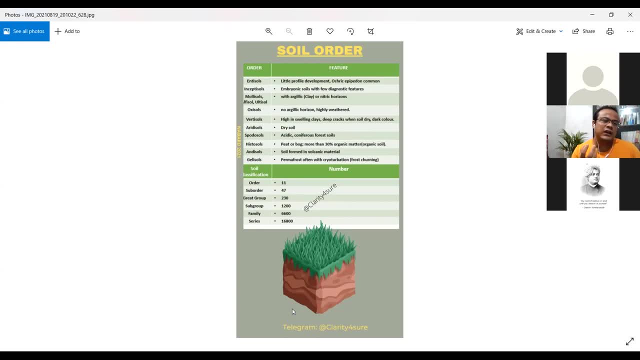 in the examination, Those who lose patience and they do not want to cover the things. then you cannot do the examination. You cannot crack at all. Ok, So keep some patience and try to be consistent. You people definitely will qualify. It is just a game of patience. 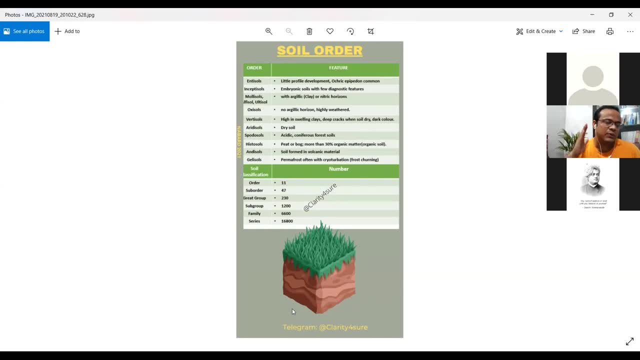 and consistency And never be negative. Never have a negative attitude. Always be positive, Keep doing it. Whenever you feel something negative, you talk to me. I will try to motivate you people. Ok, So let's go. We will meet tomorrow. 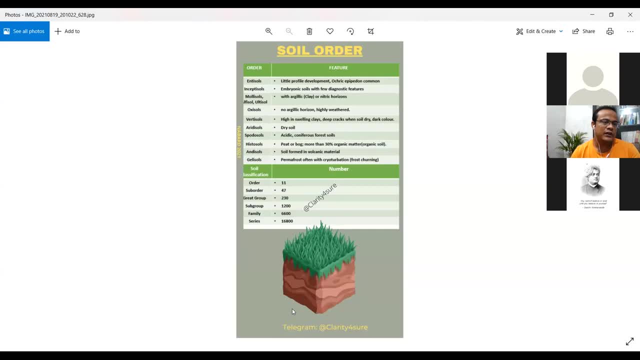 again with new topic. Ok, PDF is, I think, not editable. I think so. it is not editable. I have not tried it, but it is not editable. Ok, Let's go. I will end the session. Ok, Good night everyone.